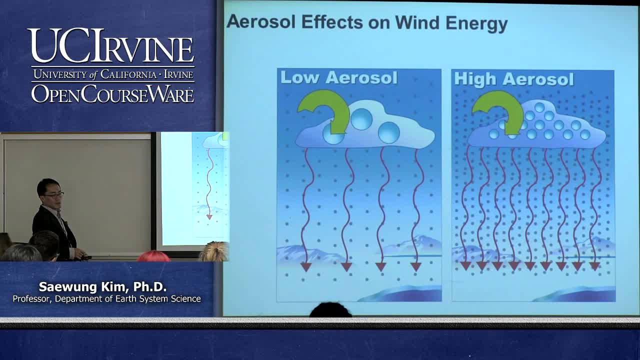 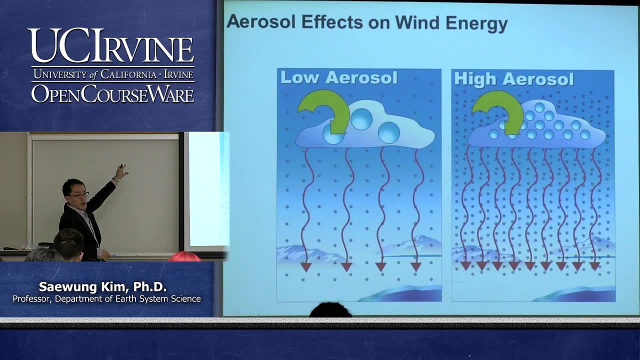 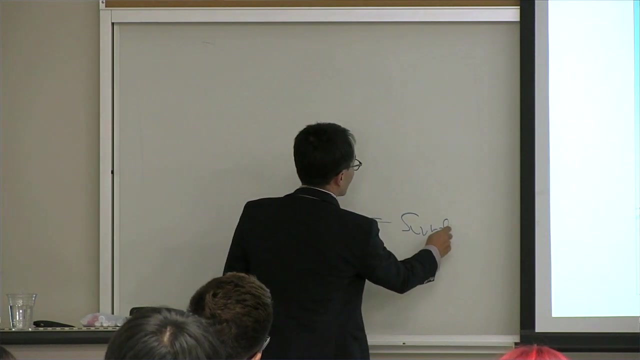 On the bottom. So let me start with. let me start from the beginning. So if we have more aerosol in the atmosphere, then surface temperature is going to be increased or decreased. So let's draw a figure: This is surface. Then you have, let's say, cloud, white cloud in the atmosphere. 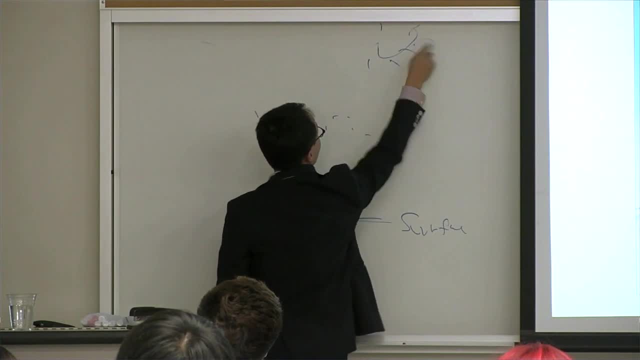 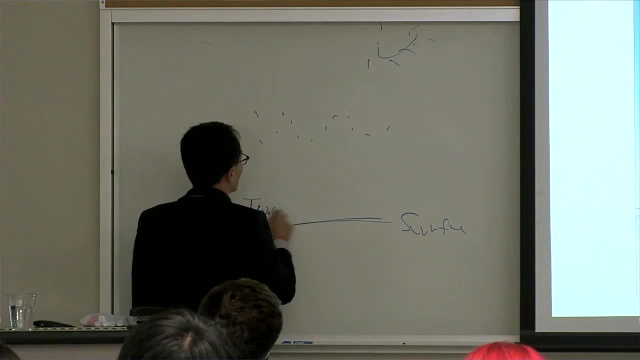 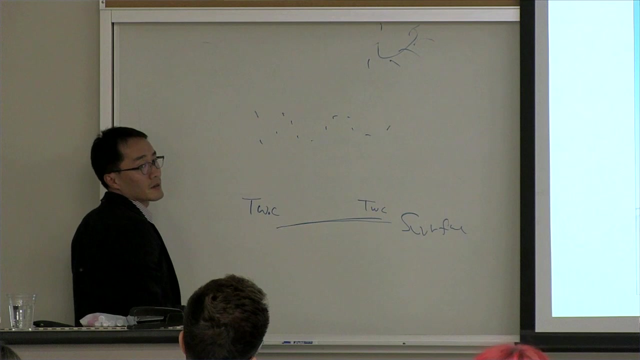 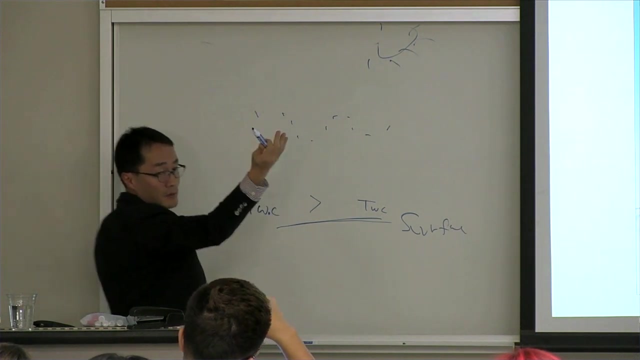 And then you have sun here. Then temperature without cloud, temperature with cloud. So which one is going to be higher, without or with? With Without is going to be higher, So let's replace this cloud as the air pollution, which is basically particle. okay. 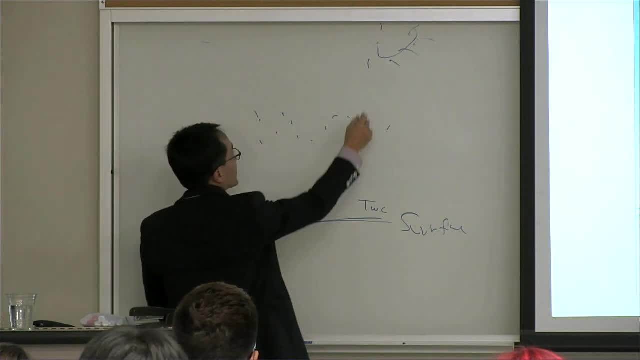 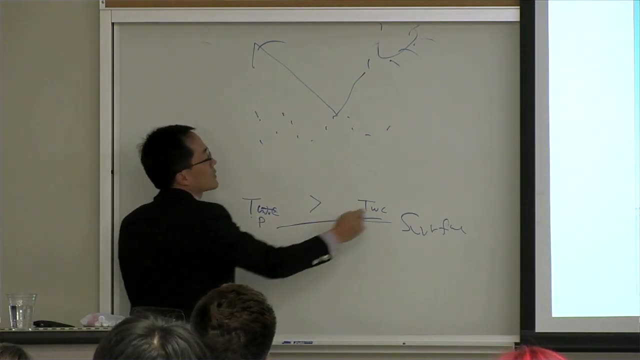 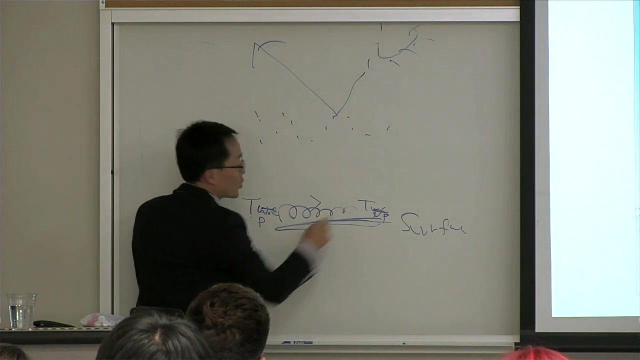 So air pollution- if there's air pollution in the atmosphere that reflects the solar radiation, then temperature on the surface in pollution scenario is higher than not polluted surface, right? So what's going to be happening when surface gets hotter is that there's going to be more turbulence. 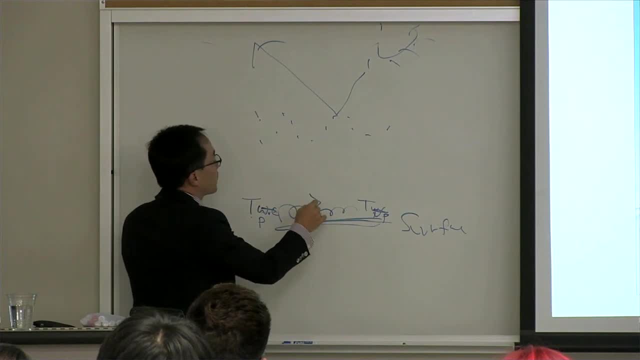 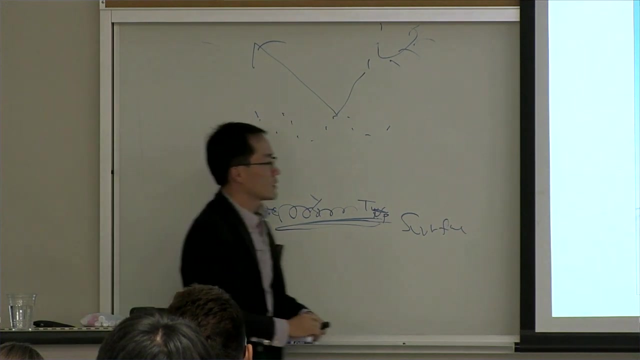 that actually makes more winds, So in. So temperature is actually. This is the other direction. So temperature in non-polluted atmosphere, the surface temperature is going to be higher than the polluted environment, So the wind speed in polluted environment is. 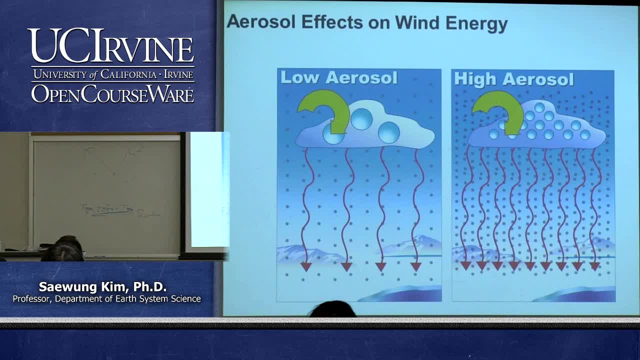 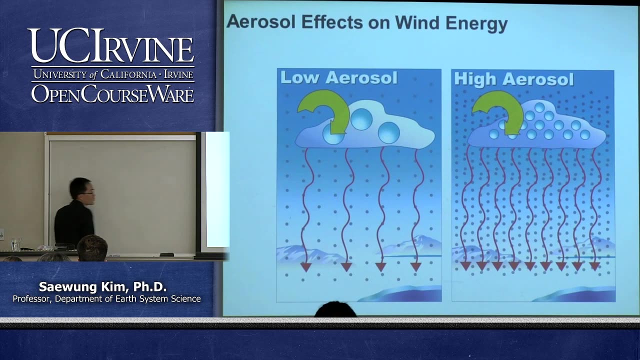 We are thinking that it's going to be higher And then pollution cause less wind, So that can affect on wind energy production. That's what we talked about before, So this is relatively straightforward. So what I'm trying to explain today is a little more complicated than that. 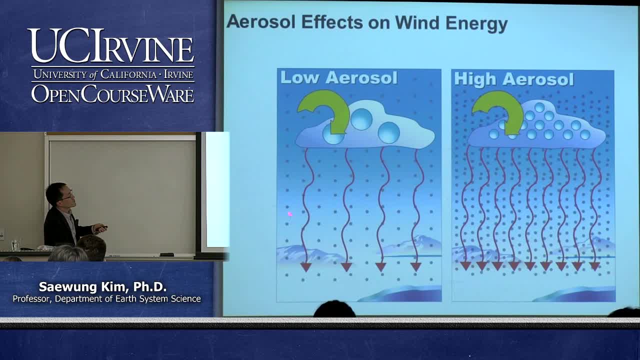 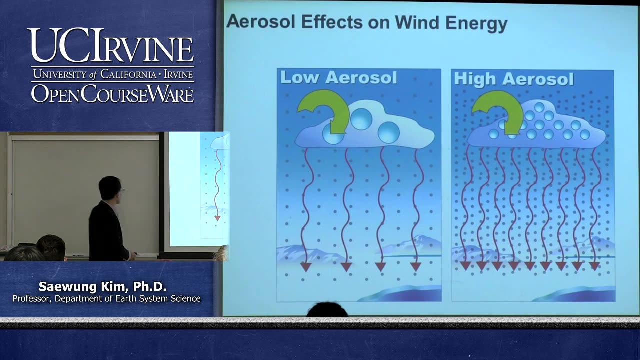 So let's also imagine two different scenario. One is less aerosol, so less polluted environment. Then the other one is higher up aerosol, which means that more polluted environment. right? So let's assume There's a 10 particle. 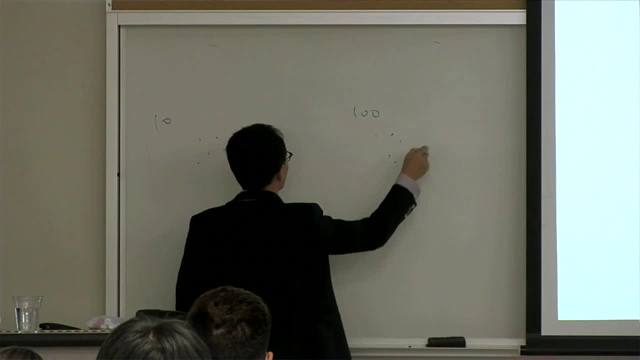 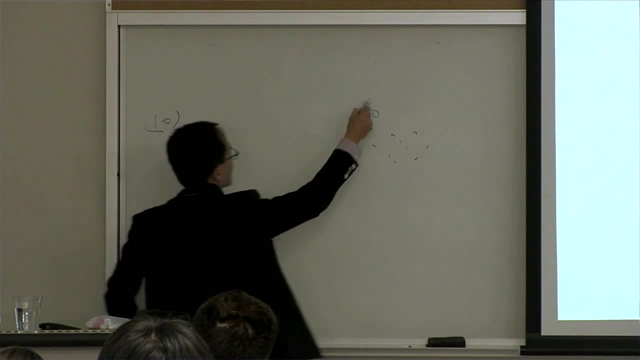 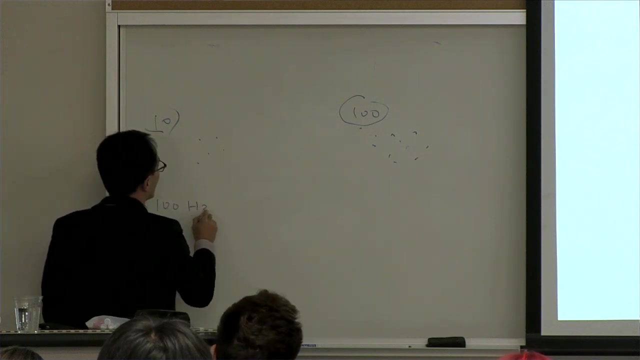 And then there's 100 particle. I'm not going to put the Make the 100 particle in the drawing in here, but let's just see the number. So this is more polluted right? And then let's assume there's 100 water vapor. 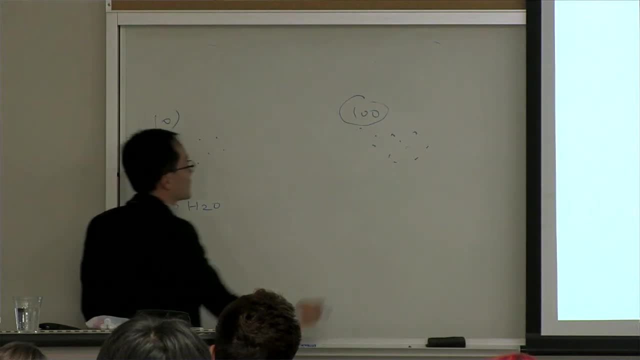 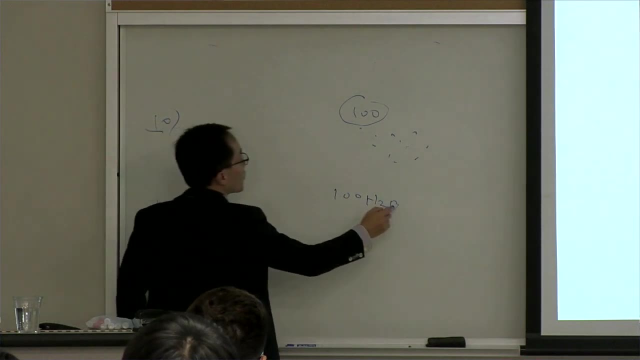 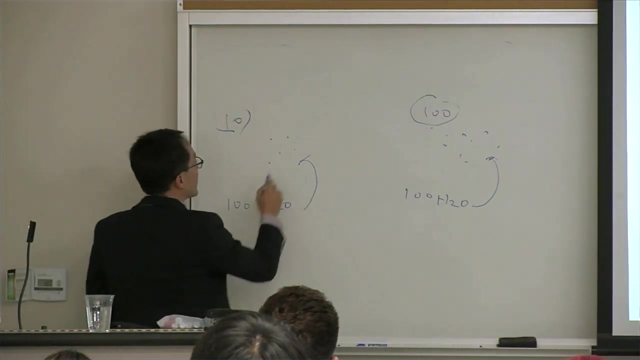 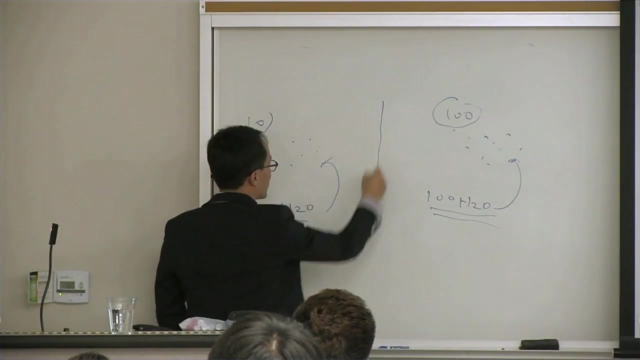 So water, H2O molecule in the atmosphere. So if this 100 water molecule all observed into the particle and then make the cloud, then how many water vapor per particle, each in different scenario? right, Let's take a look. So what's the number here? 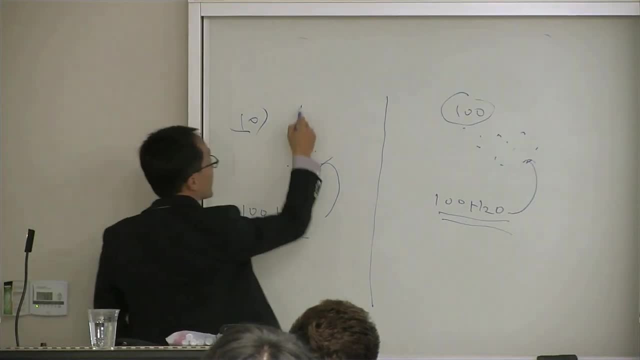 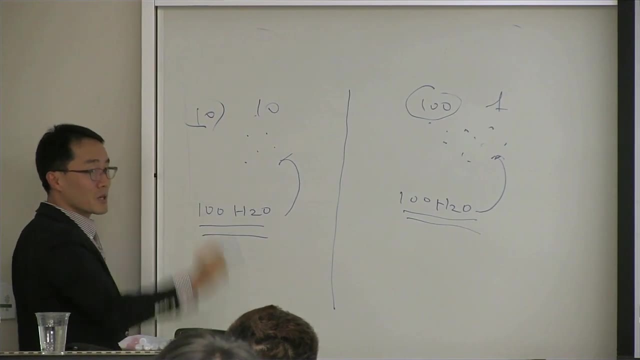 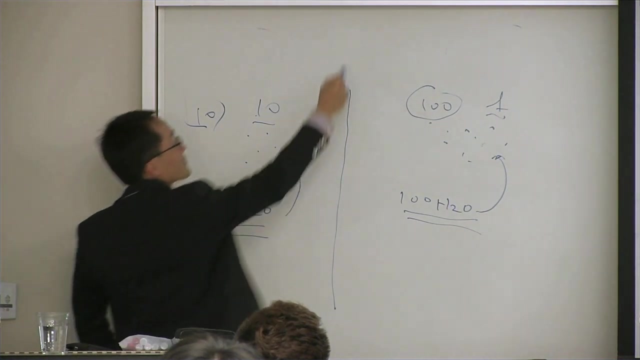 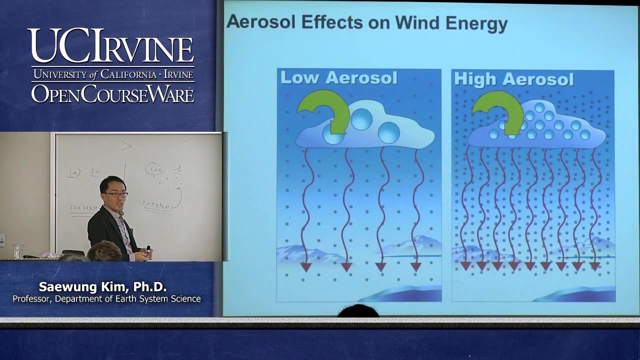 It's not a trick question, Yeah, 10.. That's one, right? So, in terms of cloud particle size, which one is bigger? It's not a trick question. Again, right? Cloud particle size. Then how rain initiated cloud particle getting bigger and bigger? 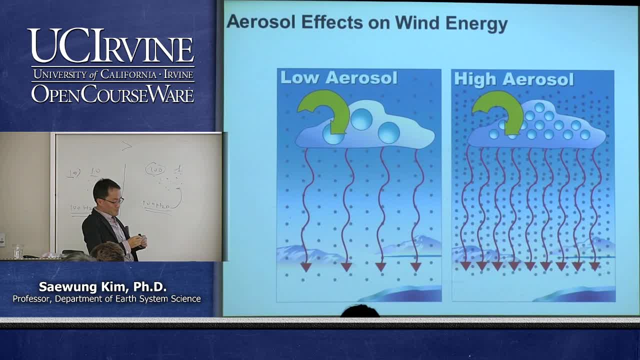 and then it's just dropping. That's, by definition, rain, right? So in the less polluted environment, then we are likely getting more rain, right? In more polluted environment, the cloud is going to stay longer, but not going to be participating into the surface, okay. 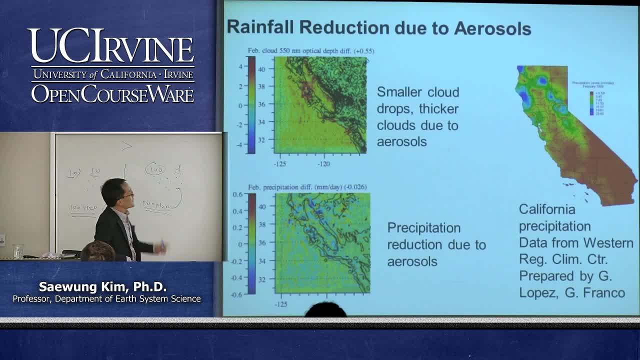 So if we just put this concept into the model and then if we just simulate the rainfall in California, more aerosol due to pollution cause less rain means less water on the surface. So that's basically this simulation results indicate that less rainfall caused by the pollution. 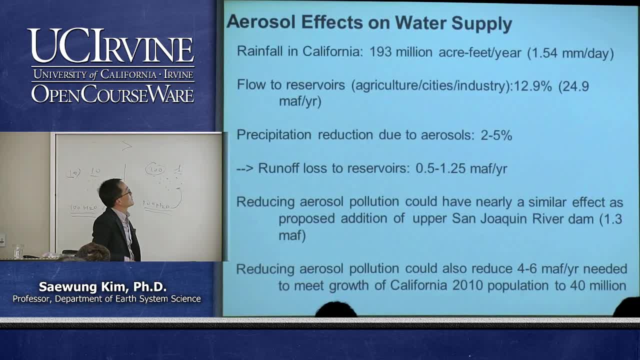 because of basically this concept. So this is summary. So where is the bottom line? So the precipitation reduction due to aerosol which is caused by the pollution, we're expecting about 2-5%, which is actually a lot. A state like California has pretty dry environment, okay. 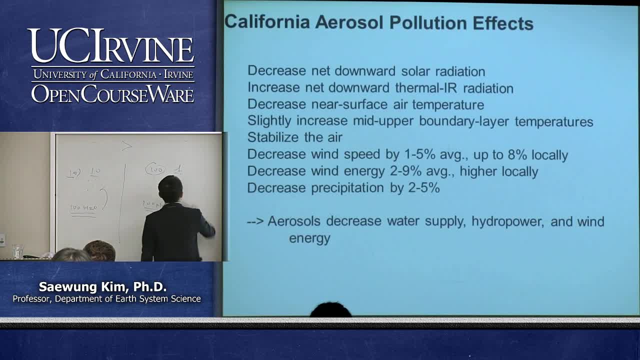 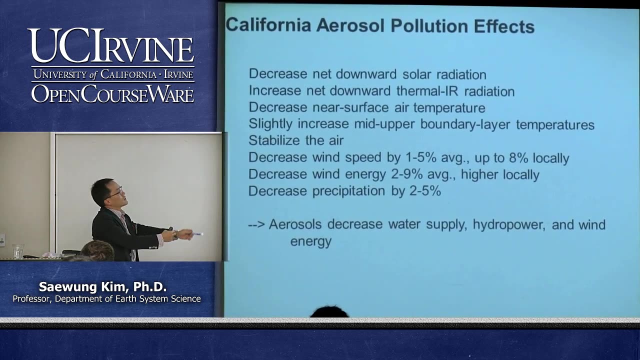 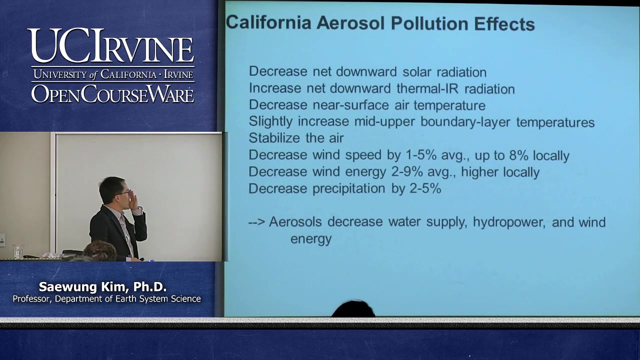 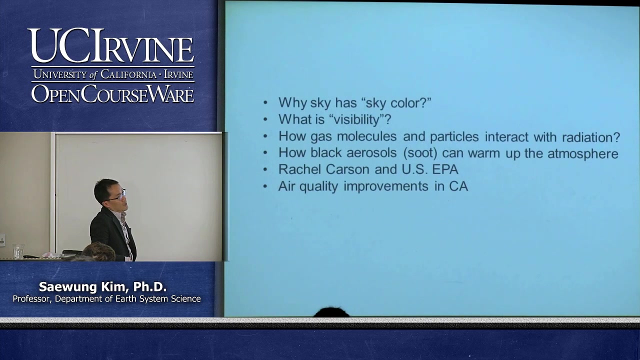 So that's the last thing, that last discussion about interaction between pollution and weather. So today we will discuss two big topics And then two chapters in your textbook. One is visibility and then the other one is environmental regulation. So visibility, so basically we will start discussion about why sky has color. 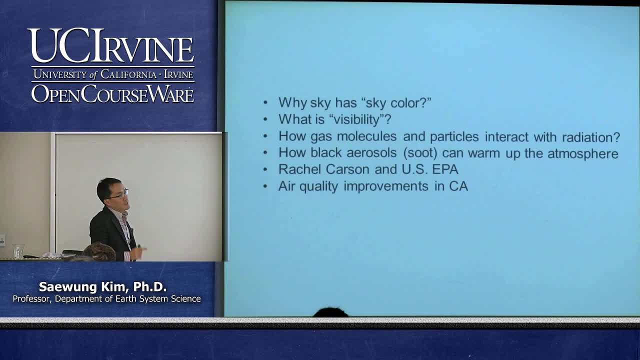 why sky has blue color and then how the gas and aerosol actually interact with the solar radiation. It's potentially visible. And then we will talk about some specific particle like soot and how the soot, that basically black particle. 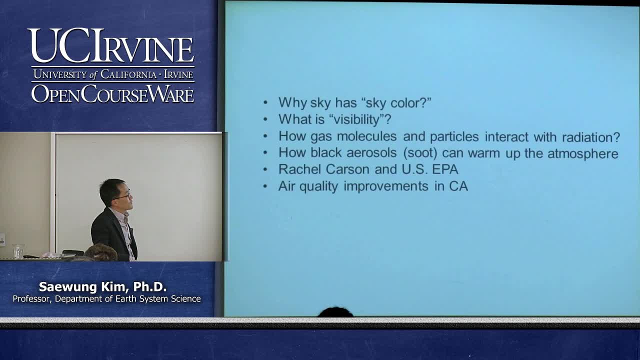 can warm up the atmosphere And then we briefly actually discuss about EPA and then current political environment. actually, some people actually think that we should get rid of EPA, things like that. So we'll just kind of review the history about how EPA initiated. 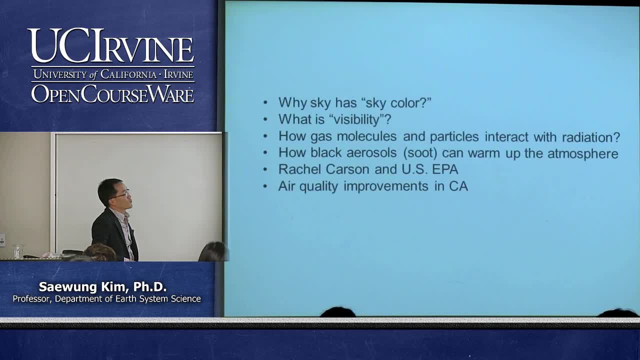 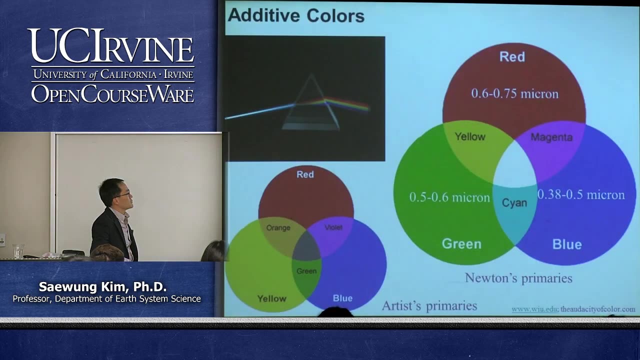 and then, what's the impact of the environmental regulation to, of course, the environment? And then, of course, I'm not an economist, but we'll discuss a little bit about the economic impact of the environmental regulation. So let's start with this one. 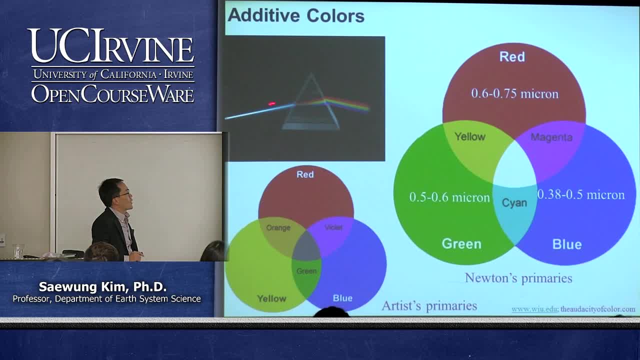 So we talked about visible wavelengths actually has so the range between between 400 nanometer to about 800 nanometer, And then in terms of micrometer, it's about 0.4 micrometer to about so 0.4 micrometer to about 0.75 micrometer. 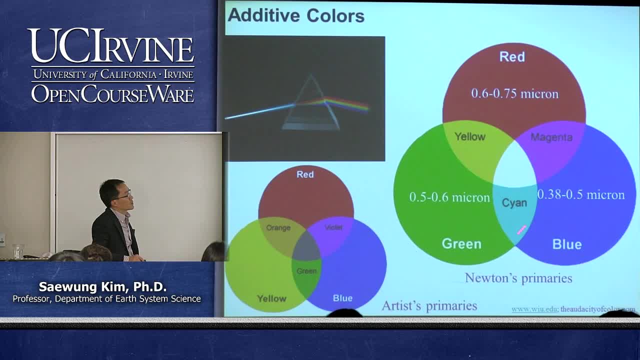 So the color range is between blue to red. So if you mix all the wavelengths between 380 nanometer to 750, it's white looking light. So that's why solar radiation looks white. But if you just mixed up color of red and blue and yellow, 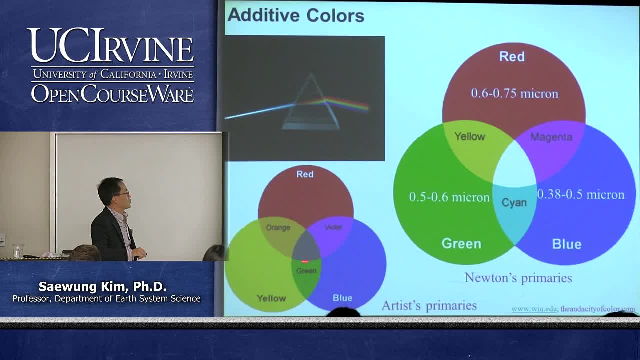 in terms of paint, it said that you will get black, But I don't know about this part because I almost I barely passed my art class during the high school, so I don't know about this, But you need to understand this thing. 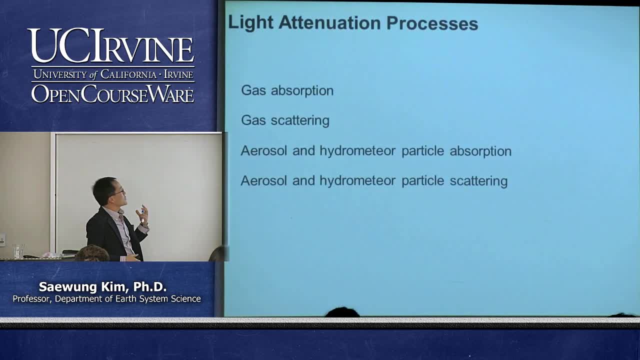 All right, So we'll discuss about two different physical processes. One is absorption and the other one is scattering. And then we talked about gas and particle in the atmosphere, right? So gas can absorb some of the visible wavelengths and then can scatter some of the visible wavelengths. 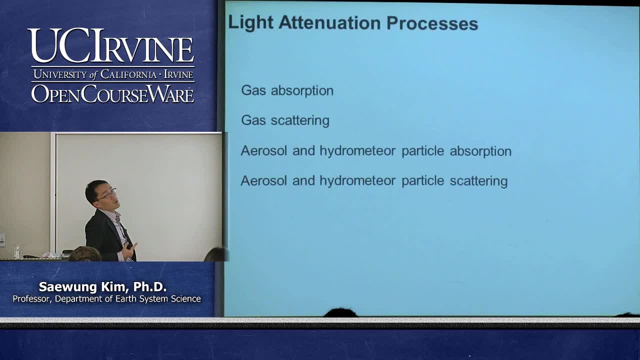 Also aerosol, and the hydrometer is basically rain or cloud. So that's so in terms of the grand schematic, you can understand hydrometer as aerosol. So aerosol can also absorb visible wavelengths region and then also scatter the visible wavelengths region too. 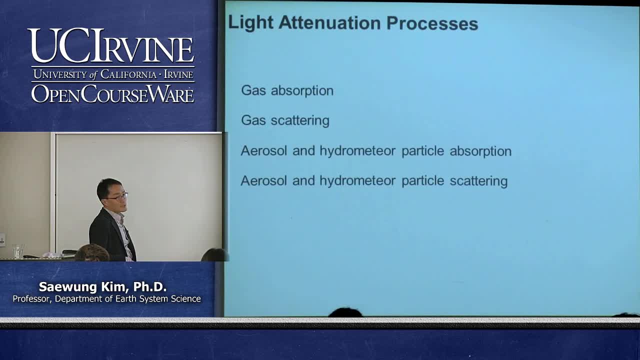 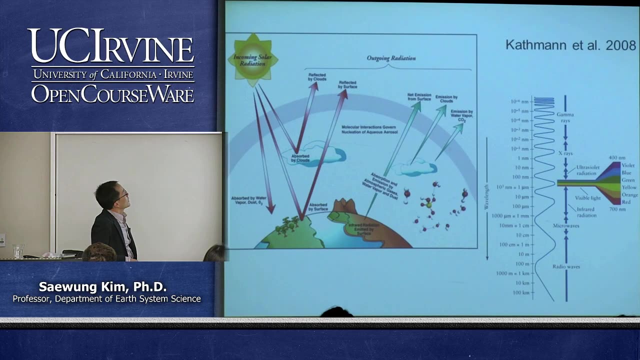 Okay, So those two physical processes- and then it's gas and aerosol also interact, can make the absorption and scattering in the wavelengths region of visible from the sun. So let's try to kind of take a look at the grand schematic how visible wavelengths is coming into the atmosphere. 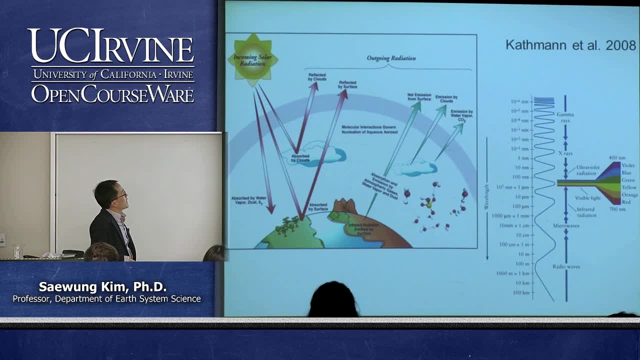 So sun. so what's the dominant energy that is coming from the sun? It's the visible right- We know about it- And then a little bit of the UV, and then a little bit of the IR. So this is the. we went over this thing several times. 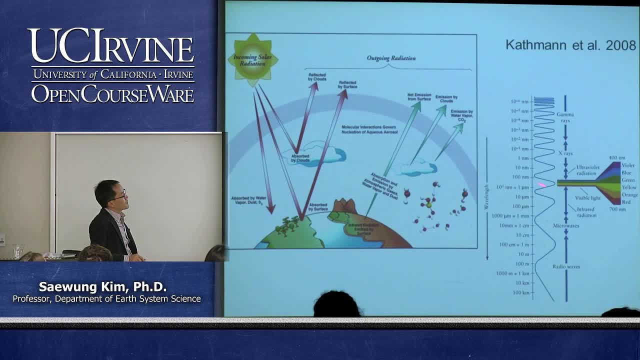 So UV is the higher energy than the visible, and then IR is the lower energy than the visible, And then we sense IR wavelengths as a heat. So that's why we call it sensible heat, And then visible wavelengths. by definition we call it visible because we cannot. 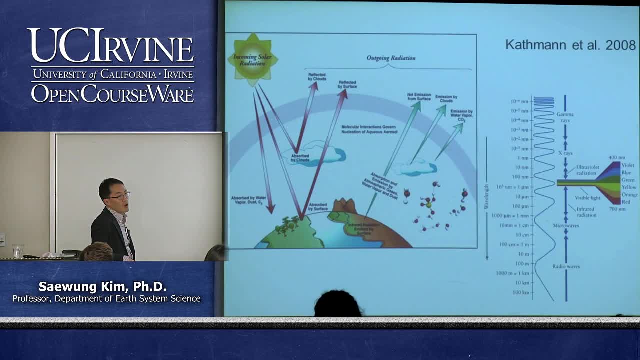 we can see that wavelength as different color, And then again, if you mix up this whole wavelength, it's going to look like a white right. So sun, solar radiation coming into the atmosphere. And then again we talked about scattering and absorption. 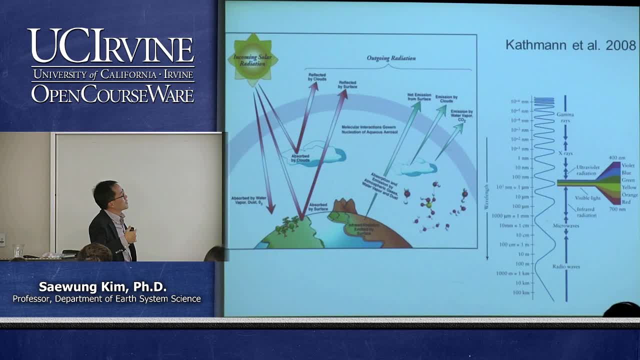 It's going to be interacting with the atmosphere constituents, with gas and particle, And then some of those things are going to be reflected away And then some of that thing is all the way go down to bottom right And then energy absorbed by the earth. 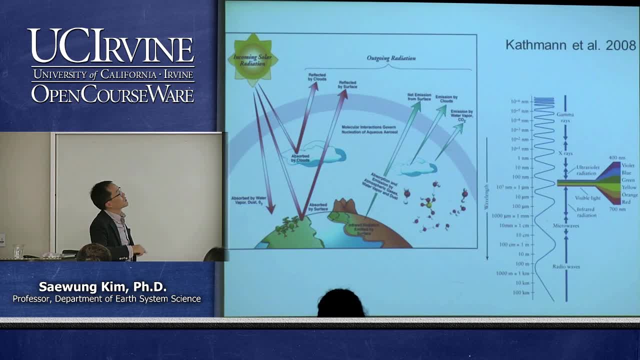 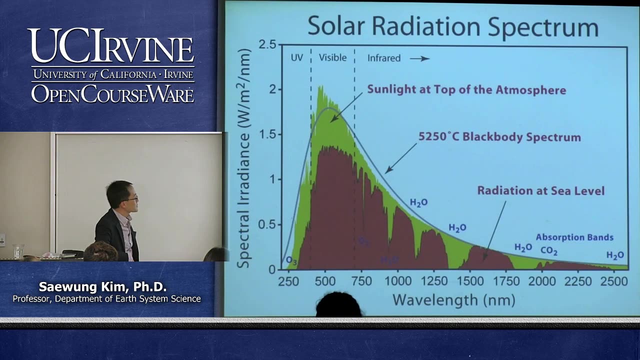 And then earth also emitting energy, mostly UV region, IR region. I'm sorry about that. And then the IR is sensible heat, So earth is emitting energy as form of the heat right To the atmosphere. So this is solar radiation basically. 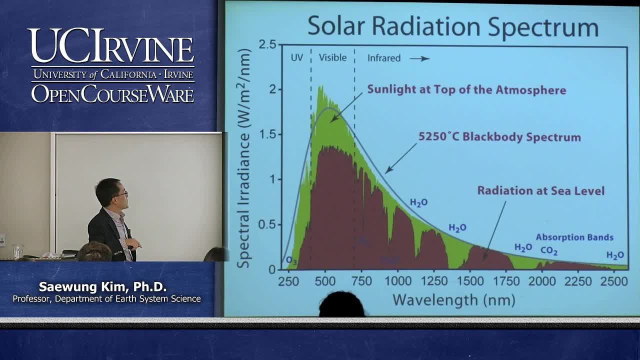 So basically, the physicist made a model and then predicted how, what kind of energy is emitting from the sun and then how much of that energy is going to get into out of the atmosphere. So that's basically this line right here is basically the predicting result. 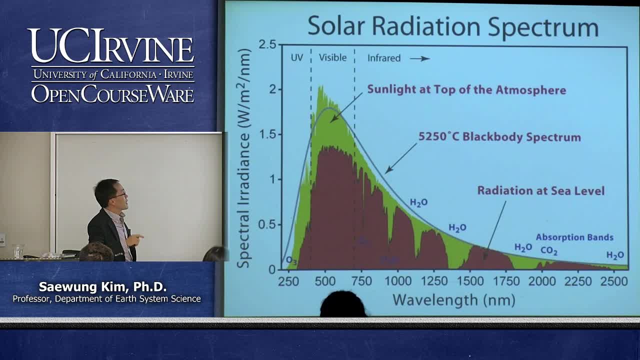 right. And then actual observation out of the atmosphere is in yellow right here. So basically the model that's set by a bunch of physicists agrees pretty well with actual observation. if you take a look at this yellow thing, The red is our actual observation on the surface. 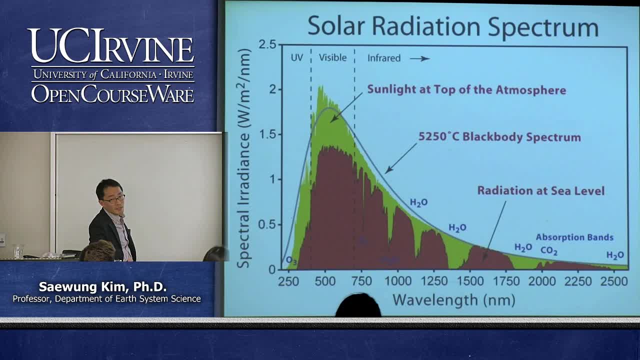 So differences between this yellow and red is basically interaction between atmosphere and then what's in the atmosphere: Gases and particles. So interaction between gases and particles make the least energy actually get into the earth's surface. Okay, And then, if you take a look at some wavelength region, 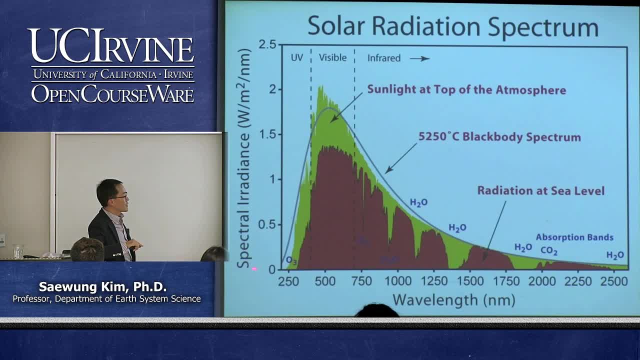 for example, low 300 nanometer, which is very short wavelength region, and then higher energy. not much of the UV actually penetrate into the earth's surface right, Because the ozone layer in the throughout sphere observe those high energy wavelengths. Okay, 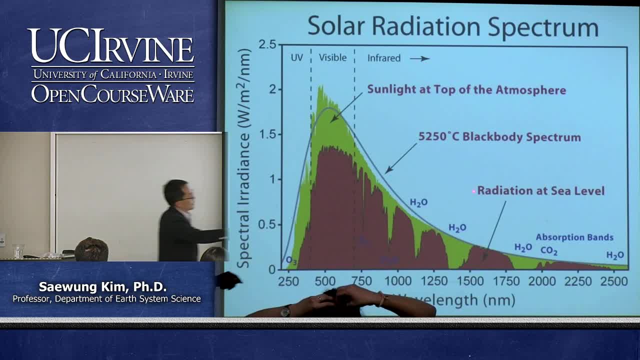 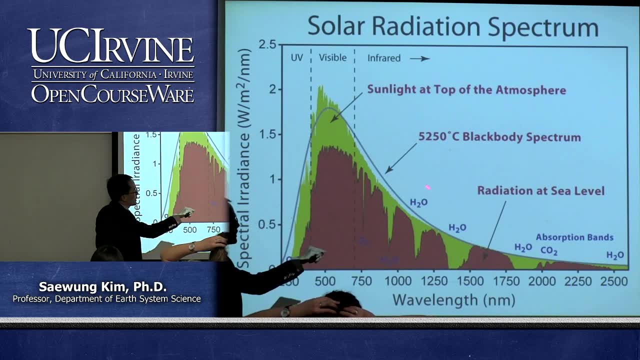 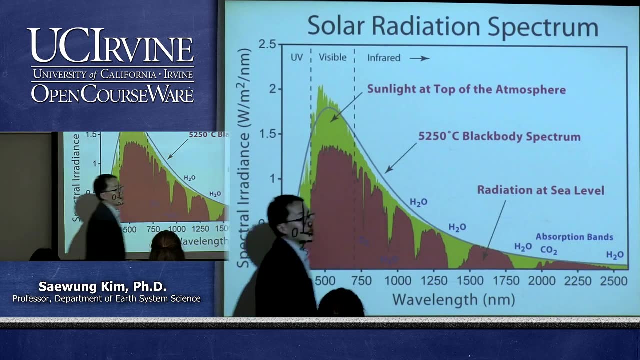 Now, if you take a look at this UV wavelength region, a lot of not UV IR. I'm sorry about that. the IR wavelength region, a lot of IR actually absorbed by water vapor. So this region right here, that IR region, which is sensible heat. 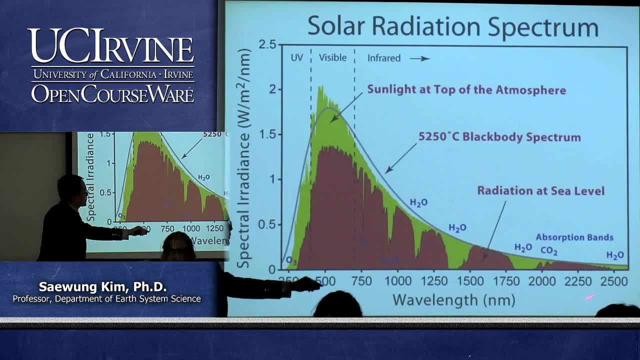 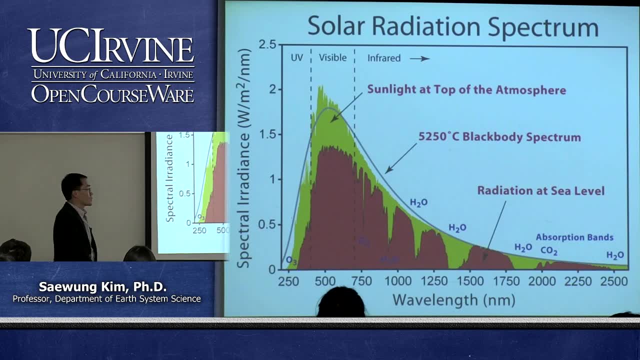 so we need to understand interaction between atmosphere and this wavelength to understand global warming, because global warming is warming of the atmosphere and then warming, by definition, is sensible heat, which is IR wavelength region, And then this wavelength region, UV, basically to understand the stratospheric ozone. 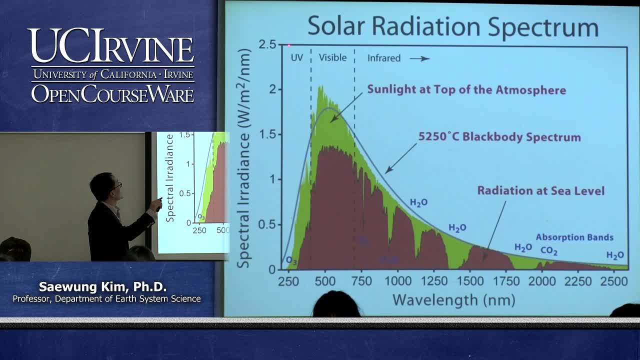 the benefits of a stratospheric ozone, we need to understand this wavelength region, UV. So today we will talk about this visible wavelength region. what actually cause this amount of decrease of energy from the top of the atmosphere, which is about 100 kilometer above the altitude? 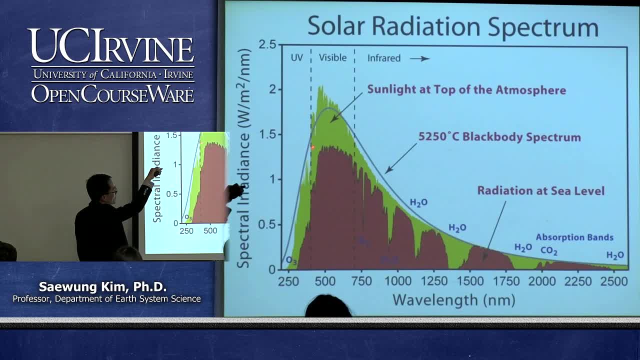 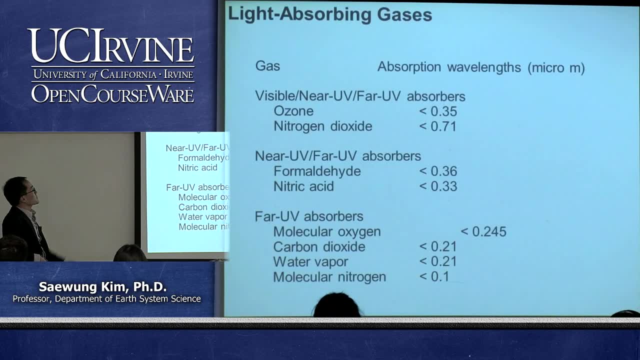 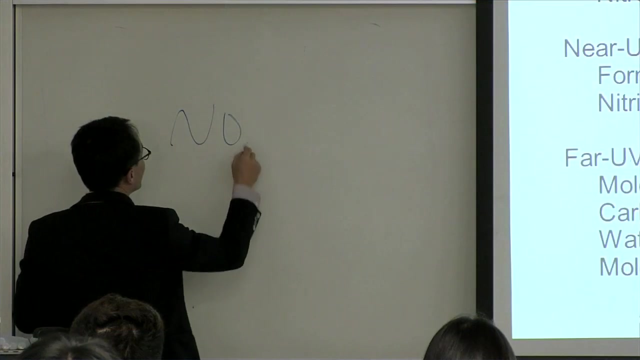 from the surface and then the amount of energy we are getting on the surface. Okay, So that's, this is the introduction. So absorption, So we already discussed about a couple of example, how gas absorbing energy, For example. we talked about this 100 times, right. 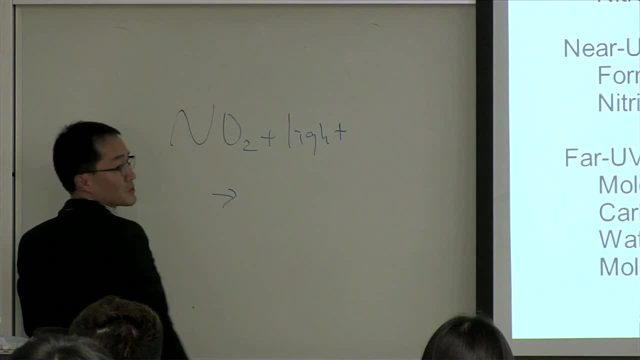 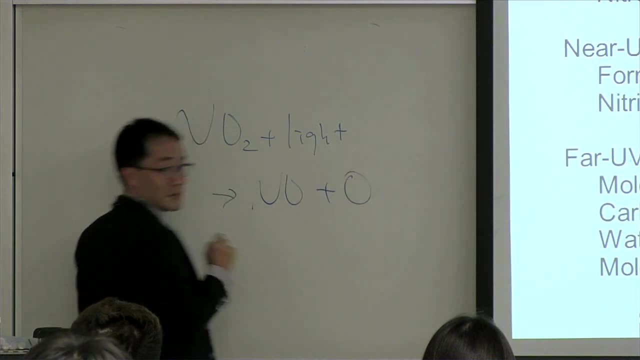 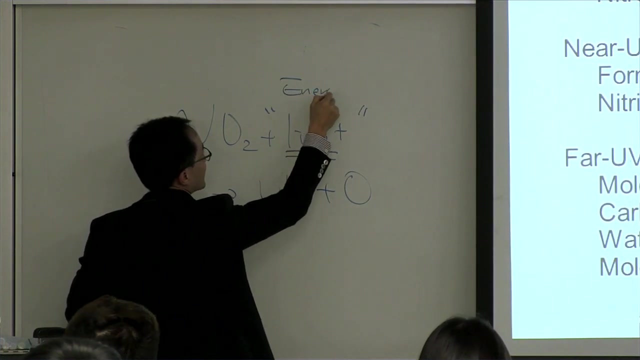 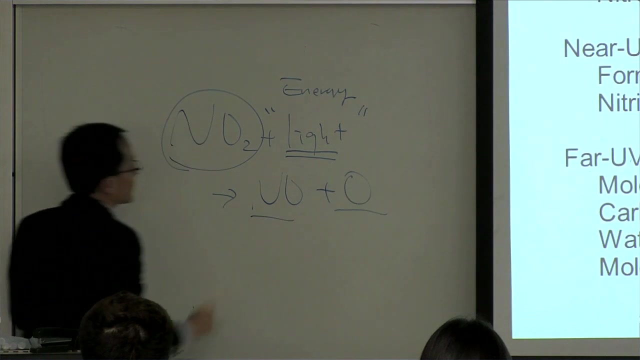 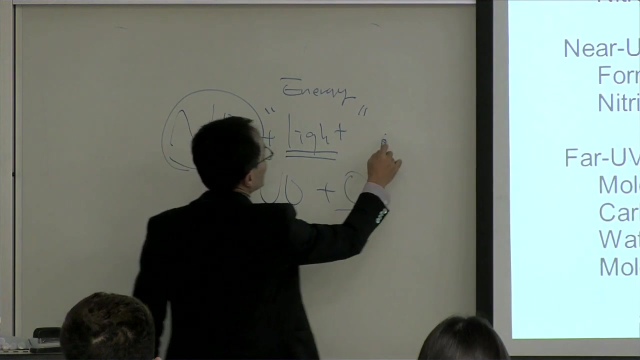 Light. So what's going to be happening, Right? So this light, which is energy, basically absorbed by this L2 molecule, and then that energy break the bonding between NO and oxygen. So that's the example of the absorption of the visible wavelength region, and then this is below 120 nanometer, right? 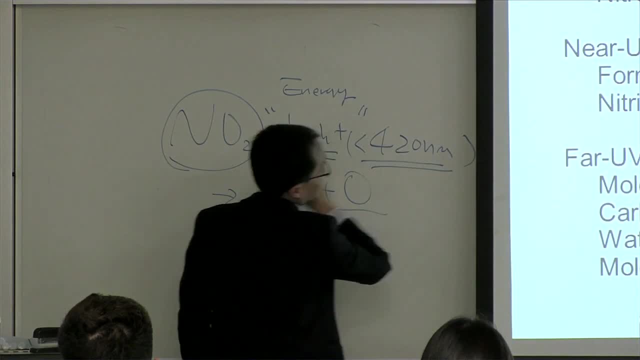 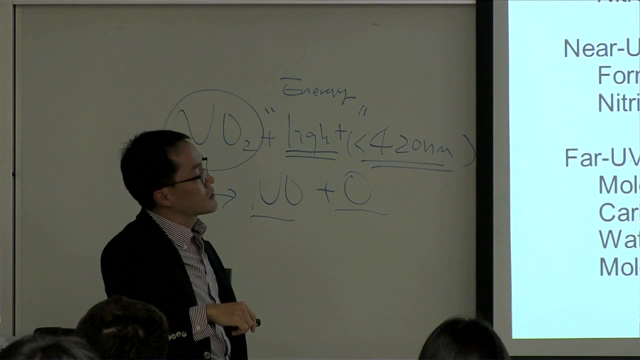 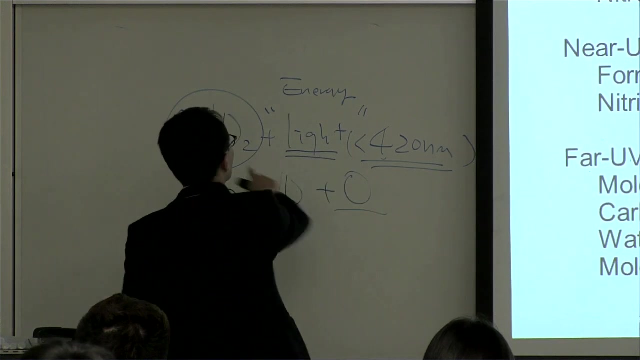 Of the light. So this is visible wavelength region. So that's it. is this light at 710, 710 nanometer. So this is active region. So below 420, every photon that observed by NO2 will cause this photolysis. 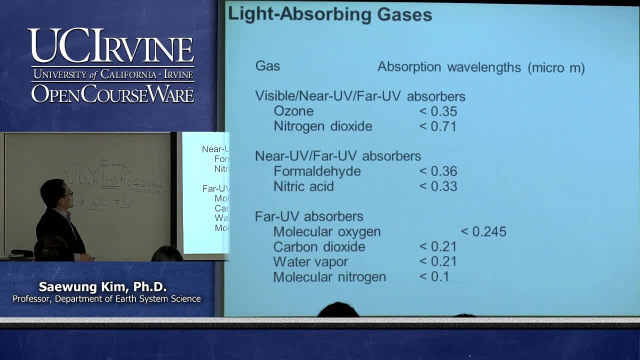 But the probability of the reaction. this reaction is going to be decreasing quite fast, Up to 710, and then the wavelength region higher than 710 would not cause this reaction, Which means that the photon higher than 710 nanometer is not cause this reaction right here. 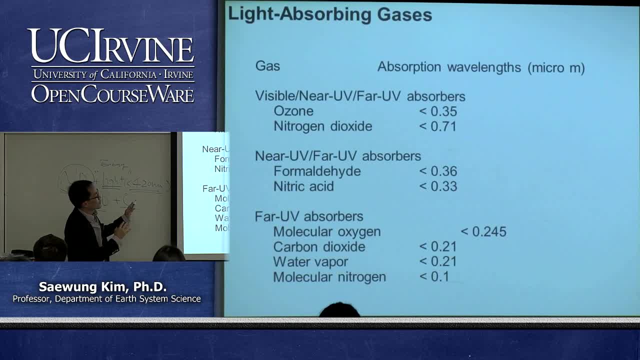 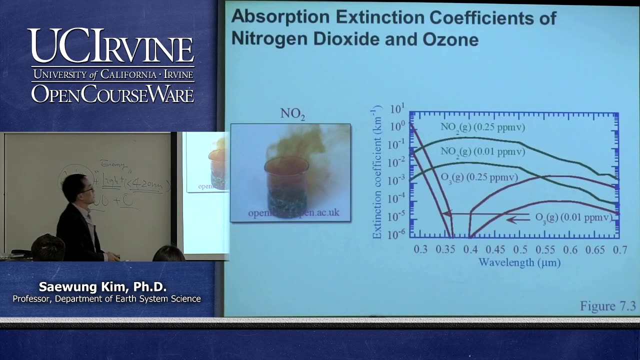 So the important thing is the nitrogen dioxide, And then there are a couple of other example, other molecules that can interfere with the visible wavelength region, But mostly NO2 in the atmosphere interacting with the visible wavelength region By absorption. Okay, So that's. we discussed why. 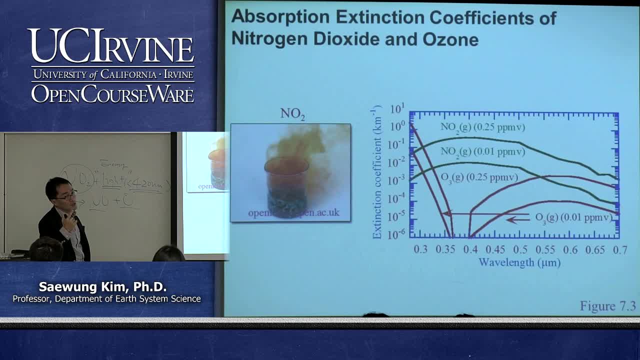 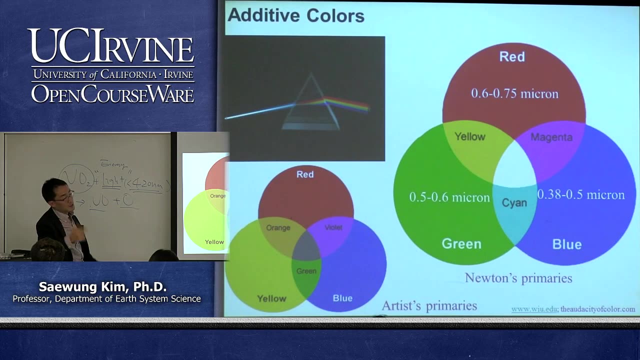 that thing is NO2, when NO2 concentration gets high, it looking like brown because it is absorbing blue wavelength region. So if you just mixed up red and green, then it's going to be brown. So that's why NO2 looking like brown, right? 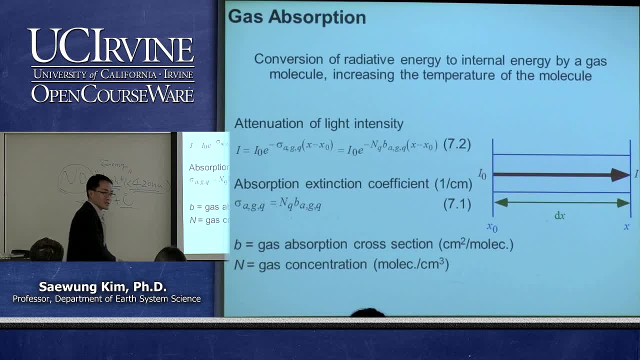 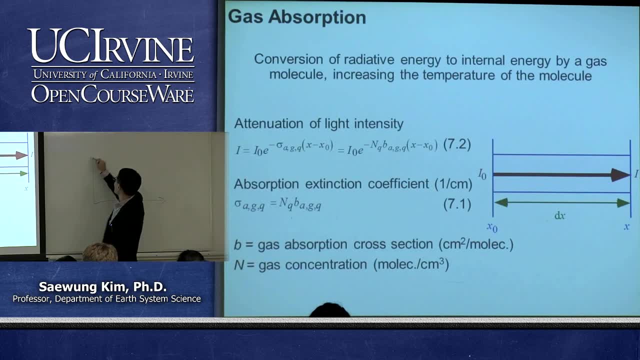 Talked about this. Okay, again, our job as a scientist make this thing pretty boring by employing equation. So I'm not going to enforce you to remember this equation, but I'm going to try to what this each parameter means, So don't get freaked out. 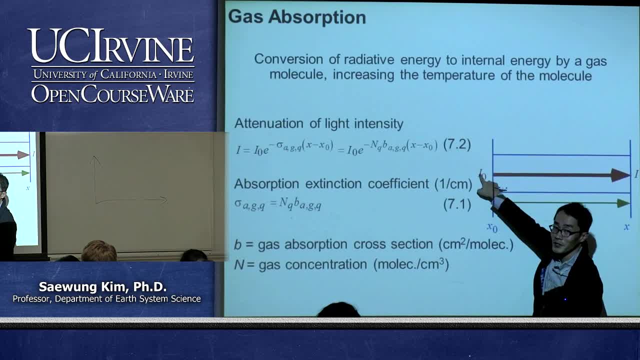 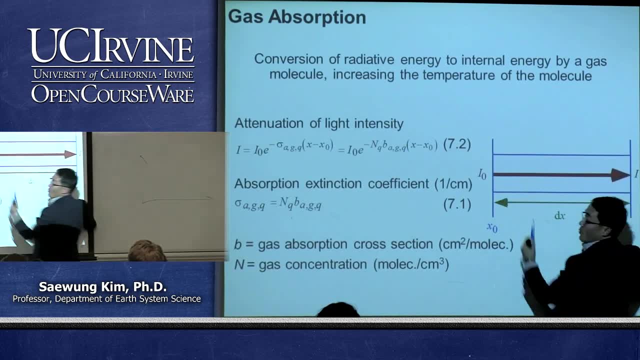 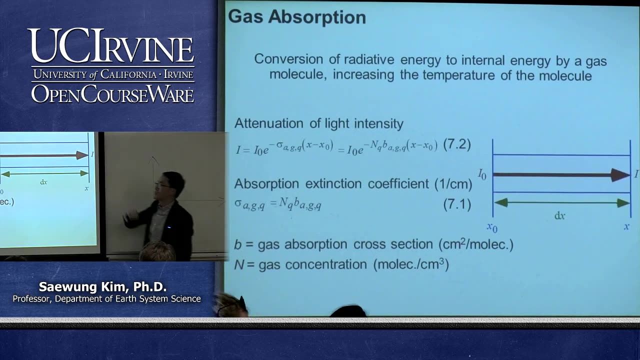 It's relatively easy concept. So that's: the light is right here, And then we are measuring the light intensity in this sand. So this is length of the path of the light, right? So that's basically x, That's distance. So 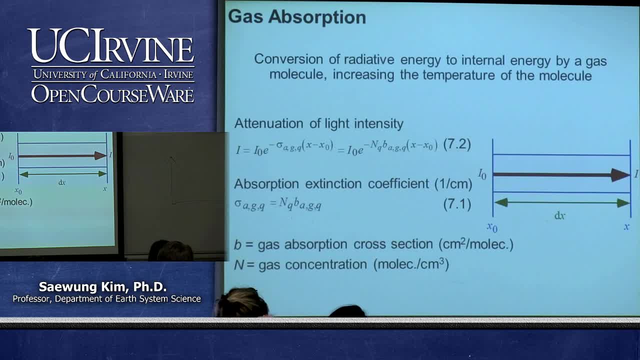 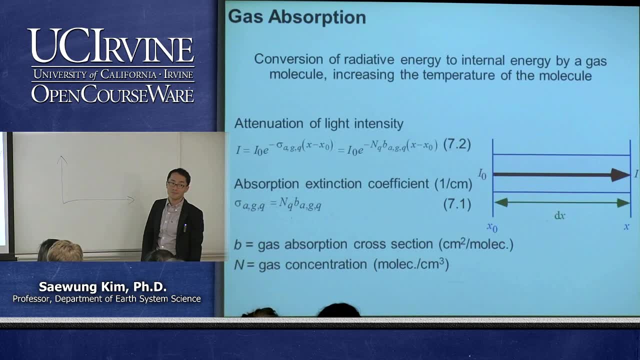 if you have a longer distance, when air is homogeneous, then the absorption is going to be higher or lower: 50-50. higher, right, Because there's more air molecule is in there, right? So basically, this is exponential Decrease. 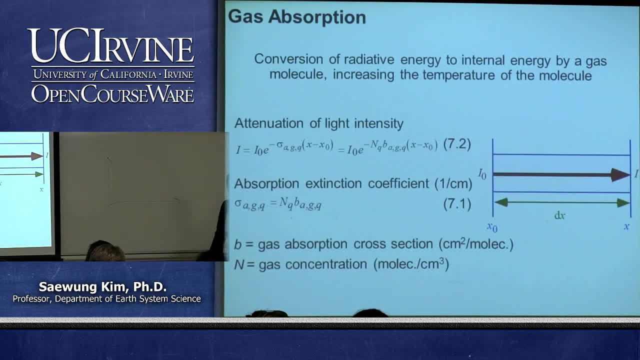 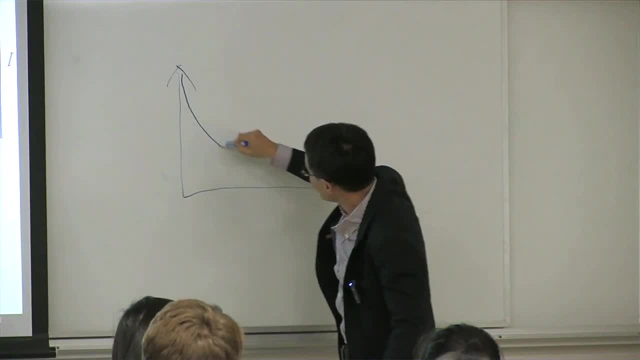 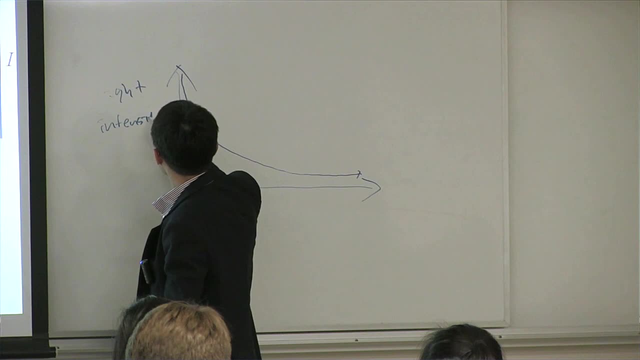 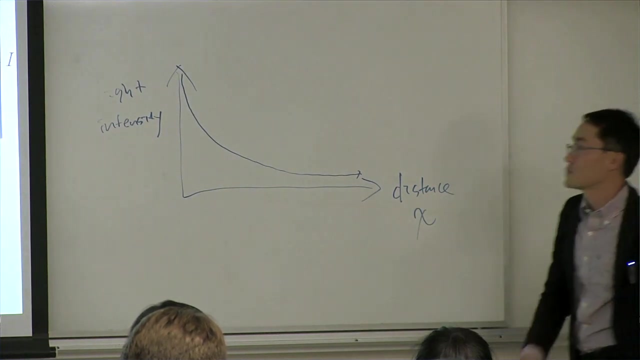 And then I explained that exponential decay is the most famous thing in the nature that usually absorb. So exponential decay is expressed like this right, Basically light intensity, And then this is distance, Which is x. So if you're going further, 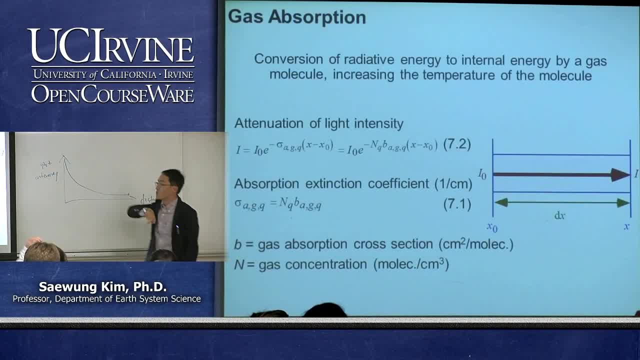 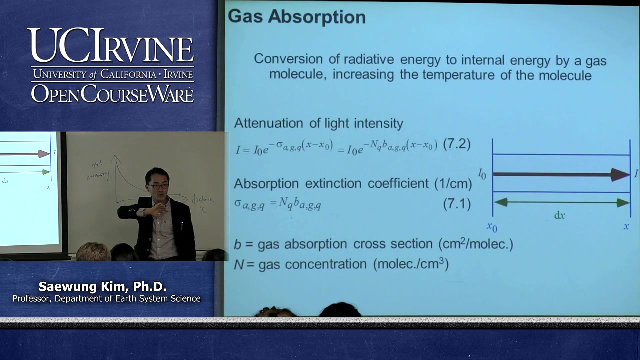 because there's going to be more gas molecule that can absorb visible wavelength, you will have less light at the end, right? And then there's couple of other characteristics we need to consider. One is concentration of gases: right If you have more higher? 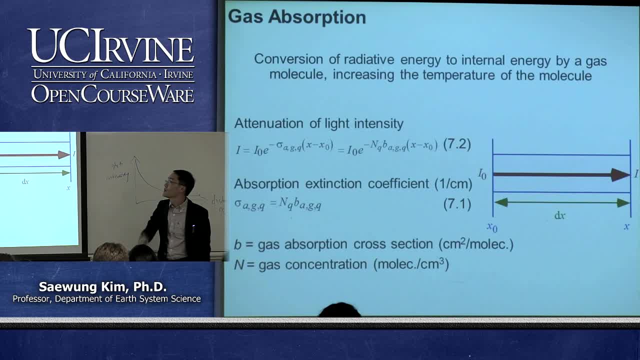 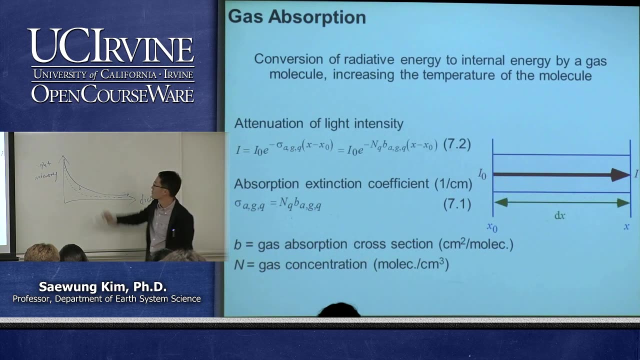 concentration of gases that can absorb light, then your decreasing rate is going to be higher, right? So it's going to be either like this, which means higher concentration, right? If you have a lower concentration, decreasing is going to be slower, right? 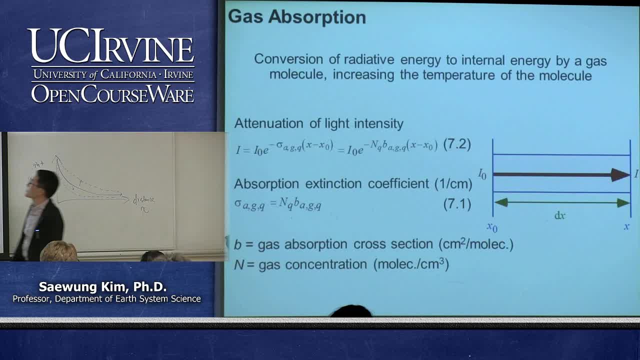 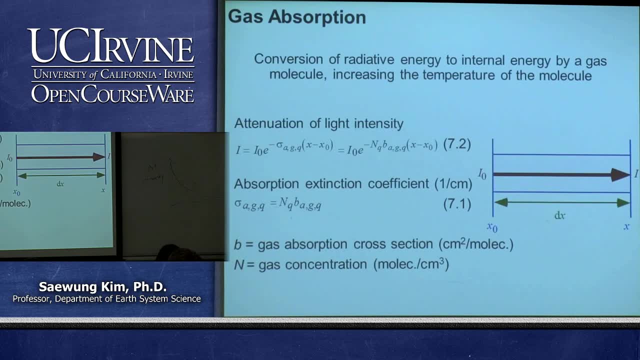 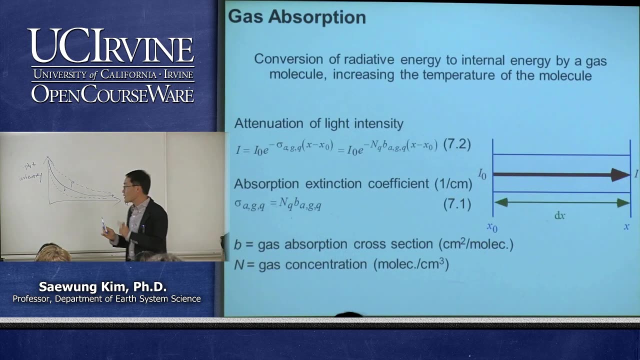 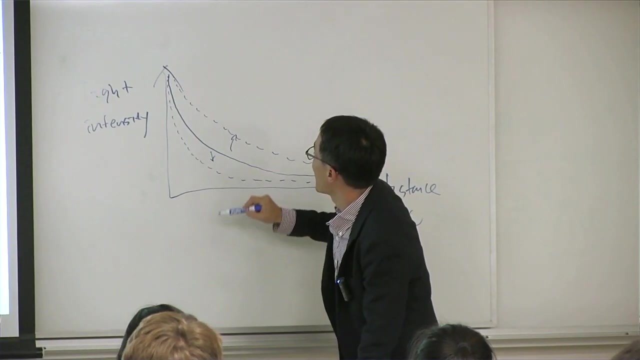 Got it. So another thing that expressed right here the gas absorption cross-section is that depends on the characteristic of molecule, that how much light can actually absorb by each molecule. If that specific molecule has characteristic high absorption, then your absorption curve will look like: 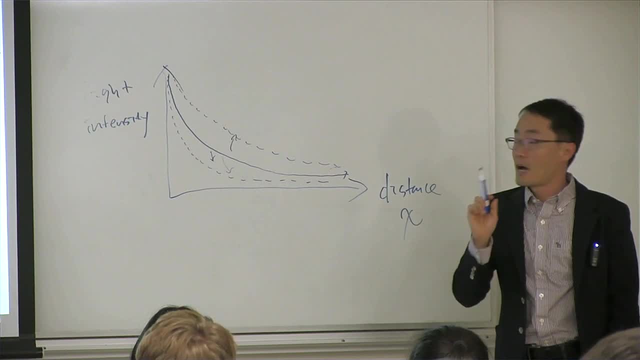 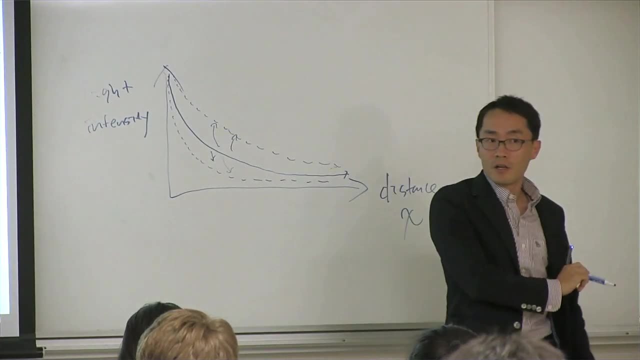 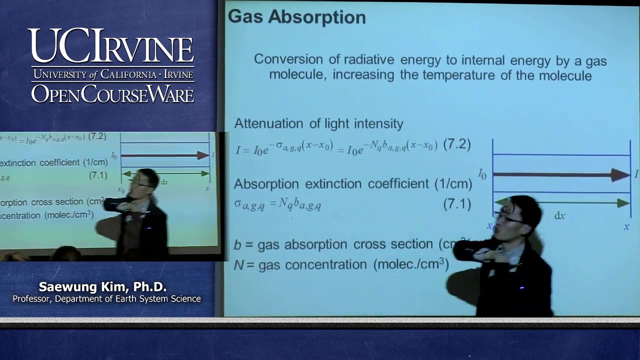 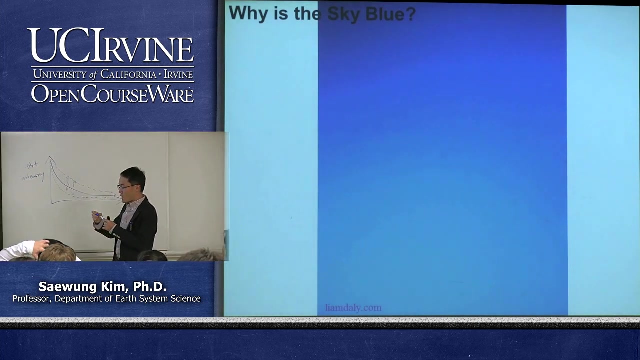 this and then that gas molecule has tendency for the less absorption, then your curve will more look like that way. okay, So that's three different parameter that plug into this equation. Okay, So that's that. So there's an interesting question: Why? 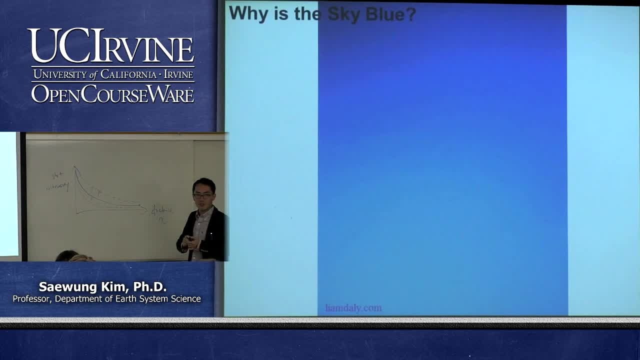 is the sky blue? Who can answer this question? Anybody? Why sky looks blue if there's no cloud? Nobody, Nobody. Go for it. What's that Rayleigh scattering? That's a good answer. What's the Rayleigh scattering? 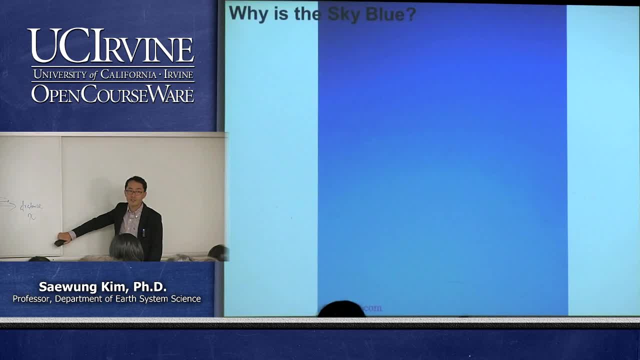 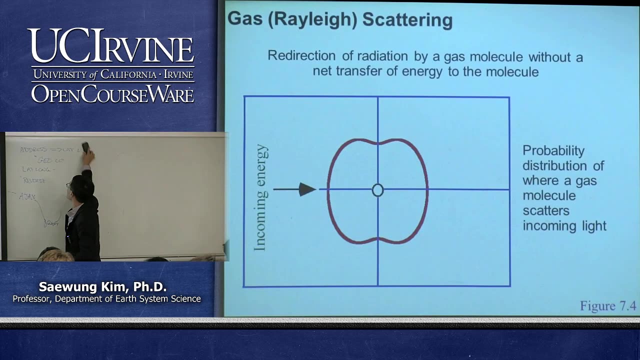 So that's Rayleigh scattering, That's scattering. And Rayleigh scattering is about scattering of of the gas molecule, of the gas molecule. So we are not really talking about this thing. So next slide. So that's Rayleigh scattering. So basically, 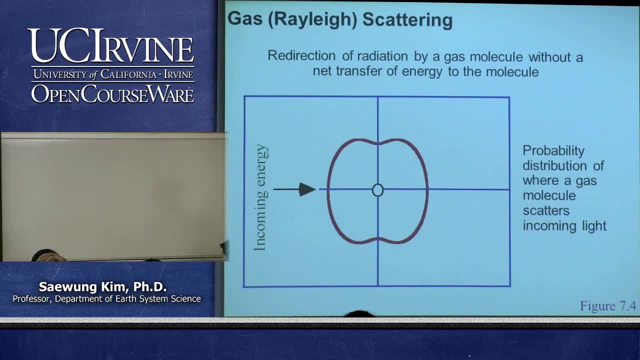 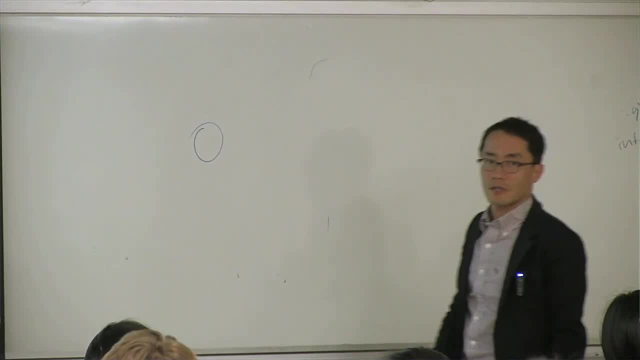 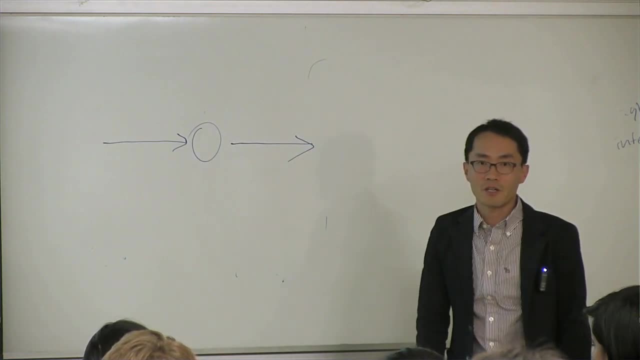 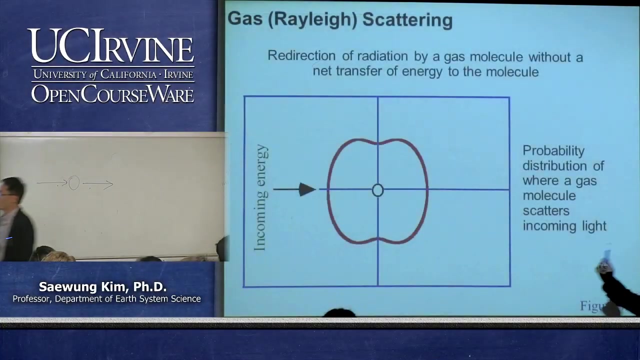 what's the difference between absorption and scattering Anybody? So this is gas molecule. Light is coming in here. There, Absorption basically absorbs some of the energy from the sun and then use that energy something else, in this case, breaking the bonding. 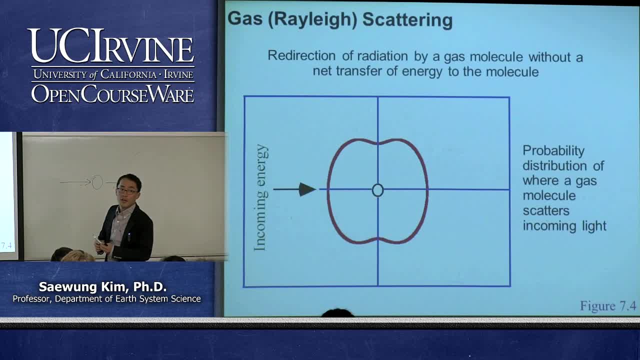 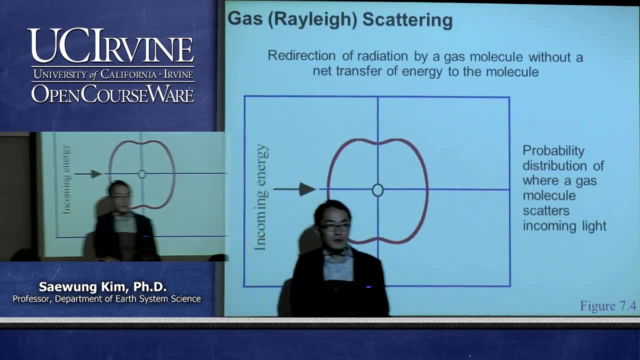 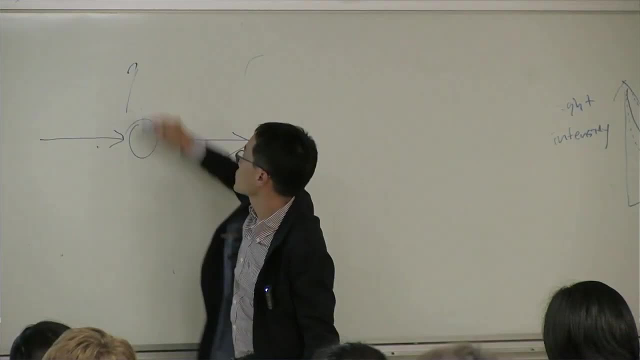 in this case breaking the bonding. So energy is taking away from the solar radiation and then used for bond breaking. Scattering, on the other hand, does not really change in terms of energy. It changes the direction of the light, So energy should be conserved. 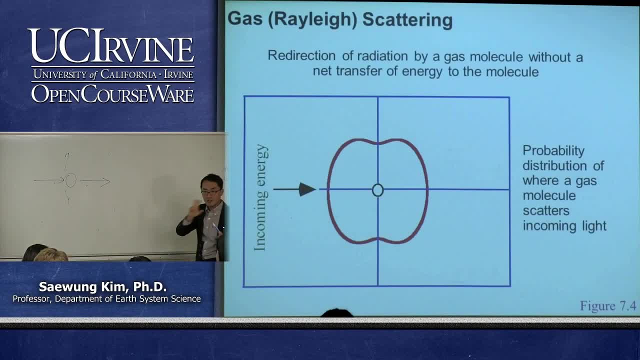 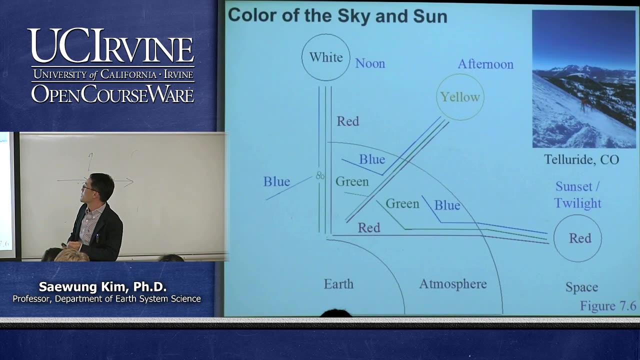 but direction is changed. So that's the difference between scattering and then absorption. So this is basically how gas molecules scatter the visible wavelengths. Okay, So this is the reason why sky looks blue, So blue wavelengths more easily scatter in the atmosphere. That means that 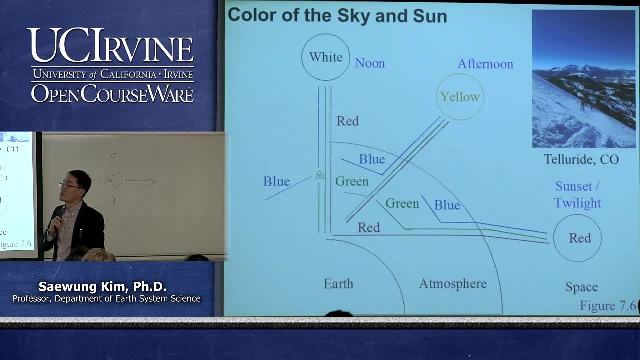 if it is noon, then the sun looking supposed to be white because it has red, green and blue, And then if you mix all that together it's just looking white And then blue is more easily get scattered. So in the high atmosphere, 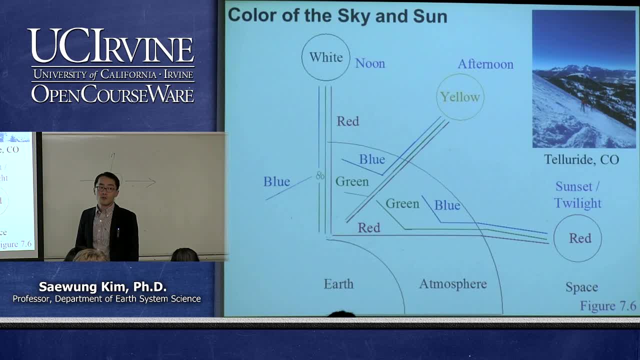 there will be blue wavelength regions- light. It's going to be scattered, so it's going to be looking blue. So how many of you actually kind of enjoy skiing up high in Colorado? more than 10,000 foot, 12,000 feet, that kind of altitude? 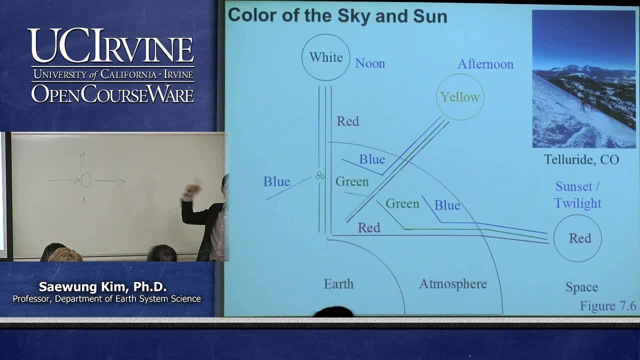 Nobody, You guys. Have you realized that actually sky out there is much blue, Very dark blue, Because you get close to out here and then it gets much more darker blue, which is shorter wavelength region. Okay, So that's Telluride Colorado. 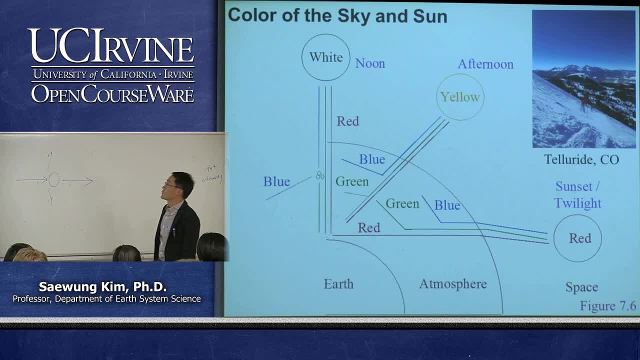 I think that's about 10,000 feet, something like that. So if you just go out there and enjoy skiing this time of season- maybe in December- it's just breathtaking, Right. So, and then this is a noon scenario. And then why? 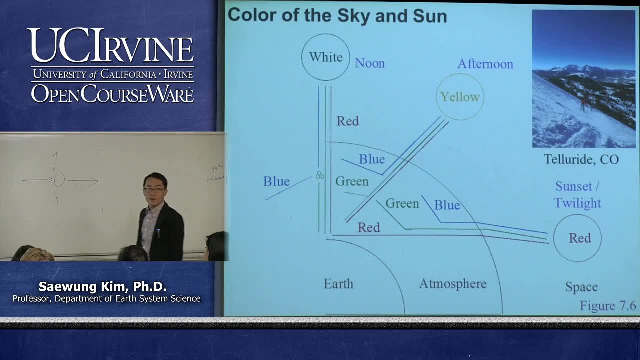 sun is looking red when it is around the time of sunset. is that so? basically, shorter wavelengths, wavelengths, visible wavelengths- is going to be more scattered by interacting with the gas molecule, the air molecule. So about in the afternoon the green is going to be scattered in the atmosphere. 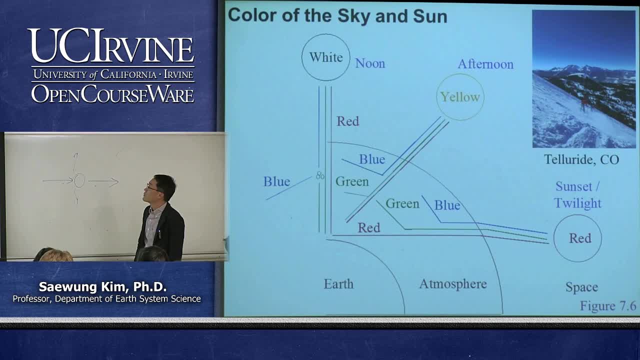 So that's why sun is going to look like yellow in the afternoon. In the sunset it has much longer path length compared with the noon and afternoon, which means that more interaction between visible wavelengths from the sun and the atmosphere. So only red can get to our eye and then 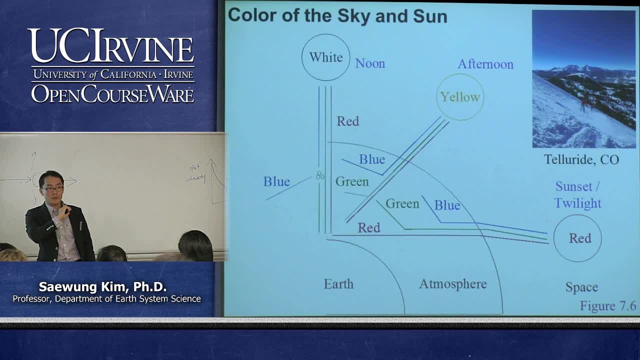 the other colors- green and blue- is going to scatter away, Right? So this is daily evolution of the color of the sun. So there's no change of the visible wavelengths that sun is emitting. So any change that is happening during the day is the path length of the. 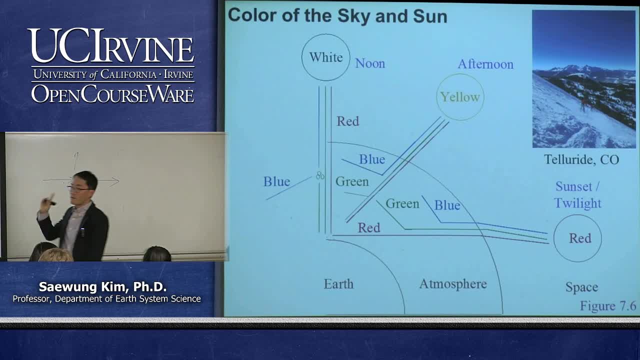 atmosphere. So during the noon it's much shorter wavelengths, so only very, very short wavelengths- visible wavelengths- blue can scatter away, So that's why sky looks blue. And then in the evening time because there's more path length that allow more interaction between visible wavelengths. 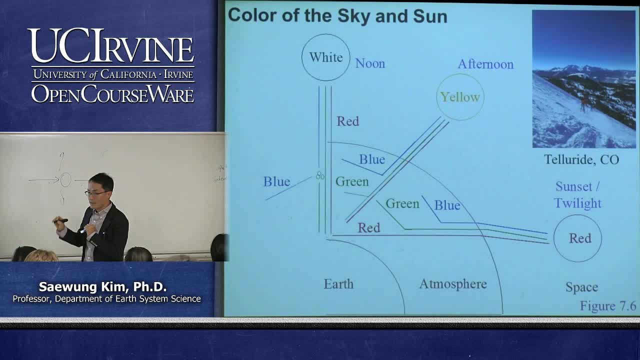 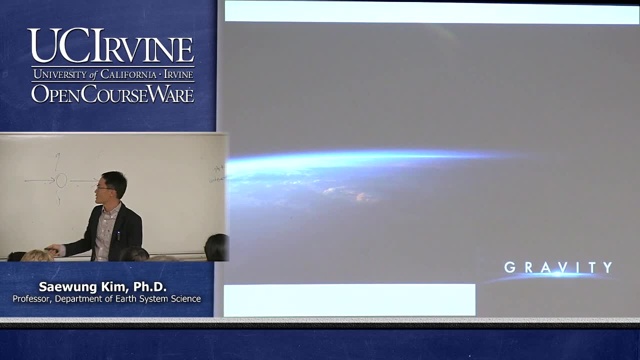 and then gas molecule and then only red can get to our eyes. Okay, So more kind of extreme example of this thing is that if you, how many of you- watched the movie Gravity, So there's couple of actually shot about this atmosphere right here, and then, if you take a look at that, 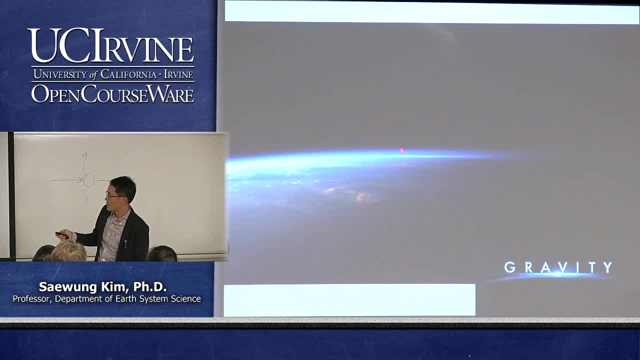 this satellite photo indicated, the blue is actually observed in the top of the atmosphere, So that's due to the scattering. Okay, So a lot of things in this movie is not really scientific. it's over dramatization, I think, but that's factual. 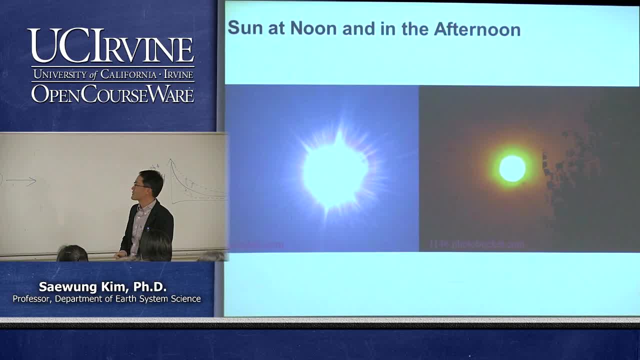 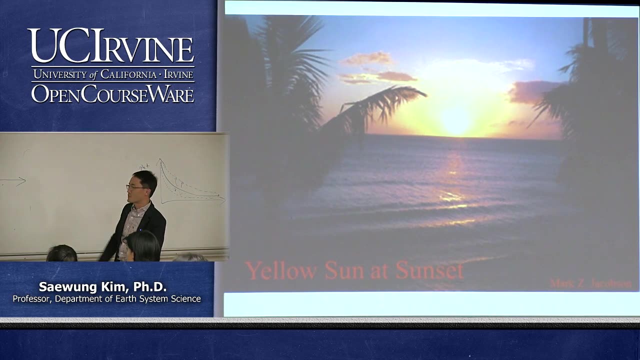 Okay, Looking blue. So that's the photo of the. at noon sun looks white and then in the afternoon looks yellow. we discussed about this thing then yellow sunset. yeah, it's a nice thing. you can just enjoy the nice dinner with your significant others and then 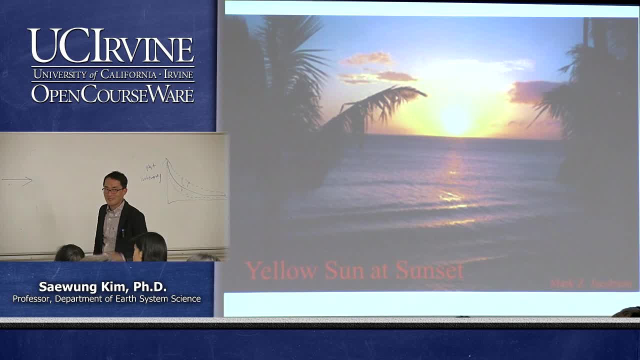 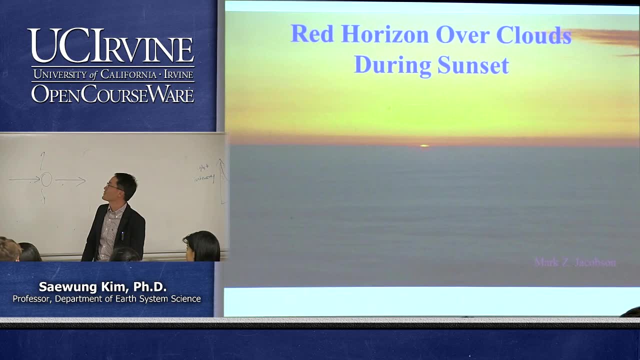 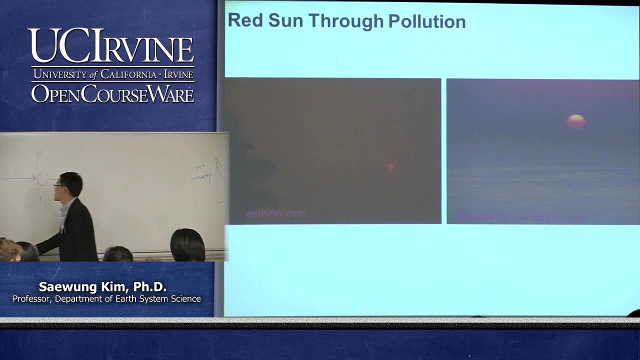 don't describe about scattering things like that while you have dinner. being there wouldn't help. So this is another example of this interaction between atmosphere and then visible wavelengths, and then this is basically this question so far is about natural atmosphere, whether there's pollution or not. 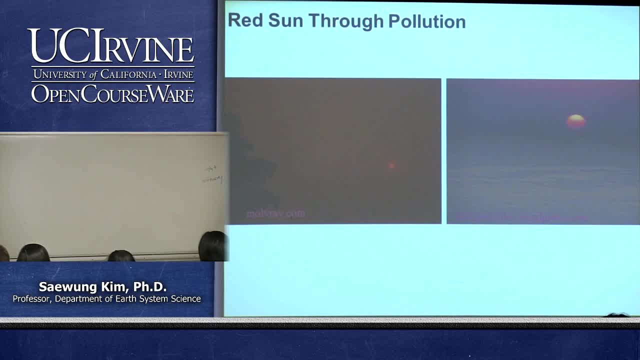 you will see sky blue and then during the sunset that sun is going to be looking like red. but we will talk about how pollution is going to impact solar radiation, especially visible wavelengths region right now. so when we have pollution, actually you can see more like gray kind of thing. 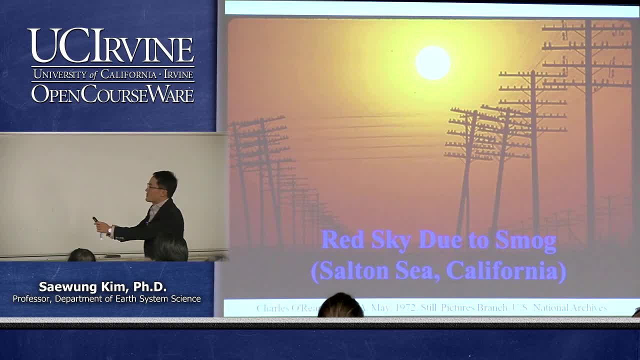 haze layer behind of the sun. so let's discuss about it. This is another example: while there's pollution layer in the atmosphere that always sun looks very different, cause of the interaction between visible wavelengths and the air pollutants, right, So we'll talk about particle absorption. so this is same. 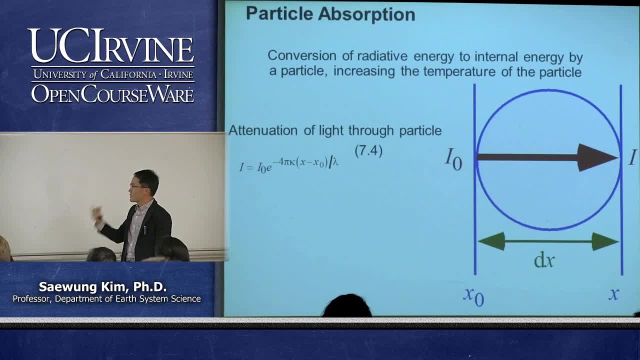 thing. so basically absorption is happening. so this is kind of counter example of the scattering. scattering is about change of the direction of the light propagation, but absorption is more like taking the energy away from the visible wavelengths region and then it will use that energy to bond breaking. 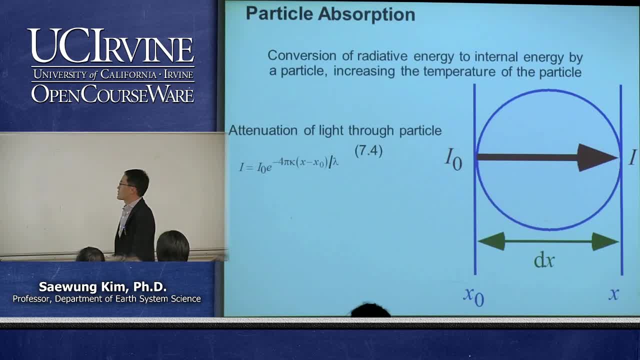 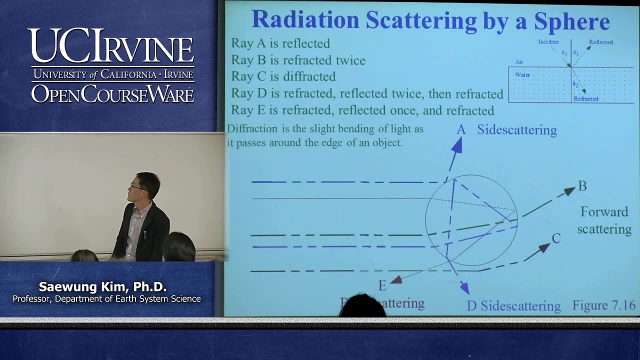 things like that, especially for the visible wavelengths region. okay, So you can. you can use the same analogy, that exponential decay thing, for the gas absorption, for the particle absorption too, so I'm not going to discuss about this thing here. and then particle scattering, so for the gas. 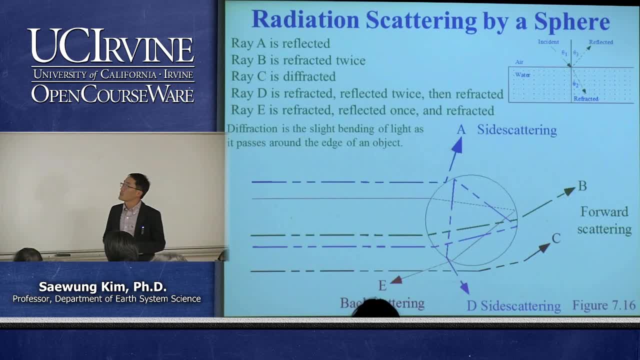 molecule scattering- we talked about Rayleigh scattering. so for the particle scattering, we call it Mies scattering, but we are not going to deeply discuss about that specific term. but we'll discuss about different interaction in terms of scattering between the particle and then visible wavelengths region. so scattering we talked about. 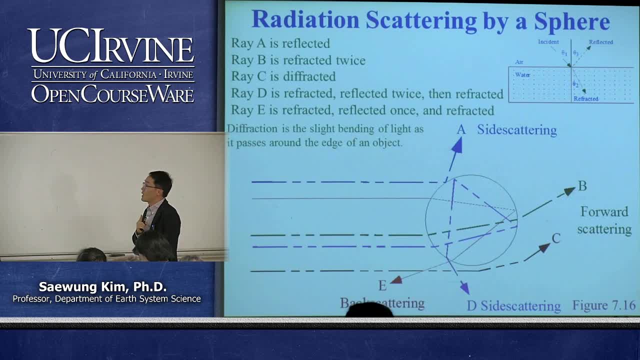 that's the direction change in terms of the radiation. so one of the thing that when we- I don't know if you took the physics class in high school- there's always some discussion about how light is propagating in the air. so light is coming to the surface of. 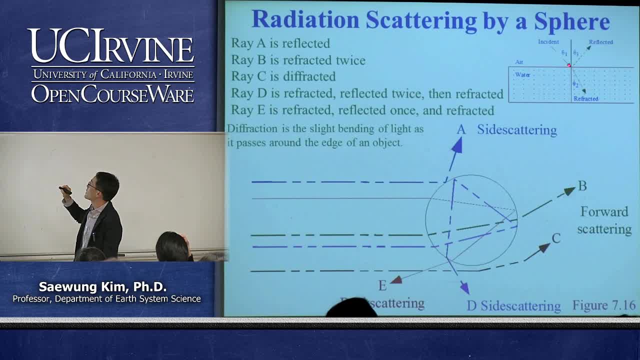 water through the air, then some of the light is going to be reflected away and most of the cases the angle is same. right, theta one and theta three is same. now some of the light is actually getting into the water. through the different medium change the angle of the propagation. 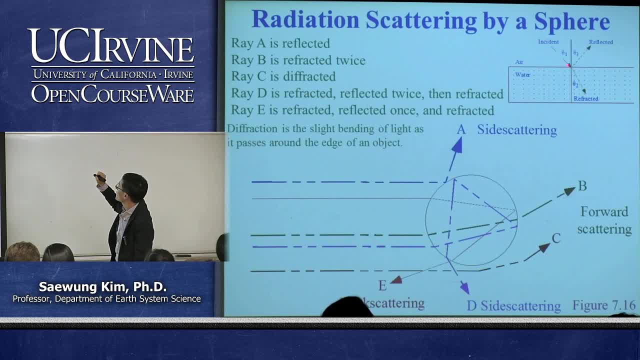 so we call it this kind of propagating some of the light into the different medium. we call it refraction, right? so this is reflection and this is refraction. then the other thing is diffraction, so that's actually C right here. basically, diffraction is is the slight bending of the light. 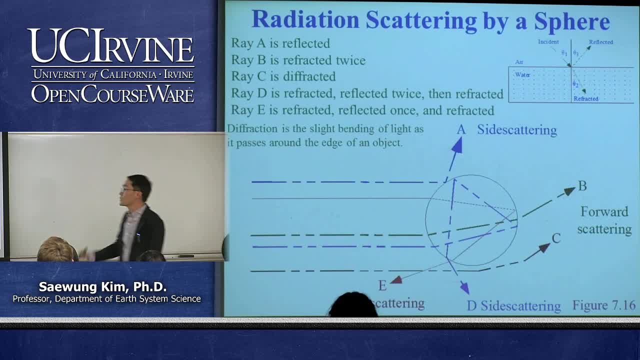 as it passes around the edge of an object. so it is. if you take follow this arrow, this light is not actually touching this particle, but the direction is slightly changing at the edge of the particle. so this is, by definition, diffraction. okay, so let's take a look at here. 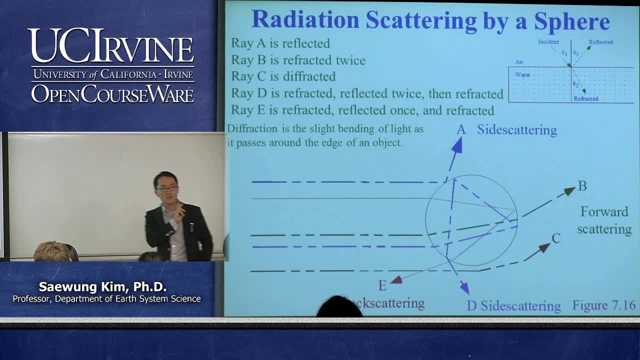 so that's the kind of characteristic of interaction between radiation and particle, right so? but if we define just based on the direction, there's three kind of the scattering between radiation, visible wavelength radiation and particle. one is side scattering, basically light is coming to the particle and then it 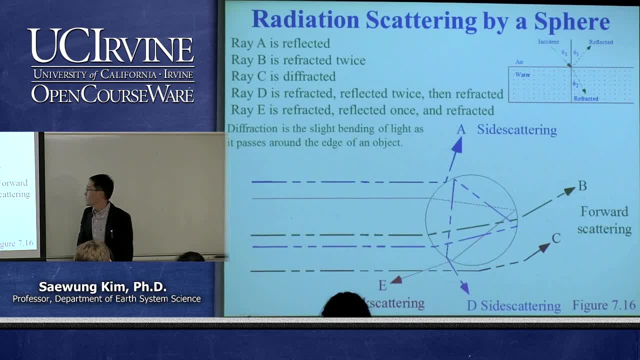 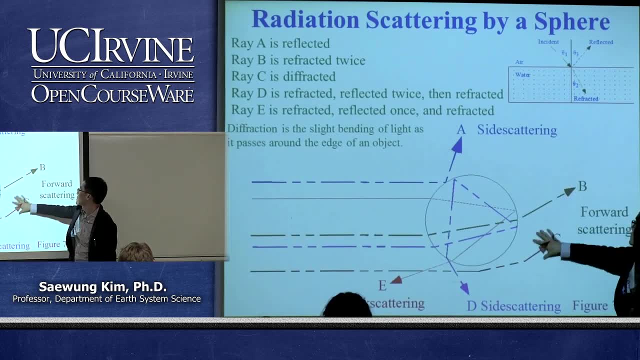 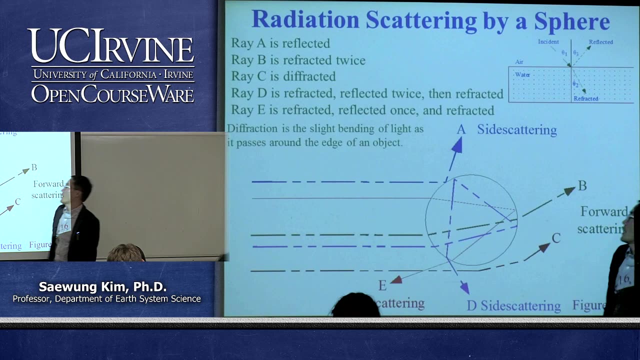 scatters to the side of the particle right and then forward scattering, although it is kind of deflected a little bit. still, the light is coming to the same direction, to the forward side right, and then back scattering. is that light is coming back right from the instant angle right here? 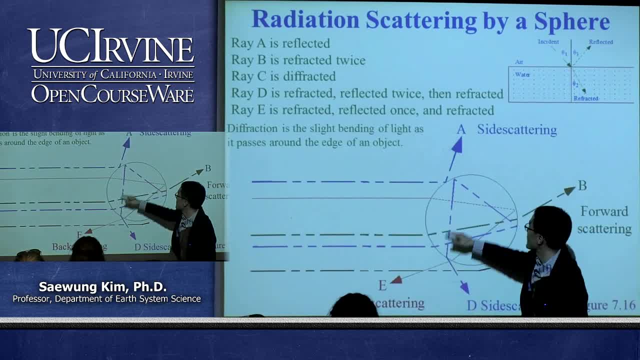 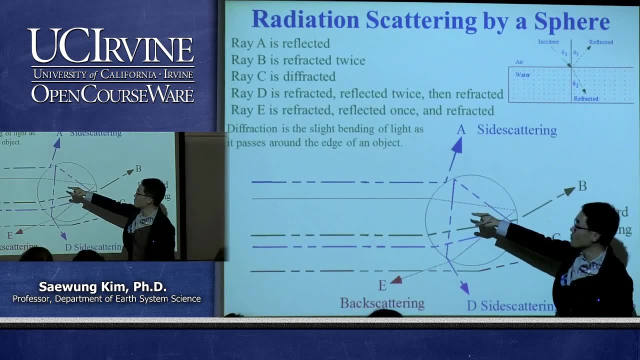 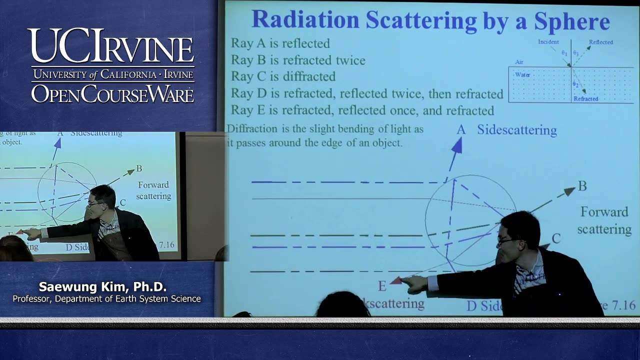 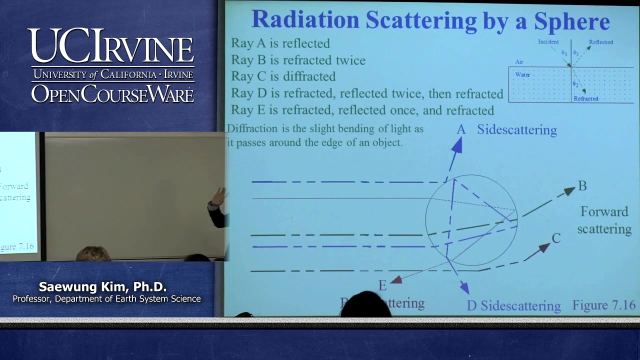 so light used to be coming back, and then it's getting into outer medium. so this is, by definition, diffraction. right out here, this thing get deflected and then deflected again, and then it makes the back scattering right. so this slide contains a lot of information about that. 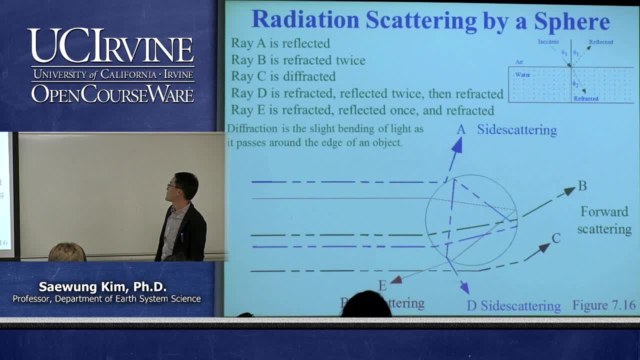 all sort of interaction between light and particle: reflection, diffraction and things like that. it's kind of funny thing that when I first got in this country, so in my mother tongue, in Korean, there's no actually difference between L and R sound. we cannot tell the difference at all. 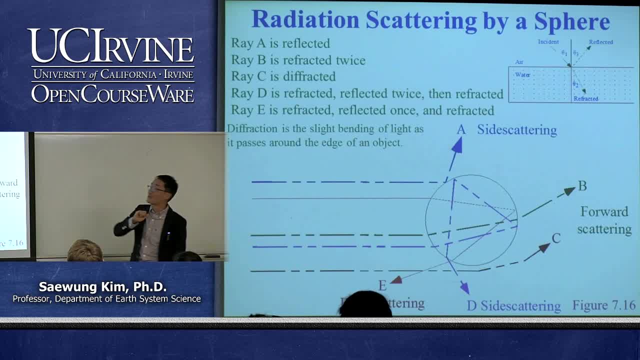 between L and R, and then it was very challenging for me to differentiate the L and R sound. somehow the English stickers really good at differentiating L and R sound, so it used to be very challenging to tell the difference between reflection and diffraction. so anyway, just a side story. 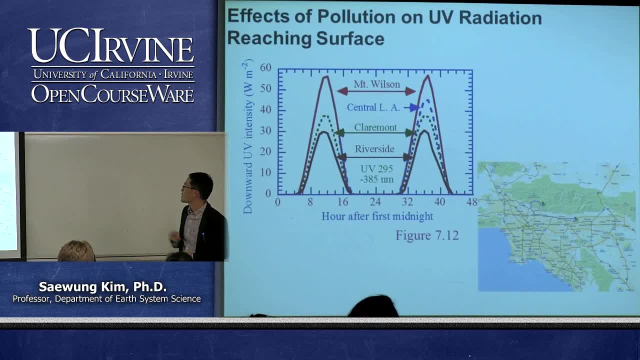 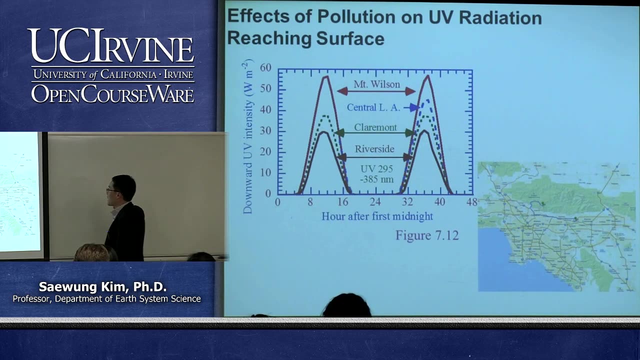 so what is this slide is about? I got carried away. so this is okay, this is effect of pollution, and then how the pollution layer is going to be affecting on the radiation actually on the surface. okay, so this is actual observation, okay, from Mount Wilson, which is right here. 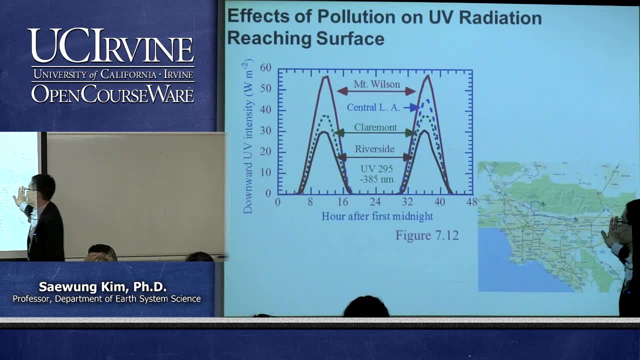 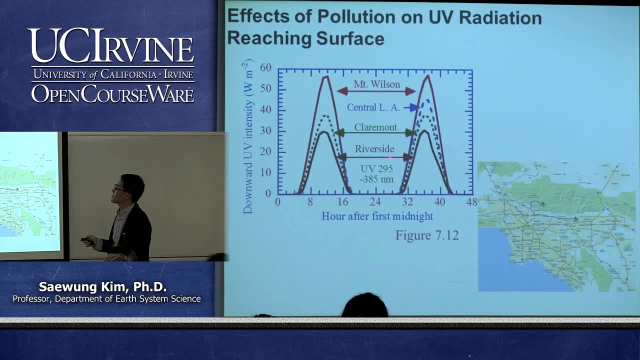 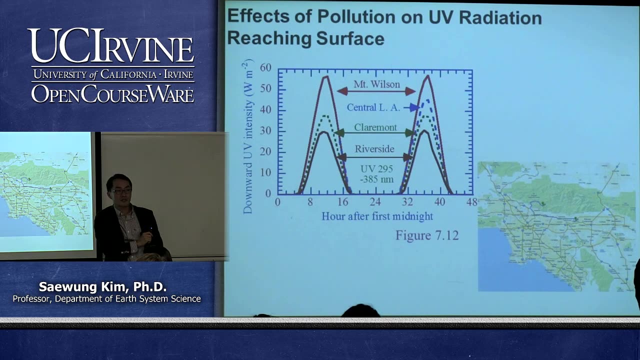 higher altitude. so you can imagine all those pollution are sitting in this Los Angeles basin right and then Claremont and then central Los Angeles and riverside. so basically, this decrease of the UV intensity. UV is from where? from the sun, from the sky. so this decrease of UV intensity 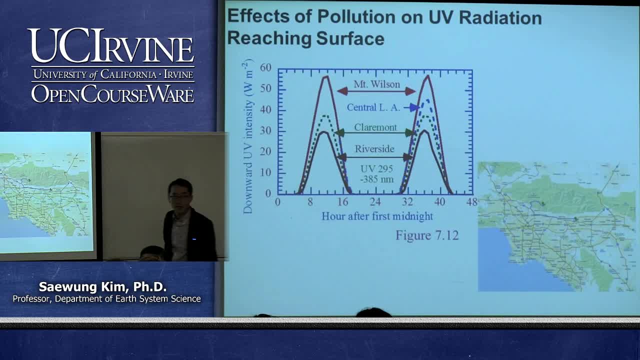 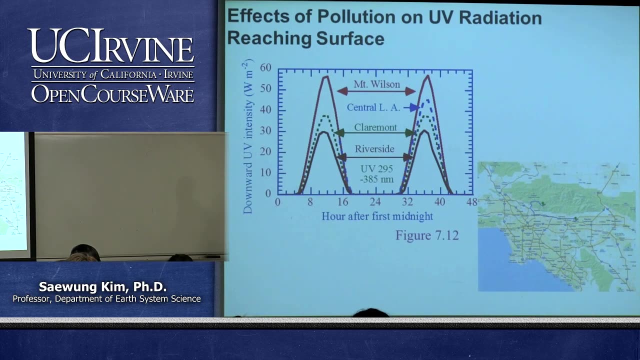 basically you can pinpoint out where exactly that pollution layer is. then this much of the solar radiation actually got absorbed by the pollution layer. then pollution we actually there was on the what's the air pollution definition. it is both gas and particle. alright, so gas and particle interact with the 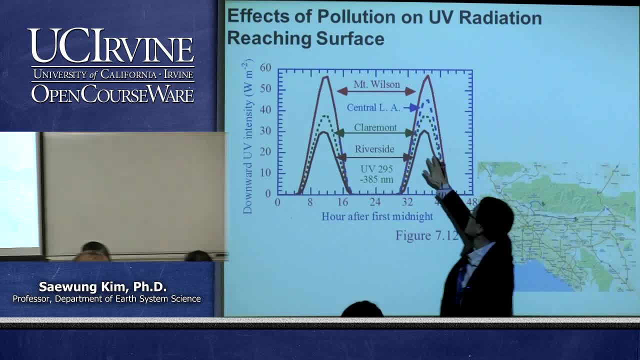 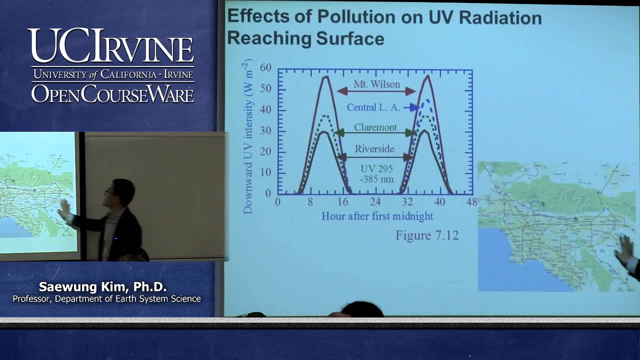 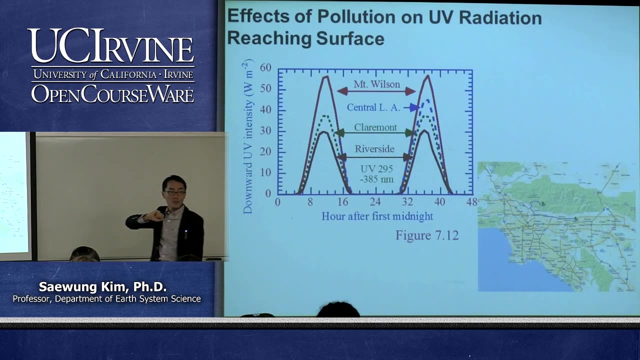 solar radiation and then there's less energy actually gets into the surface of the atom's surface that we leave, because that pollution layer absorb and scatter the energy from the sun. okay, so that's what this plot is all about. so let's take a look at little more. 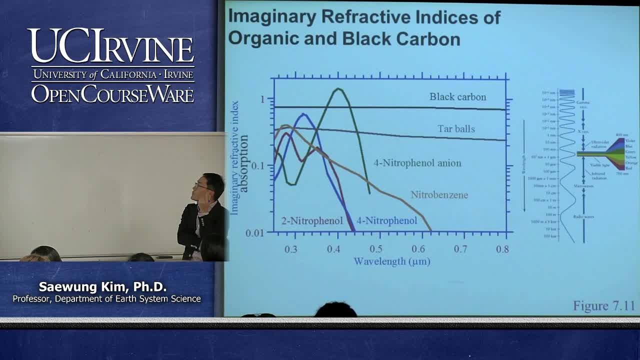 on how different aerosol particles interact with the different visible wavelengths region. okay, so black carbon. so why some particle looks black like soot? because all the visible wavelengths is absorbed, absorbed by that specific particle. that's why it looks black, right. so by the so this by definition, absorbing. 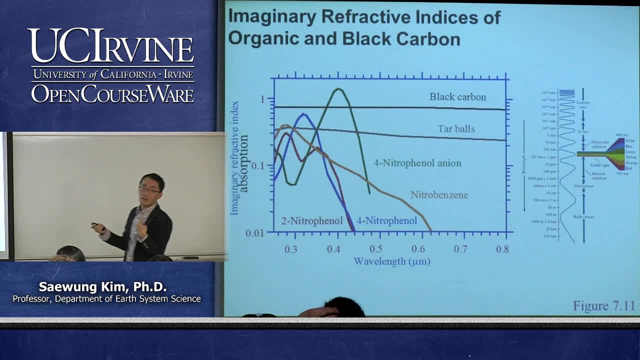 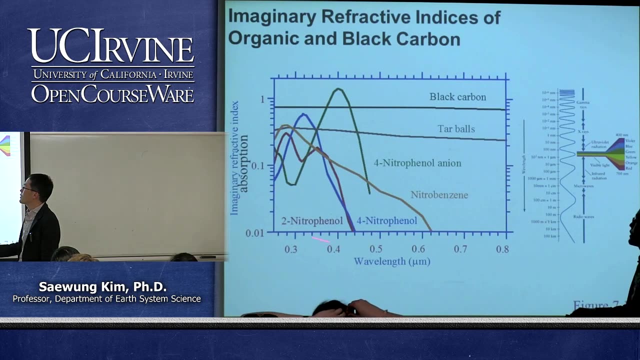 all the solar, the visible wavelengths by the particle, so that's why it looks black and then different chemical composition actually ended up making different color. that means this different chemical composition of the aerosol, observing selectively some wavelength region, kind of the region behind of the selective absorption. 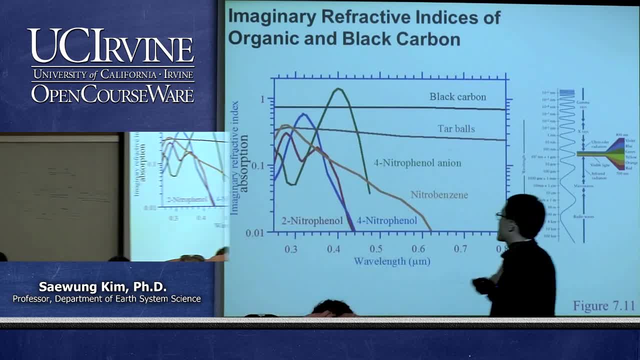 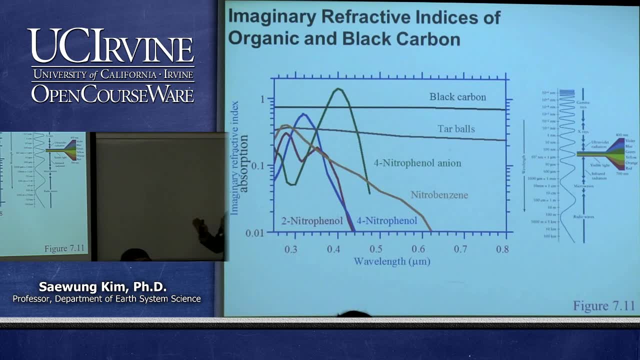 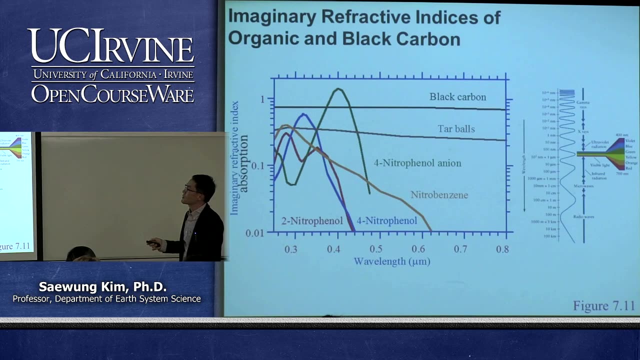 is just like that. so some of the chemical prefer to absorb some of the different wavelength region that may that can cause some sort of this kind of chemical reaction. okay, that's why different chemical species observe different wavelength region. that makes different colors of the atmosphere particle okay. 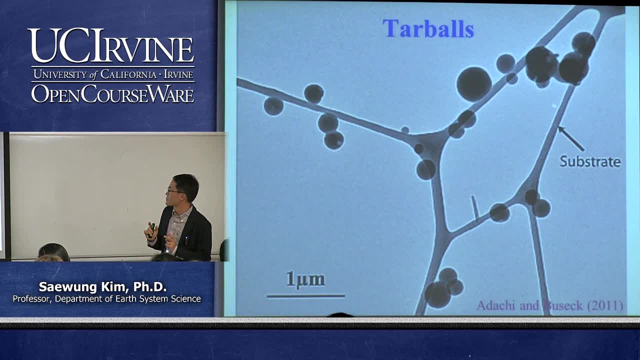 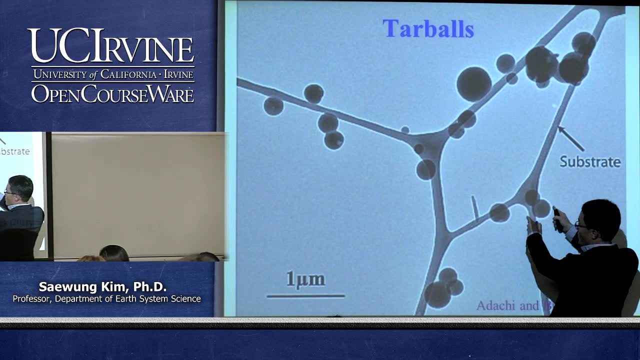 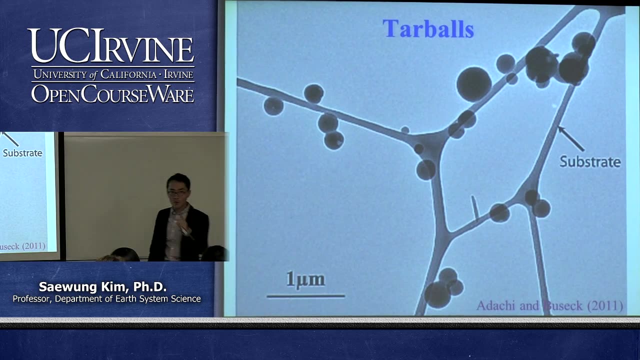 so this is the actual kind of microscopic view of a table. so that's basically one micrometer. so that's about one micrometer. so that's by definition. is that by definition of what PM 2.5 right? PM 2.5 is particle size below. 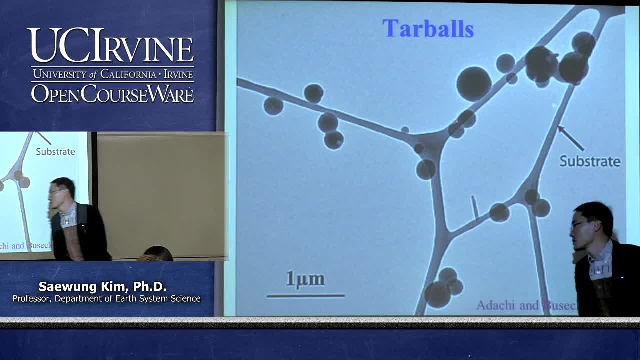 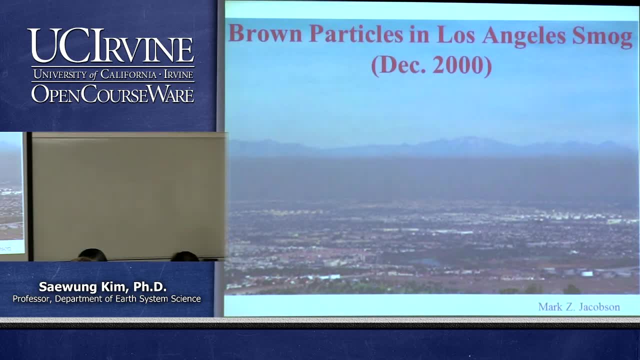 2.5 micrometer and then, as you can see, this table is smaller than one micrometer. so that's, each table is going to be PM 2.5. okay, so we talked about this brown color. some of this brown color is absorption of NO2. 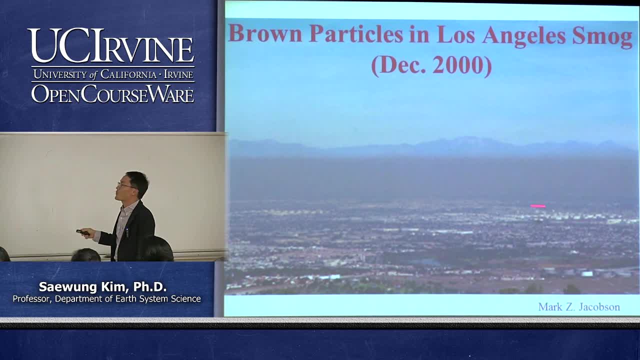 which is coming from the core, but this kind of dense brown thing is actually due to absorption by particle. okay, that's why this looks this dense brown. so let's take a look at the implication of that, this very brown looking particle in the atmosphere. so so your beautiful. 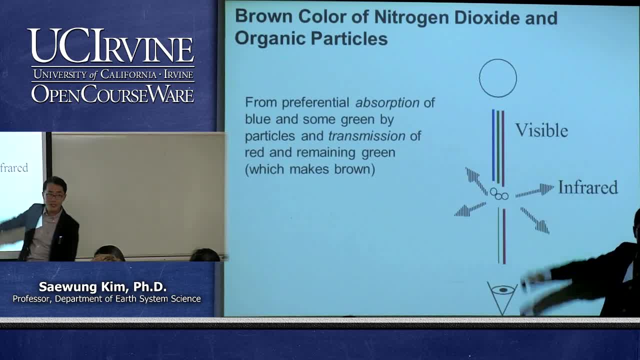 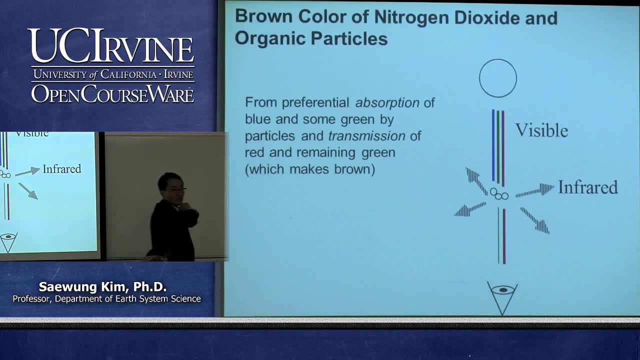 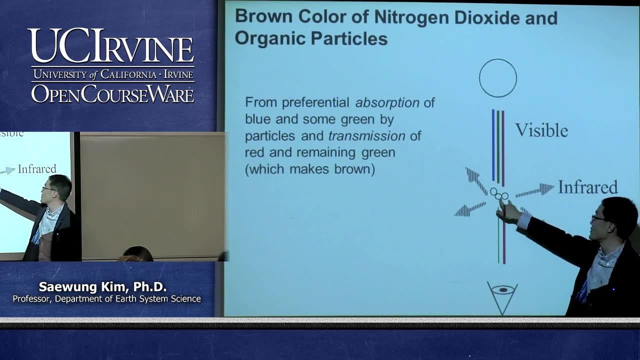 eyes here and sun is there right, and then this looks brown. why that looks brown? because it's absorbing the wavelength region of the blue and then a little bit of green, right, it's absorbing right here. so basically, this particle absorbs UV wavelength region, not UV. so below the 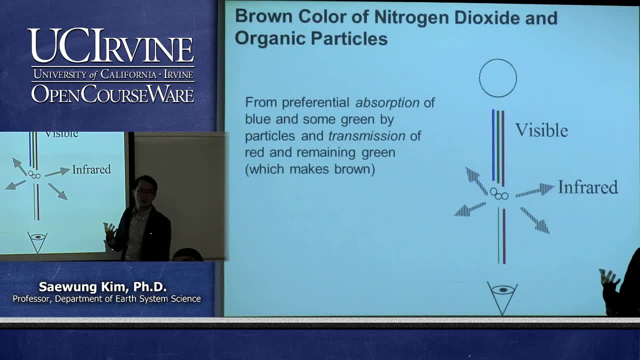 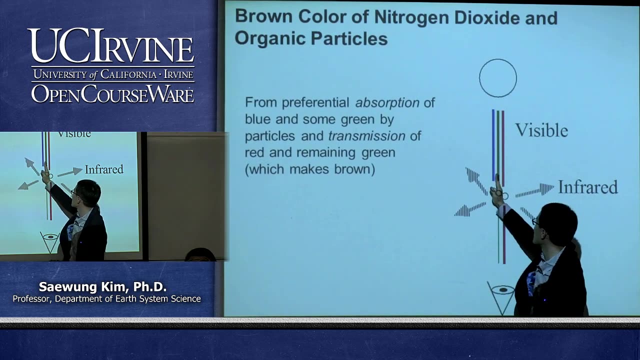 green wavelength region, probably about four. so we so one of the question about the asking about green color laser pointer is 530 something nanometer, right? so below 530 nanometer this brown looking particle is going to be absorbing the energy, right? so if you remember, definition of a black body radiation. 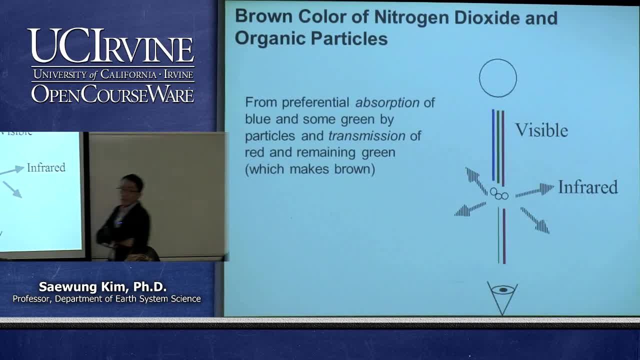 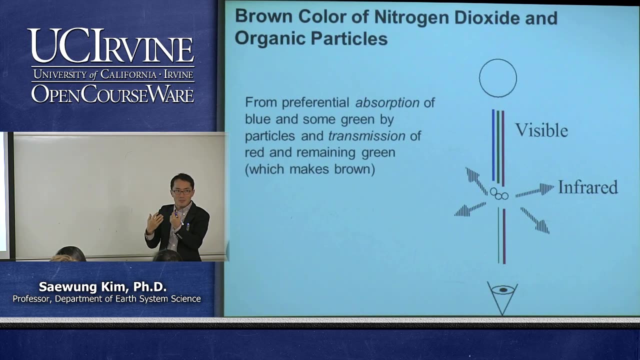 this guy absorbs some of the energy from solar radiation, then what that thing is going to be doing in the atmosphere- it's absorbing some energy- then what it's going to be doing, it's going to be saving the energy in its body. that's not the nature saving. 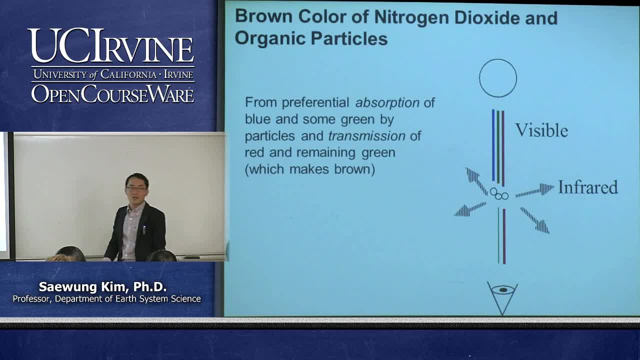 is not the nature. it's going to be emitting direct, right away. okay, observe some energy, then it's going to be emitting energy. then what would be the energy form that this particle is going to be emitting? so it is absorbing visible wavelength region. what kind of energy? UV. 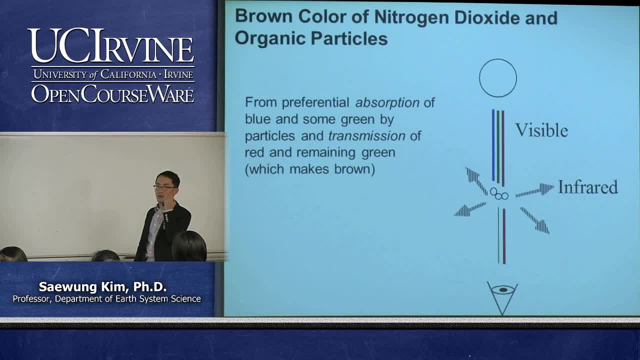 or visible or IR. so what determines the? what determines the characteristic of the electromagnetic radiation temperature? sun is very high temperature, so it is emitting higher energy wavelength, which is visible, right. what's the temperature of this thing? it's going to be atmospheric temperature, which is very close to earth. 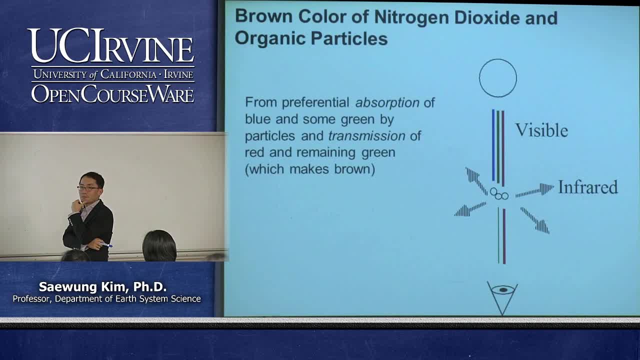 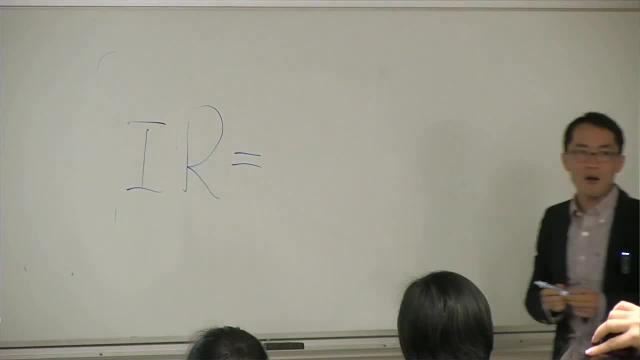 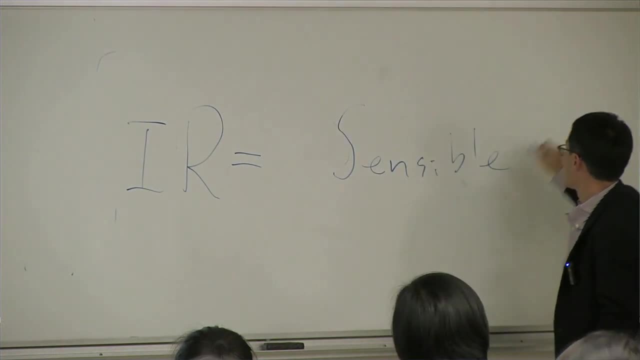 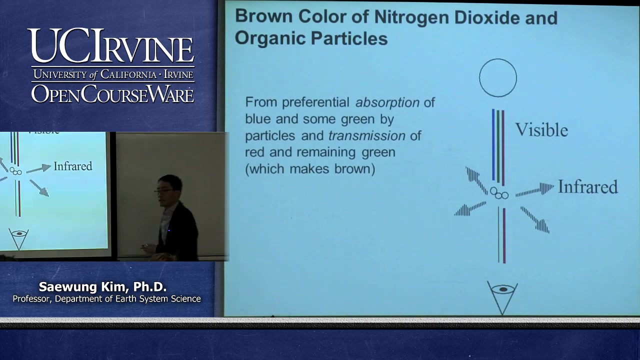 temperature. so what's the earth is emitting, what's the nickname of the IR infrared? yeah, so basically what this brown particle is going to be doing in the atmosphere: it's absorbing visible wavelength region with sense as a light, and then it's going to be emitting heat to the 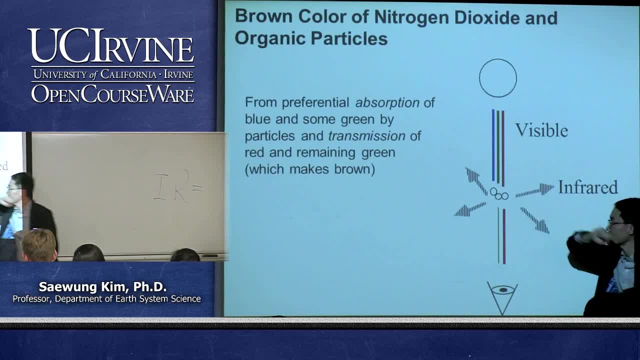 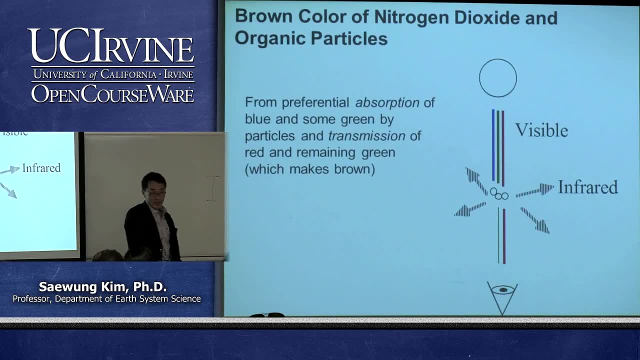 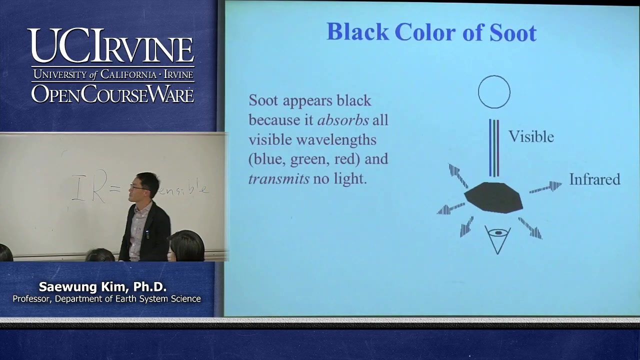 atmosphere, right. so basically, this brown looking particle is going to heat it up. atmosphere right, okay, clear, it's very important, alright, so even worse that black color. so so why this soot looks black? yeah, observing everything, right, all the energy from the sun. so it's going to. 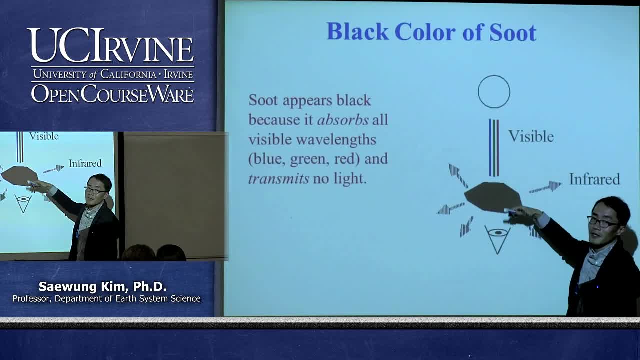 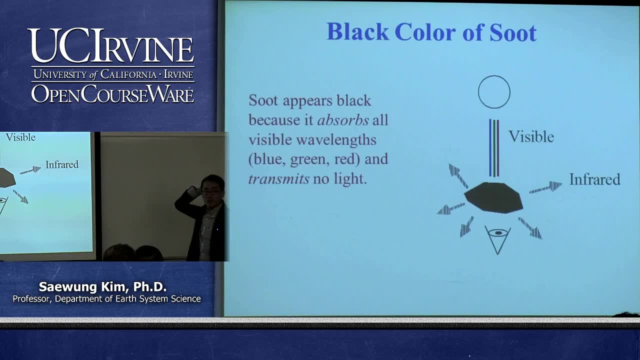 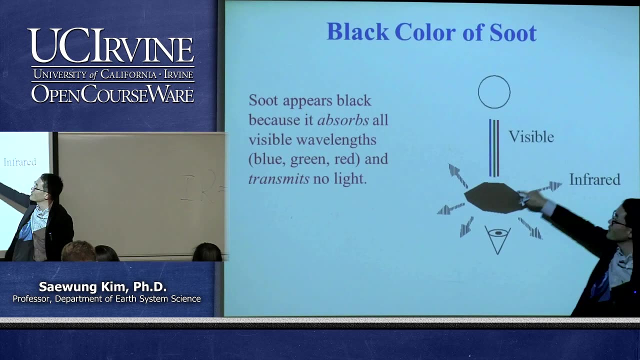 be observing all the energy from the sun, the visible wavelength then, by definition, of black body radiation. it's going to be emitting everything again to the atmosphere in forms of what sensible heat. so it's going to be warming up more the atmosphere, right? so that's why. 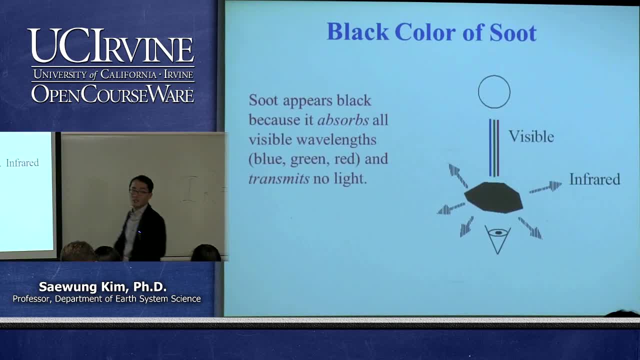 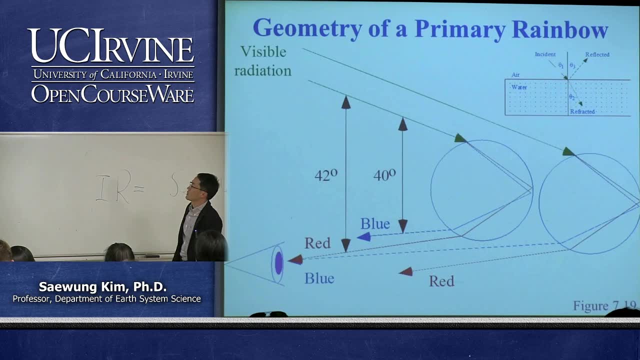 we're worrying about this black carbon that's going to heat it up the atmosphere, right, it's going to be accelerate global warming, okay, so we talked about very scary thing about the particle. let's talk about some beautiful thing that particle is doing in the atmosphere: making rainbow, right. 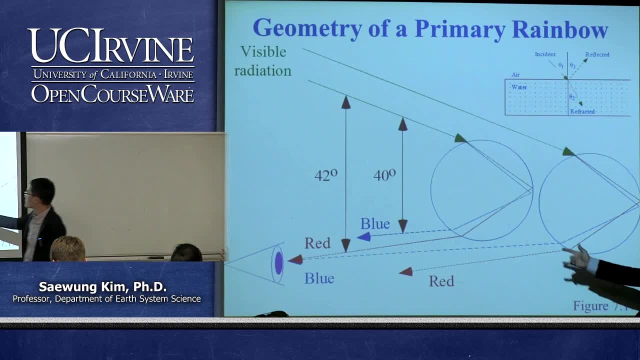 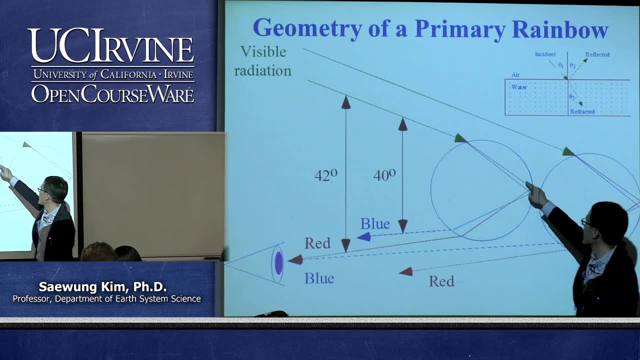 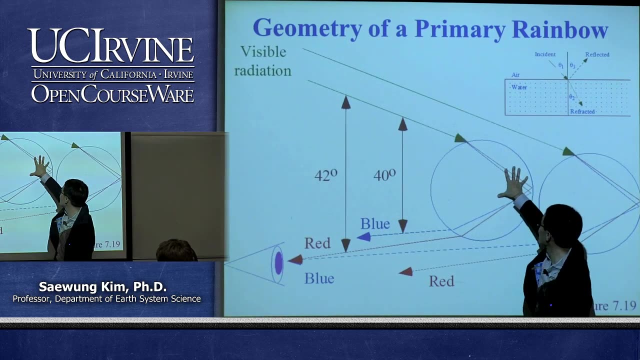 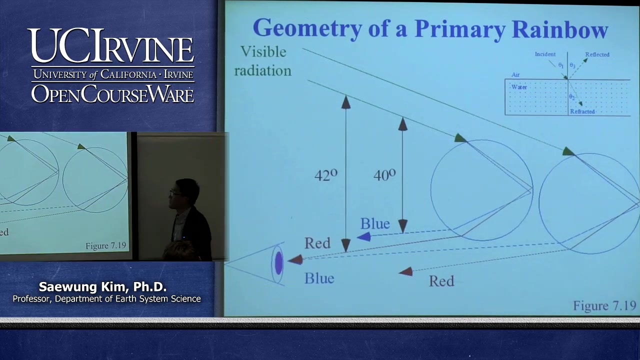 so rainbow basically is based on the different reflection angle, diffraction angle, rather of the different wavelength region: right, so red is have, so basically blue has sharper angle than the red. so basically this water drumlet can separate that different wavelength region of the of the visible so that we can see the rainbow. 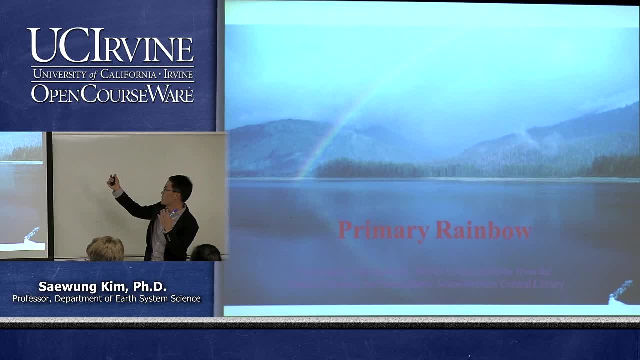 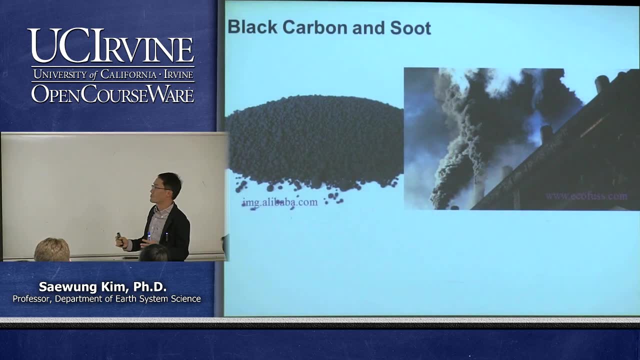 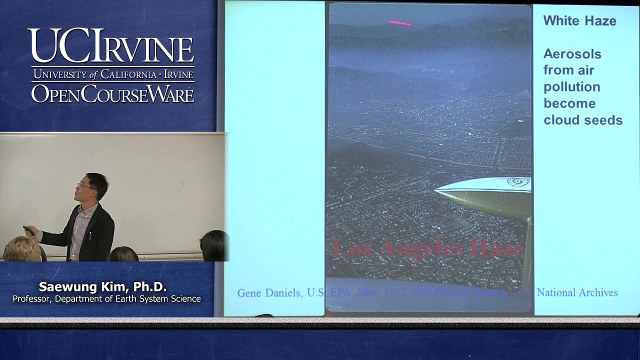 okay, so that's the beautiful side of the interaction between light and the particle. and then this black carbon from the pollution is kind of a dark side of the interaction between visible wavelength region and particle in the atmosphere, right, so if it is white looking one, actually, this is actually. 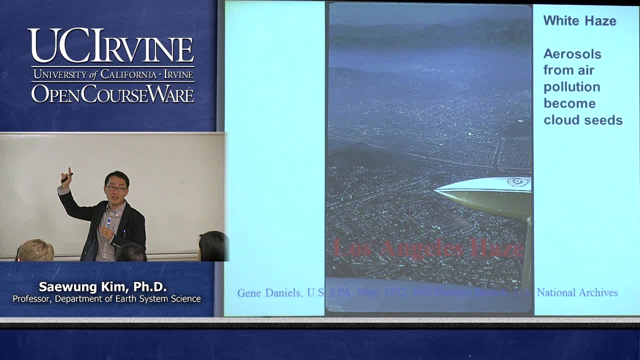 cooling the atmosphere, because it's basically reflecting the solar radiation away from the atmosphere. so that's white haze, and then this white haze, usually from the sulfuric acid, H2SO4, makes, yeah, this white haze. so it depends on the color that actually the particle in the atmosphere. 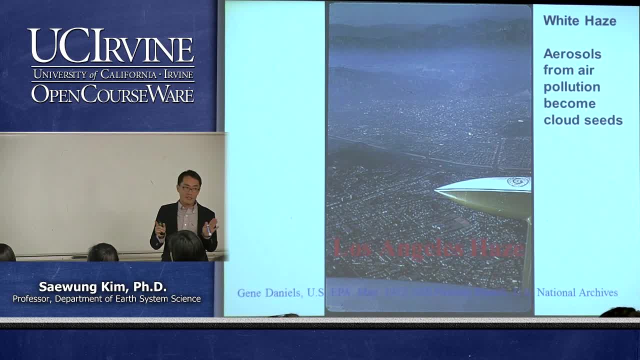 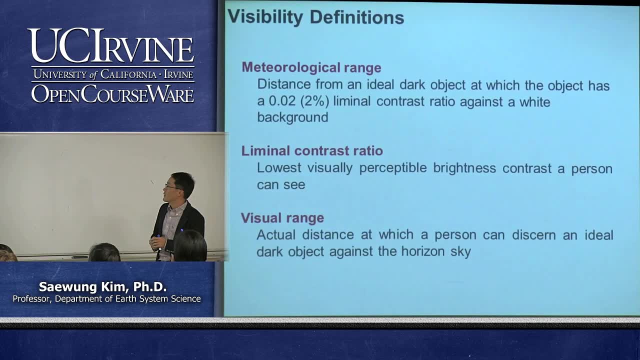 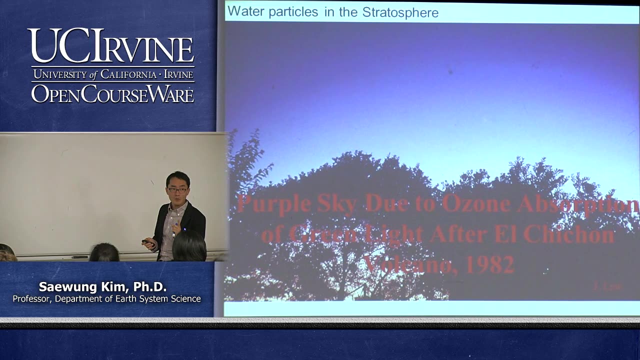 can heat it up the atmosphere or cooling down the atmosphere, right, so hazing for Los Angeles and then we will just get down to visibility. so sometimes, actually, one of the question of the quiz is about the volcano particle. so basically, sometimes you can see the volcano particle when it is very 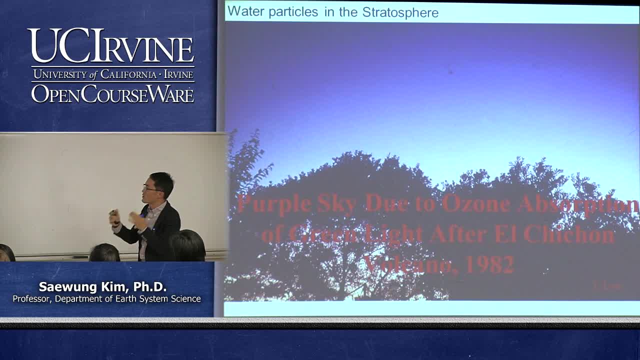 it's a large number of particle actually gets into the stratosphere. so this is 1982, that's a big volcano actually erupted in, I think, Chile, and then that's erupted a lot of gas particle- not gas particle, particle particle, so particle to the stratosphere. 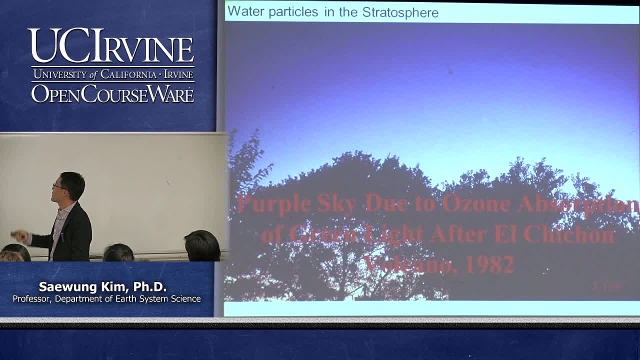 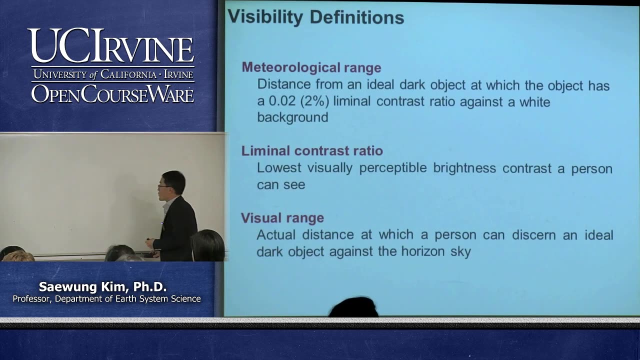 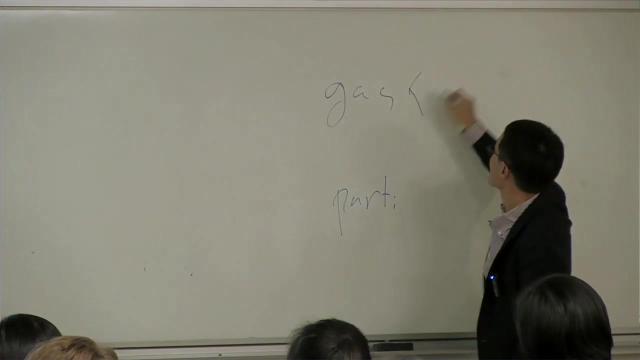 and then that make looks sky white because of the sulfuric acid gets into the stratosphere. then that cause this white color in the stratosphere. so we are talking a lot about this visibility. so we talked about gas and particle and then absorption and scattering. 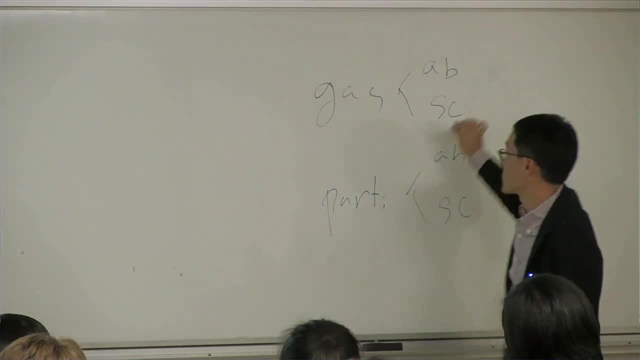 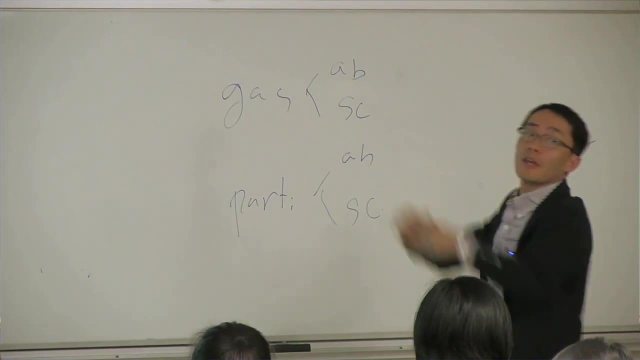 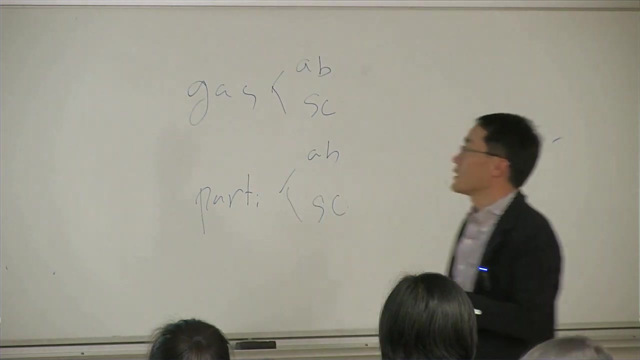 and absorption and scattering the inaction. there's four different: inaction between gas and particle, and then if you add these things, and then that will affect the visibility. so definition of visibility is basically how far we can see in the stratosphere, right? so this is. 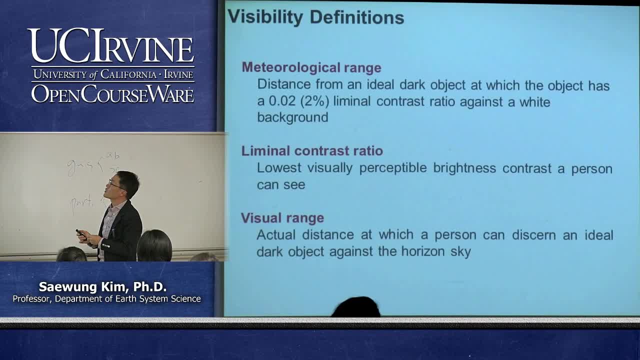 very confusing concept. but basically the definition of meteorological range, meteorological visibility, is that the distance we can identify, about 2% of liminal contrast, and then definition of liminal contrast is even more confusing. so basically, the people can identify, so I don't know if it's really. 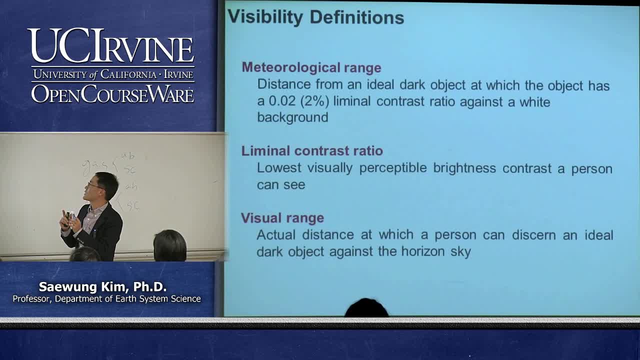 scientific or not, but the way I can kind of grasp the concept of this thing is that maybe 100 people out of 2 can see that far is about 2% of the contrast. that's how I remember it, but that's not really important. so that's basically what. 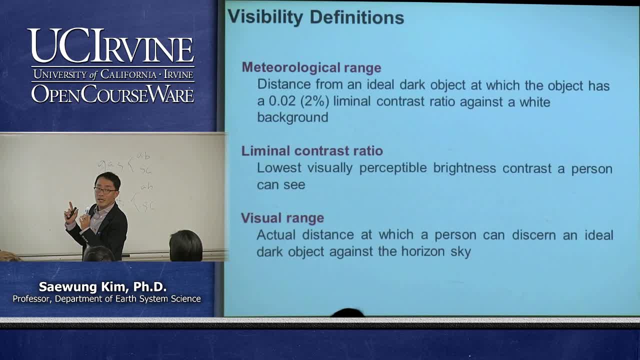 I'm trying to say in this slide is that basically visibility is how much we can see, and then there's some definition. that's why if you go to the airport website, actually airport website, actually publish the visibility range: 10km, 20km hourly visibility. 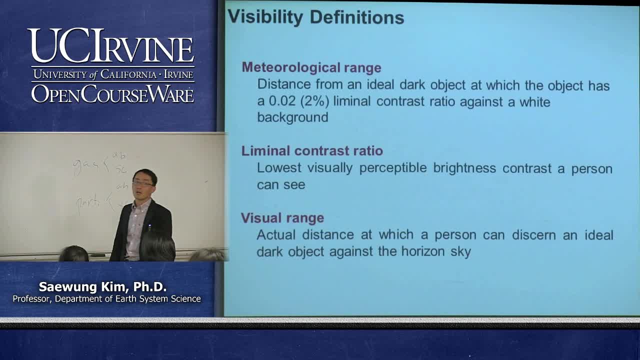 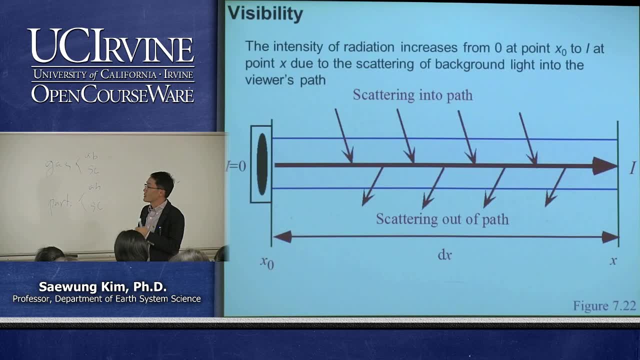 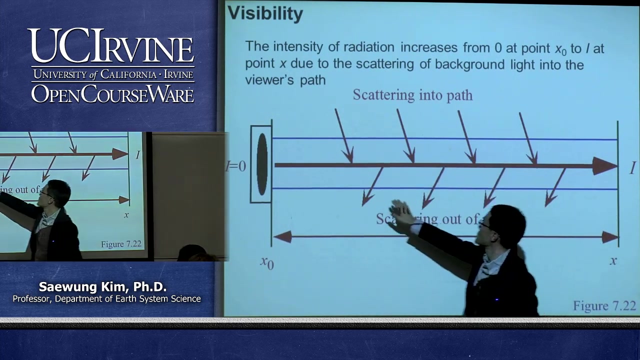 range. and then these are the definition of that determining the visibility when you listen to weather forecast, things like that. so again, so visibility is kind of a imagine, this kind of light path for the atmosphere. so, although this is just shaded as red, so basically in this column: 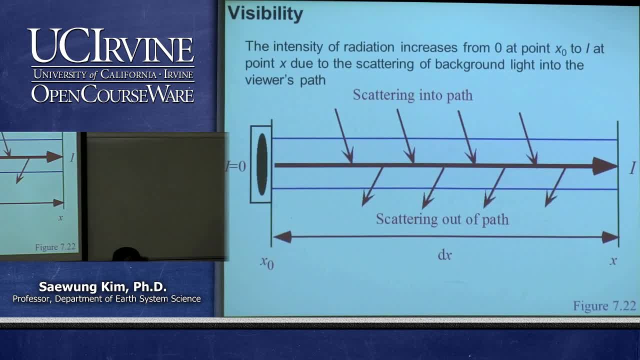 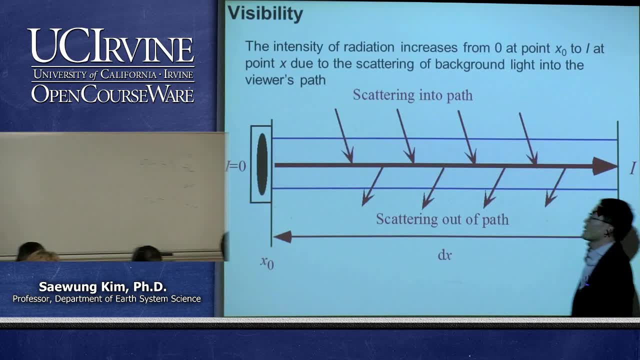 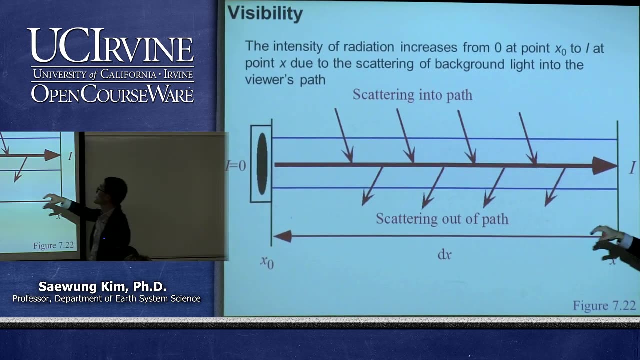 there's an interaction going on between gas and particle and then specific physical mechanism is absorption and scattering and then there's less light is coming from here to here. so if there's some more interaction going on, then you will get the less visible wavelengths here, then you will get the less visibility. 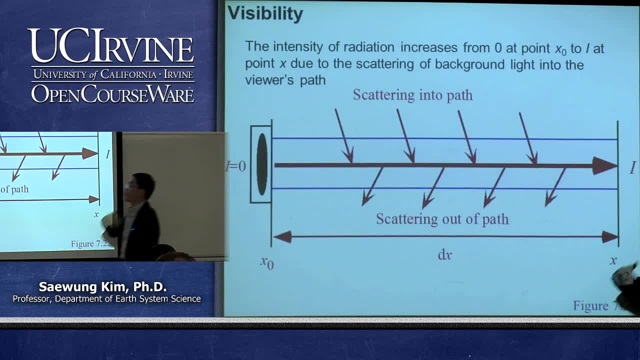 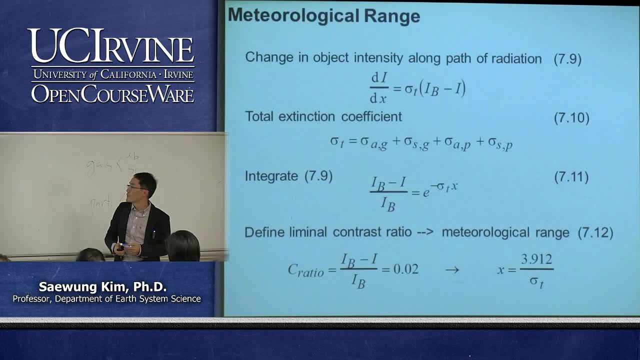 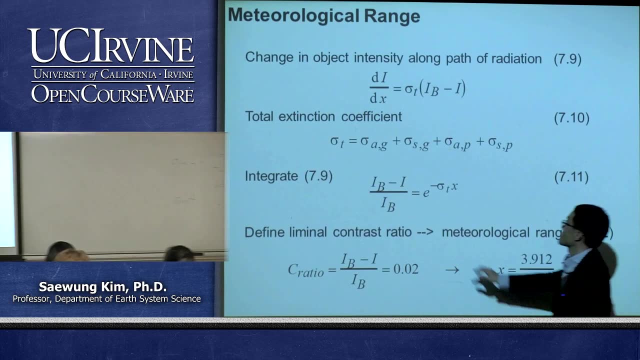 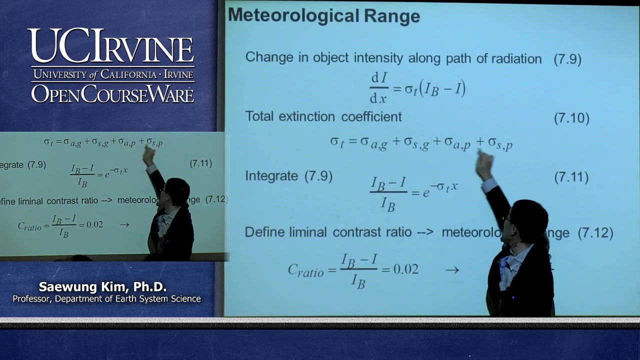 then if there's more visible radiation is traveling, then you will have better visibility, right, that's the by definition. so if you express this thing, if you are mathematically oriented person, again you can put this separate parameter which is gas absorption, gas scattering, particle absorption and particle scattering. 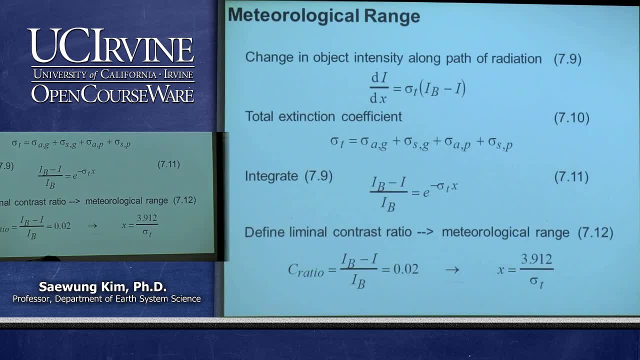 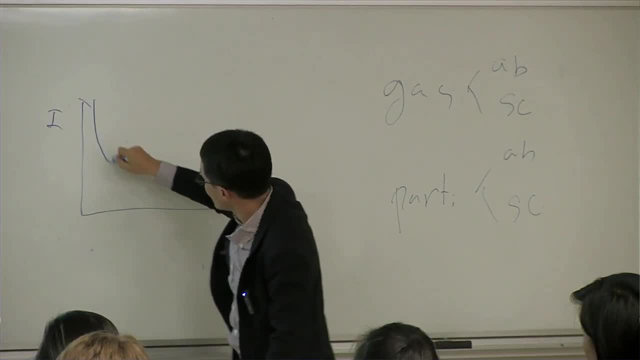 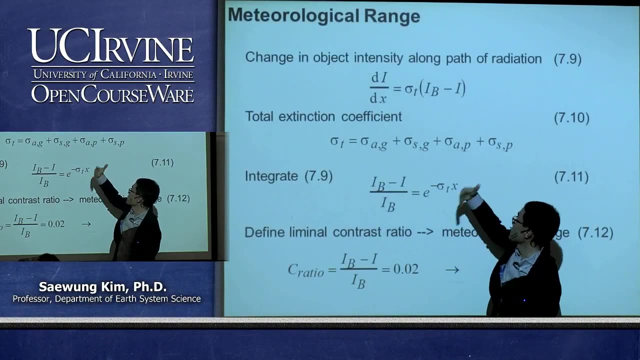 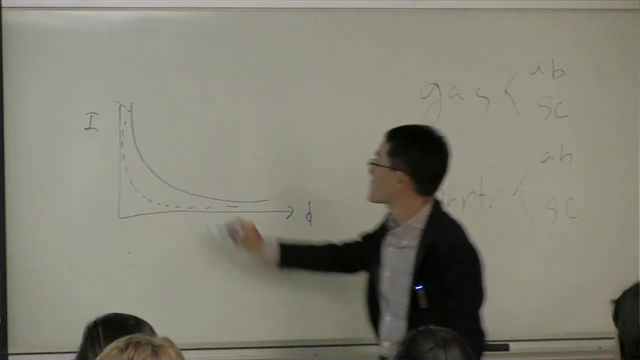 again. so this is exponential decay. we talked about exponential decay which is distance and then light. it's gonna be decreasing like that, and then if you have larger absorption or larger scattering, both gas and particle, you will get the fast extinction of the light. so that's by definition. 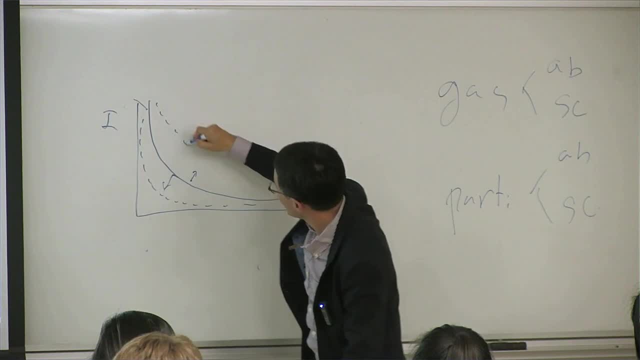 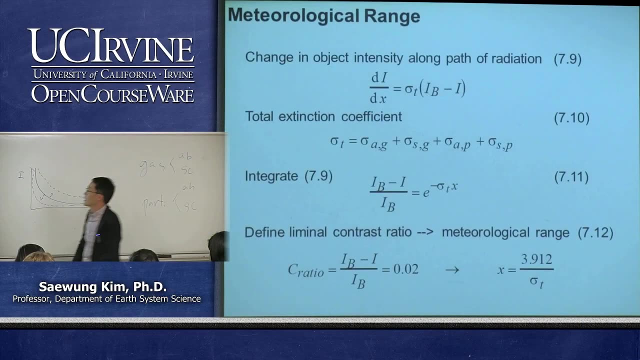 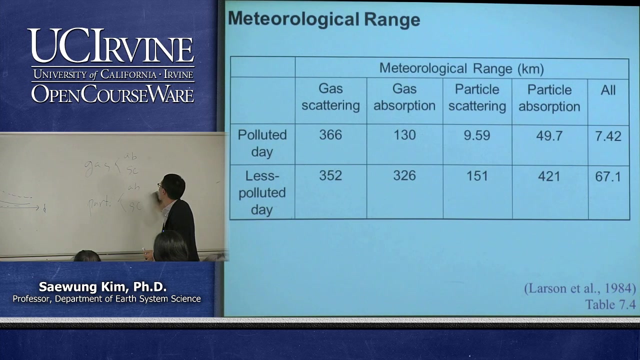 bad visibility and then clean air, you will get the slower extinction. so this means the better visibility, right? so that's actually. I love this way to express this visibility as a science geek, but you may have different idea, so I prepare another slide right here. so this is real world example. 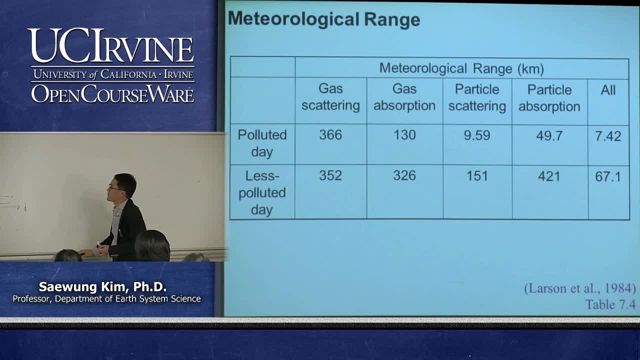 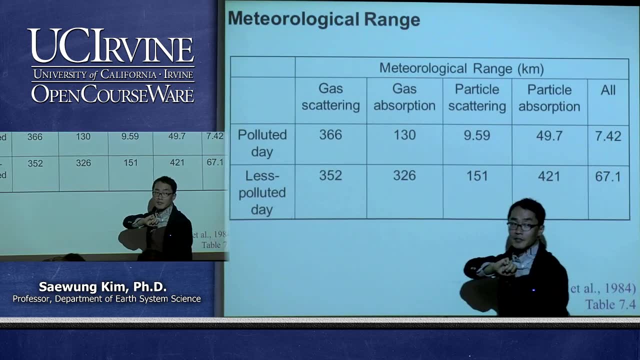 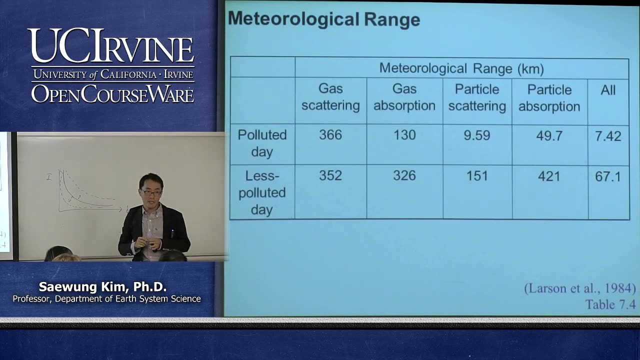 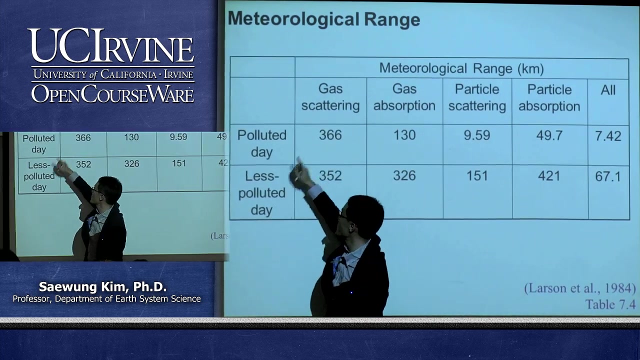 so basically, this number right here means that if there's only gas scattering in the atmosphere, basically you will be able to see 366 km away from here, right so, which is pretty far, and then this is polluted scenario, polluted atmosphere. this is not polluted atmosphere, so gas. 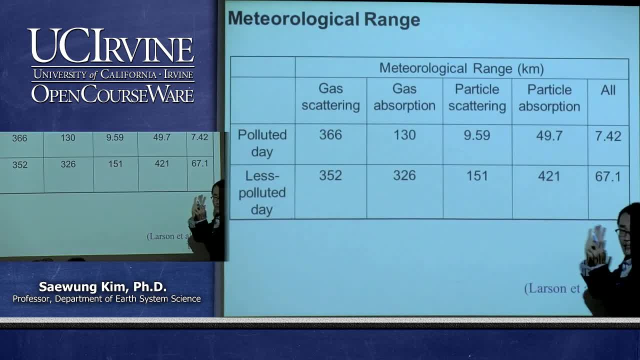 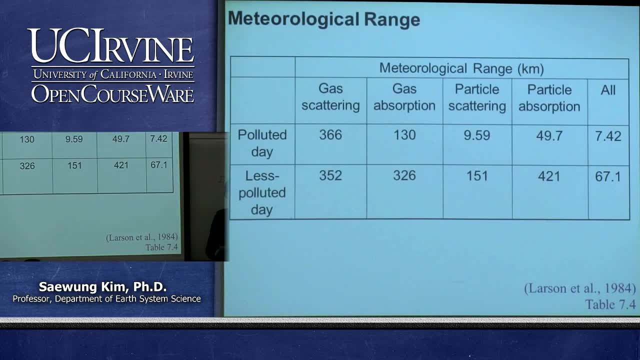 this is gas scattering and the gas absorption. if there's only gas absorption is happening in the atmosphere, then you will be able to see 130 km in polluted day and then you will be able to see 326 km. right, so you can take a look at the particle. 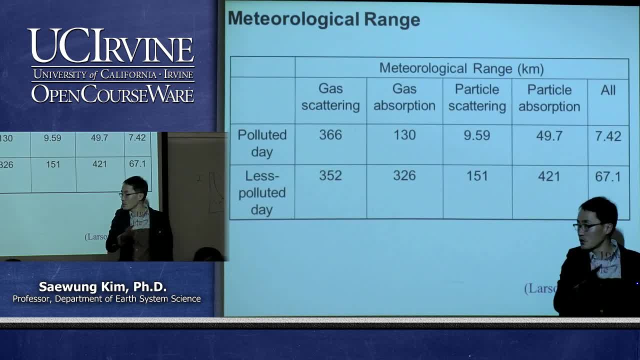 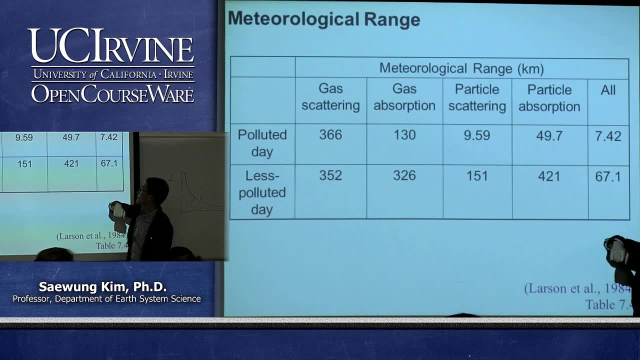 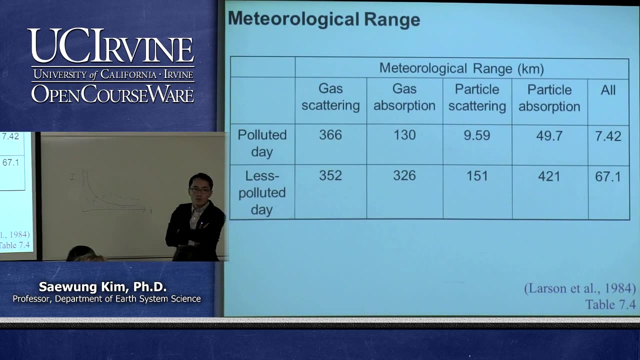 scattering, so only there's particle scattering in the atmosphere. then you will see about 10 km and 151 and the particle absorption is about 49 and then, when not polluted day, about 421. so which one is most important factor to determine the visibility in the 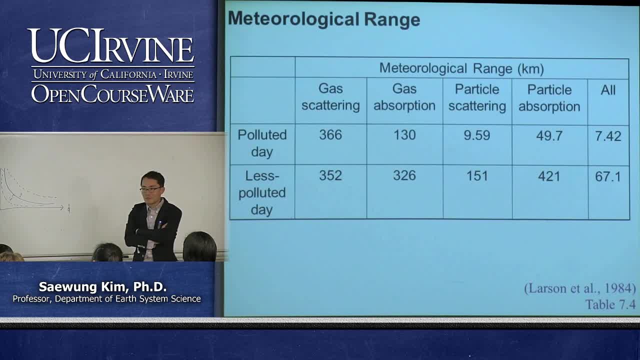 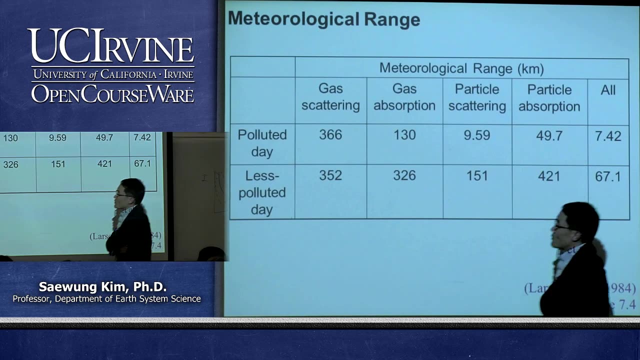 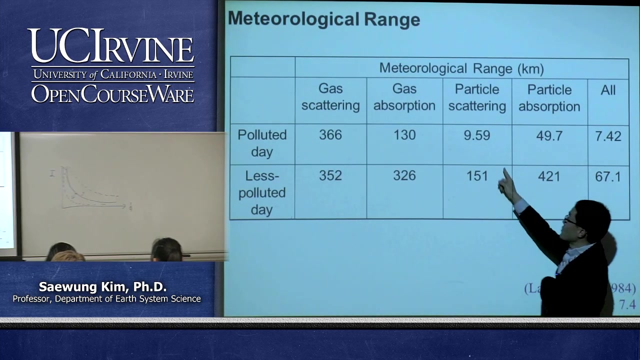 atmosphere anybody. which one is most important factor. again, if there's in the atmosphere only gas scattering, you can, you should be able to see 366, and then if there's only particle scattering in the atmosphere, then you will be able to see 10 km in polluted day and non polluted. 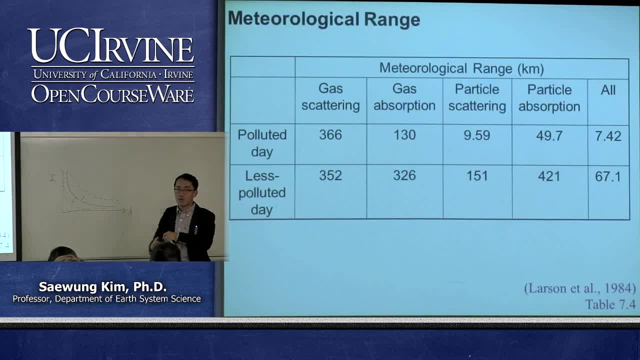 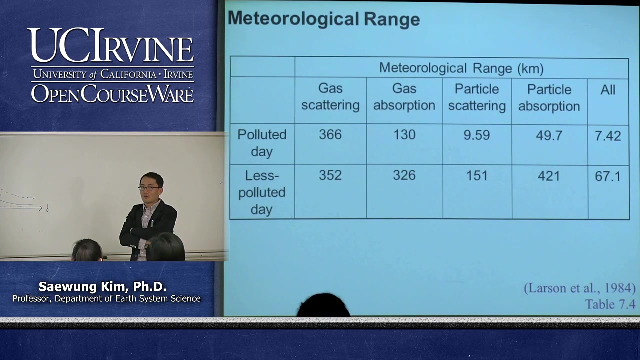 day, you should be able to see 151 km. so I'm asking you which one is most critical factors among gas scattering, gas absorption, gas scattering, particle scattering and particle absorption that determines visibility in the atmosphere. I can go for it. why is that? yes, that's the right answer. 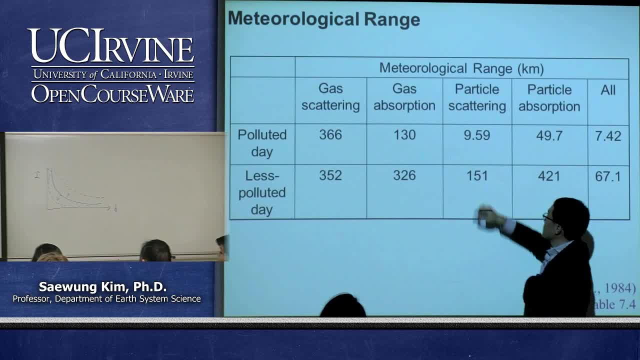 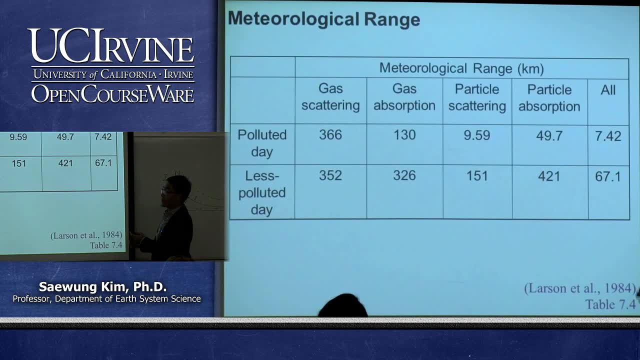 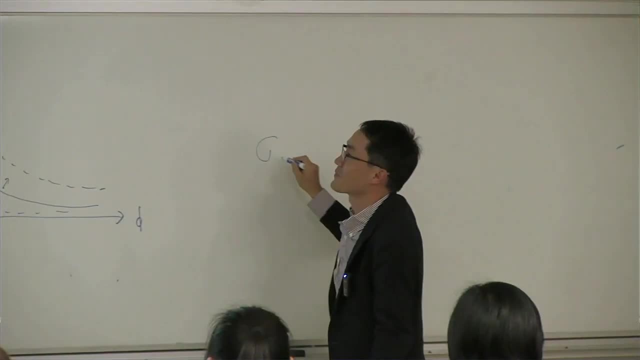 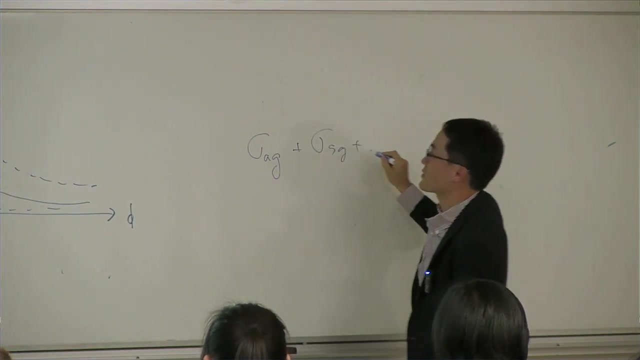 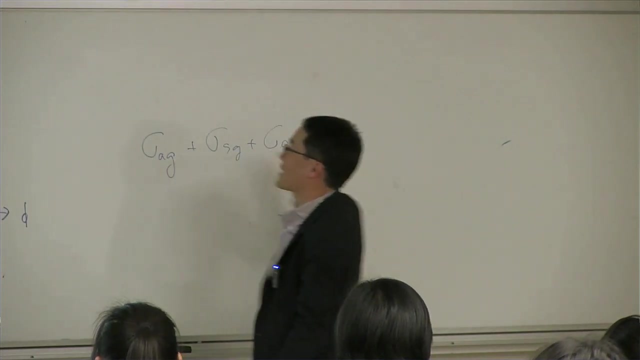 basically so, basically so. so that's kind of quantitative, qualitative approach. so I love math because it's much more straight forward. let's take a look and not many people buy that argument. I will try to change that to your perception. so that's basically total. so that's distance, right? 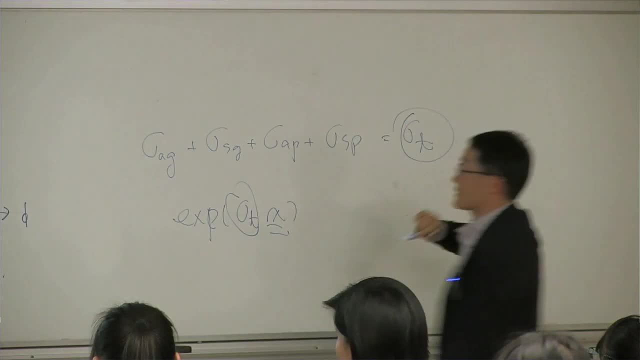 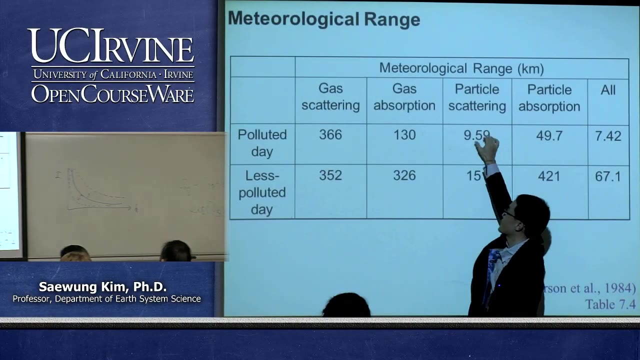 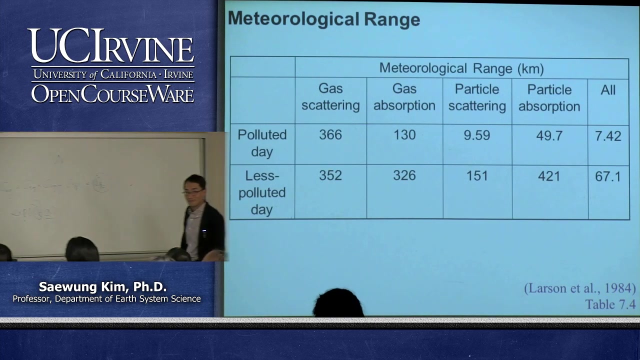 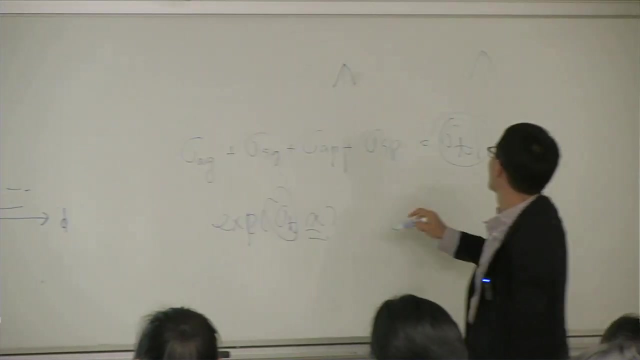 so you are adding these things whole up as this thing, right there. so basically, this means that this scattering particle, scattering has highest value, right? if you have high or this parameter, then you are going to this direction which deters visibility, and then if you have low, this parameter. 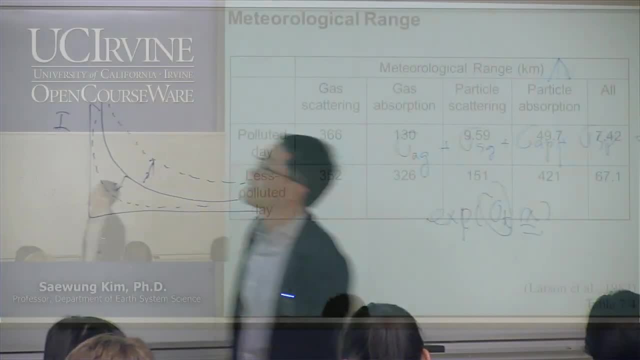 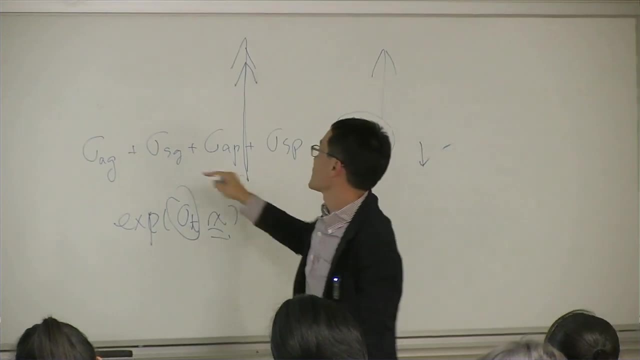 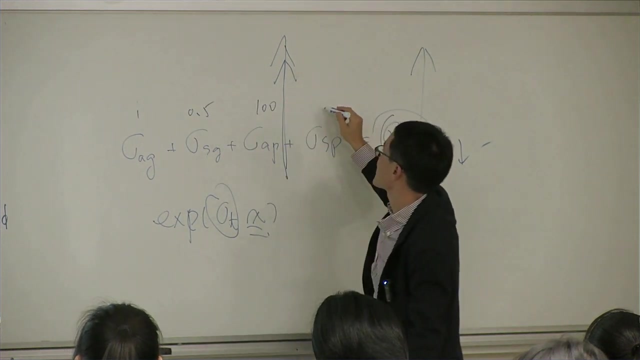 then you are going to this direction, right. so that's last distance means this large. basically, if you just put some number here, it's going to be 1.5, this is 100, and then this is going to be maybe 20. so what's the number? 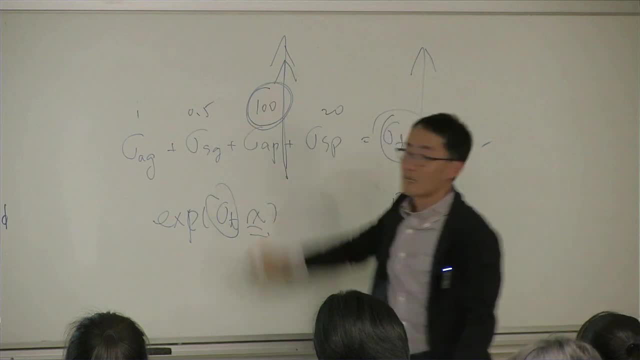 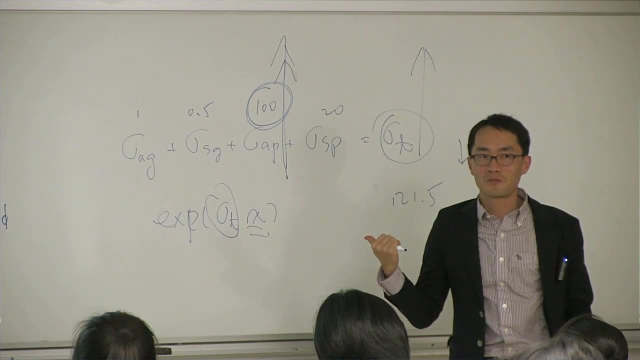 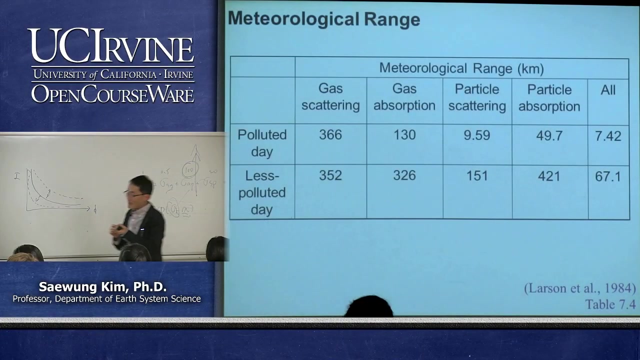 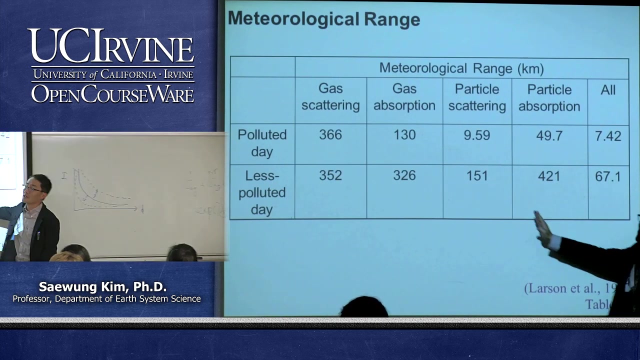 121.5. so most important determining factor is going to be this one. you see, this is easier or difficult, this is more difficult. ok, forget about this, let's go back to this one. so so how many of you got that idea that particle scattering? actually most important one. 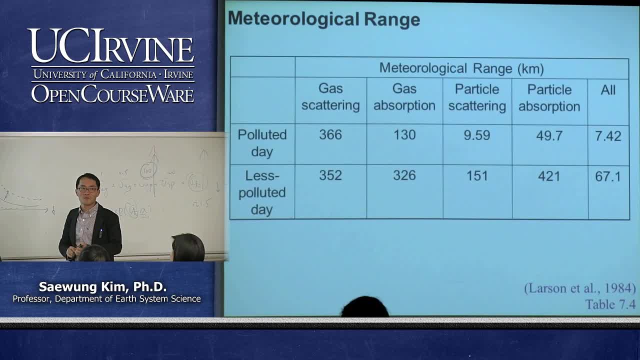 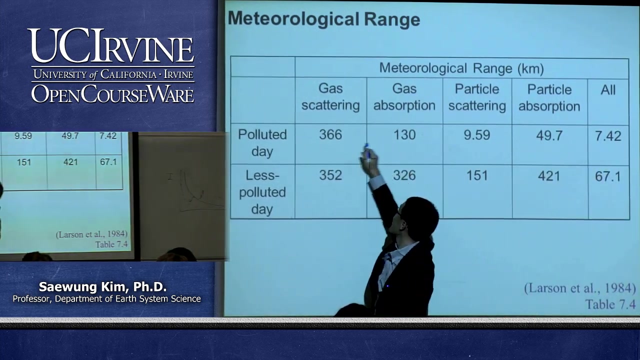 raise your hand, few, maybe 2 or 3, something like that. so let's, let's go back to explain this thing once more. still have 30 minutes, so that's good. so overall, so that's overall visibility right here, right, so we added up everything: gas scattering, gas absorption. 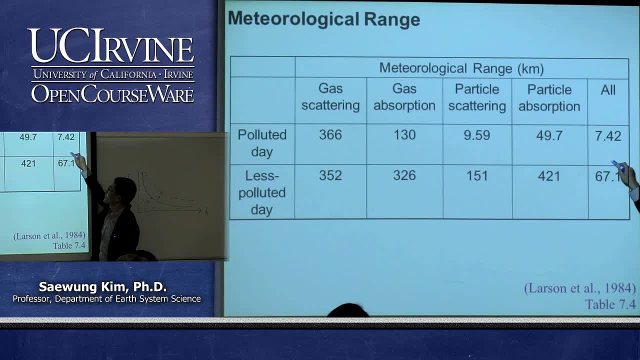 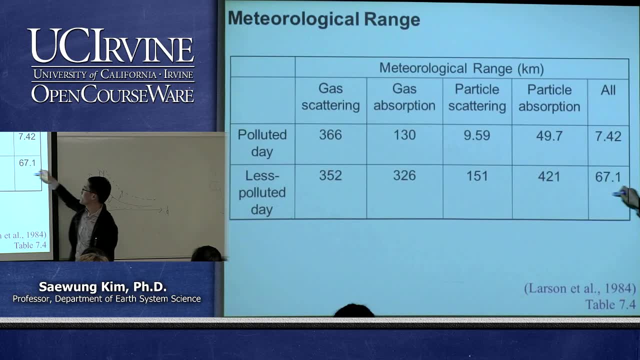 particle scattering and particle absorption. the visibility in polluted day is about 7 km. basically, you can see 7 km ahead of us, right? so in non polluted day we can see about 6-7 km. you can see they are 6-7 km away, right. 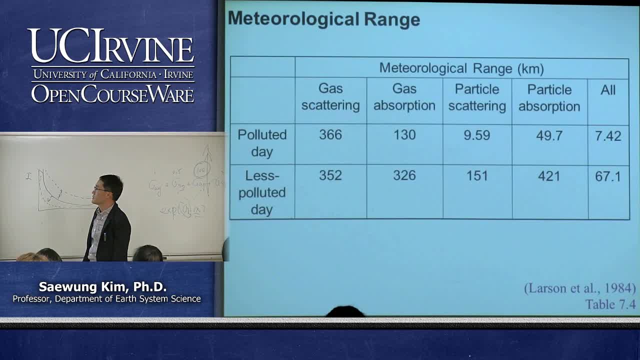 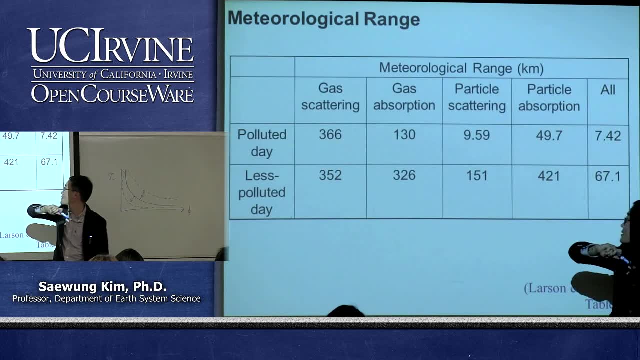 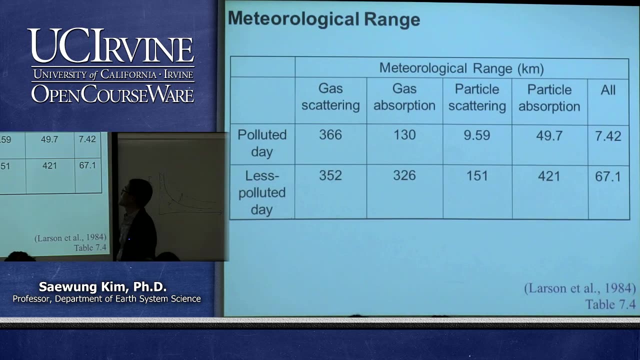 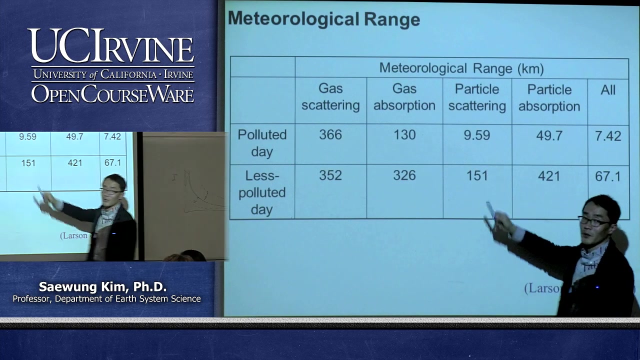 so some magic happens, right, if we prevent this process- particle absorption process, and then gas absorption process, and then gas scattering process- and then we can only make this particle scattering interaction between light and particle, then visibility in that case is 9 km, right? so what's the 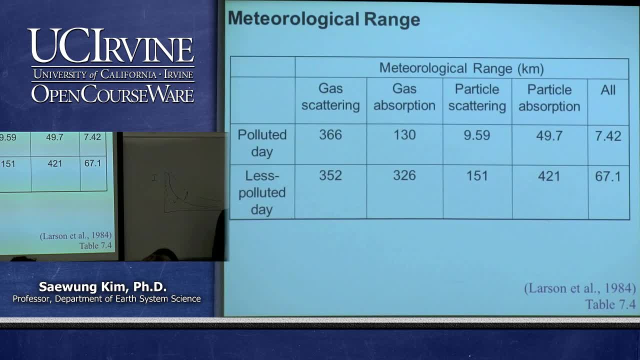 difference between this one and this one: 2 km right, about give and take about 2 km, so 2 km of the visible. the visibility decrease is caused by all three right, only 2 km right. so let's take a look at this one. so if we 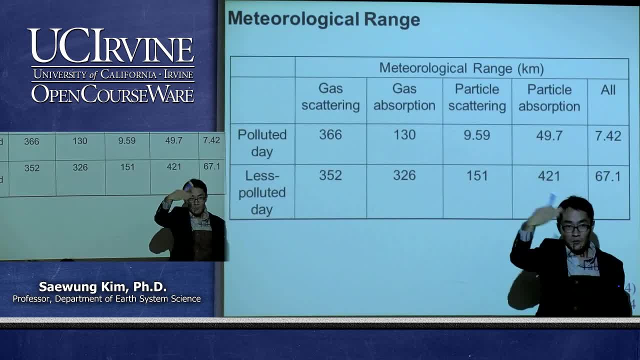 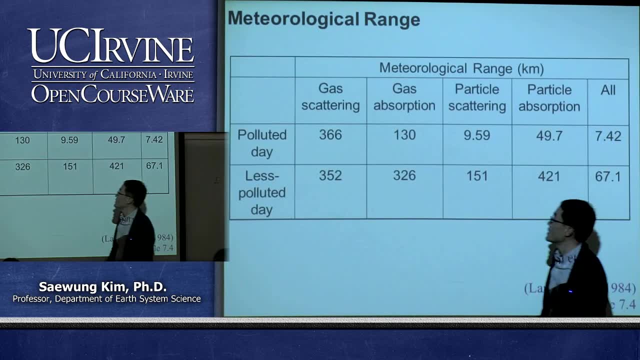 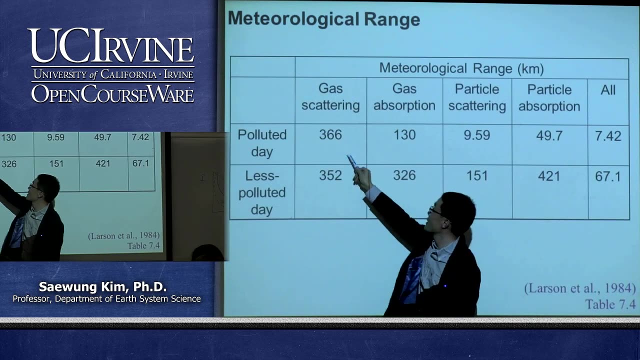 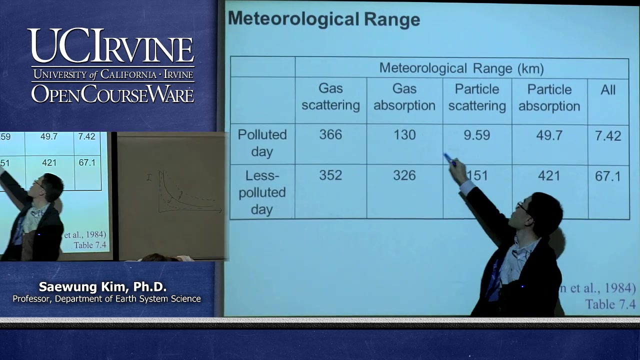 kill all the interaction. if we stop all the interaction between gas absorption, particle scattering and particle absorption, the visibility is 366 km right, so 366, and then, if you add these things up, it's about 7.4 km right. so how much of these three? 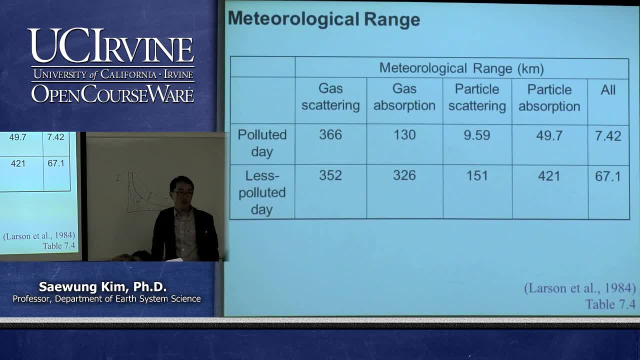 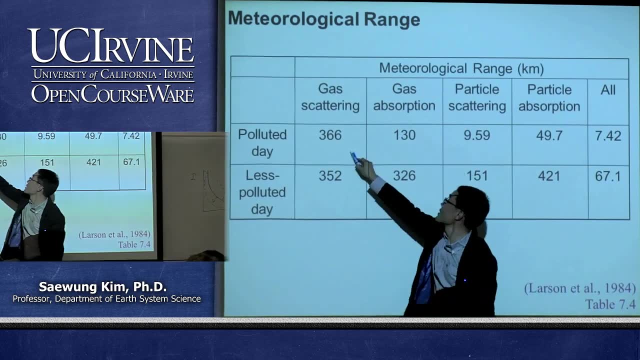 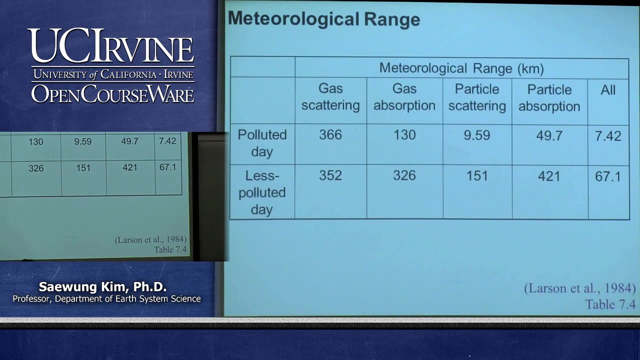 are making the difference about 300 km. right, that's a lot, isn't it? this is only 2 km. the other three, then this one, this, the other three, making 306 km of difference in terms of visibility right. so, basically, this is least important: one, gas scattering and then 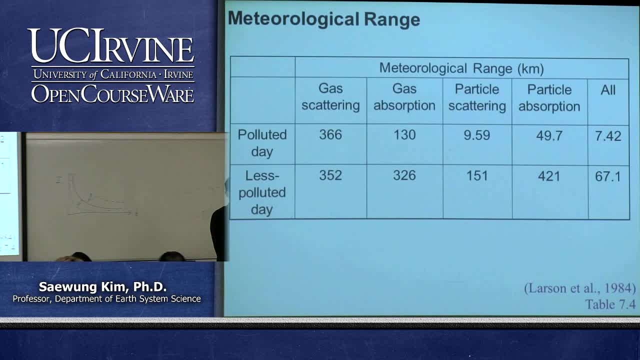 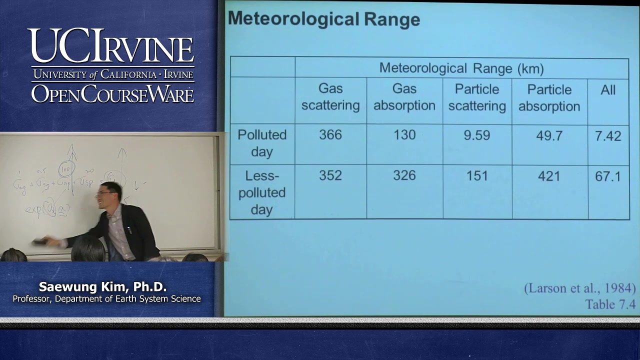 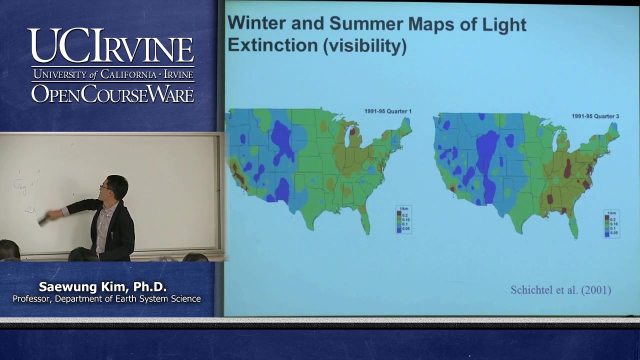 this is the most important one, right? still don't get it? Ian will try hard in the discussion section. so if you don't get any of this, just remember particle scattering is the most important one. okay, so let's make this thing even more complicated. how about this? 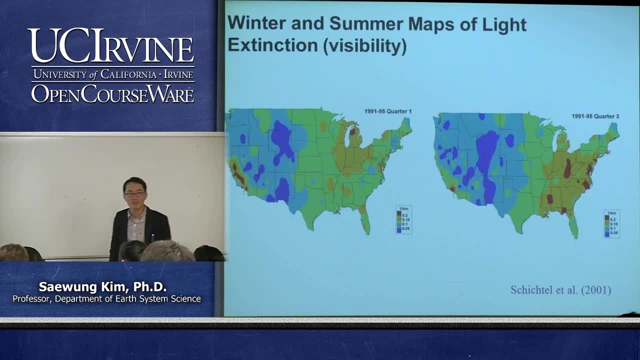 so this is actual visibility distribution all over the United States, alright average between 1991 to 1995. 1991 to 1995. quarter one, which one? what is quarter one? January, February and March. right quarter three, which is June, July, August, no, July, August and September. 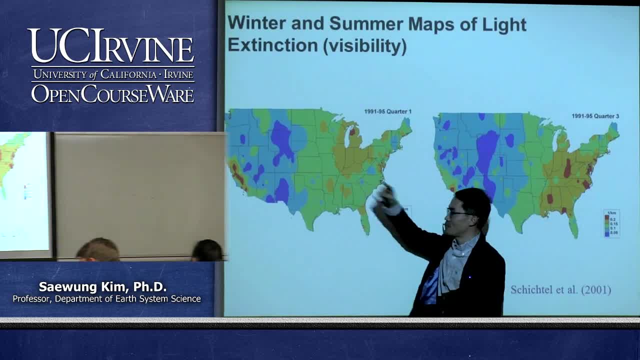 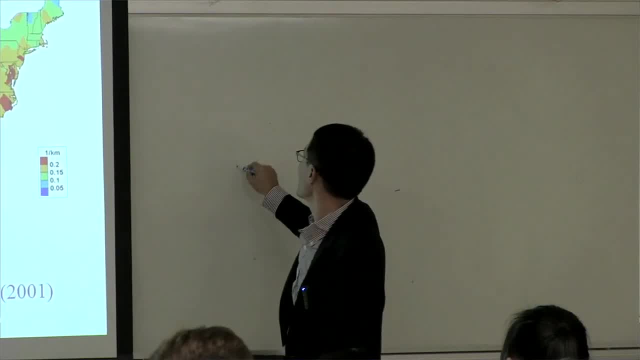 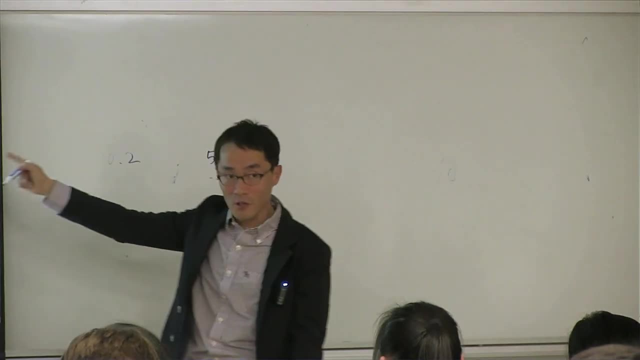 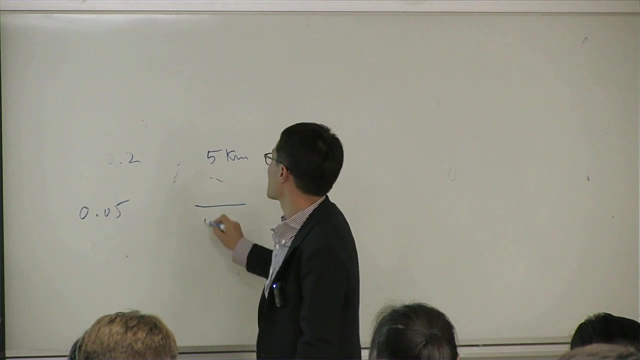 right, so basically, this is summer time, this is winter time, so this is visibility: 1 over km. so basically, 0.2 means visibility of 5 km, right, because that's 1 over km. and then 0.05 means, so basically that's 0.05. 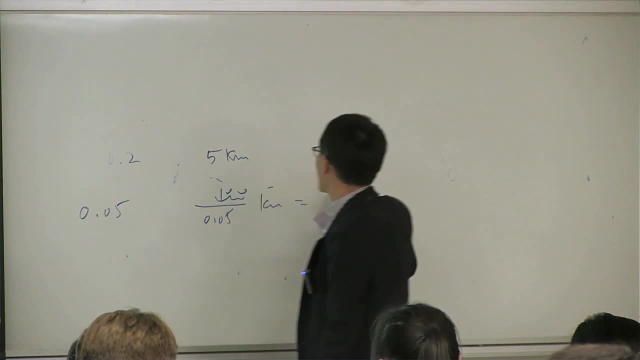 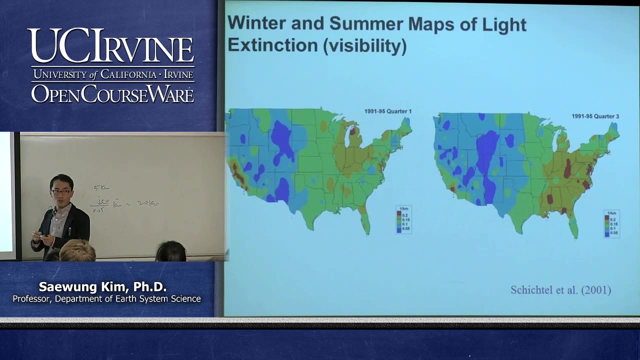 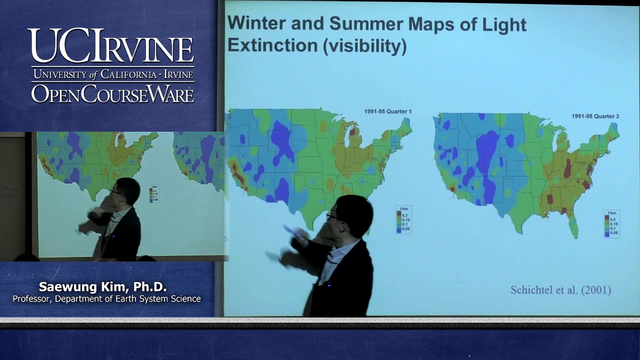 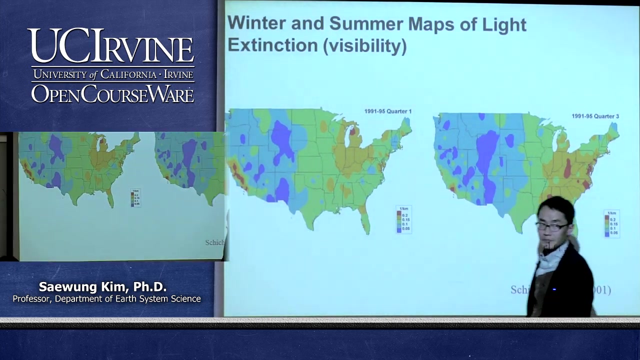 1 km, that's 20 km. so basically, red is bad visibility and then blue is good visibility. okay, so let's take a look at the winter time first. all the bad visibility in California is observed in central valley region, right? how about in the summer time? 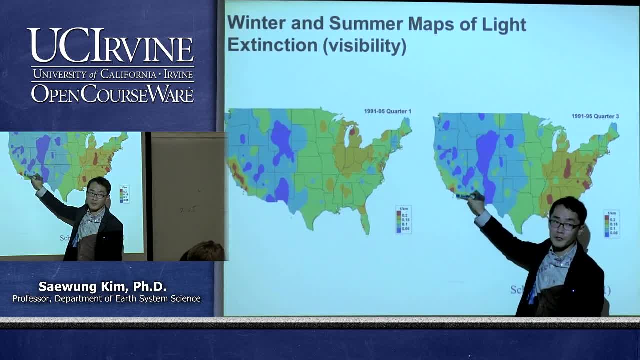 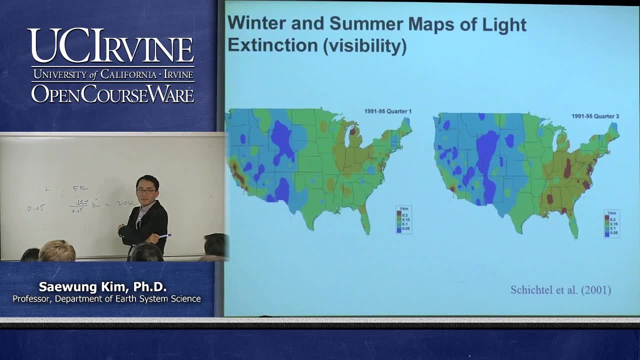 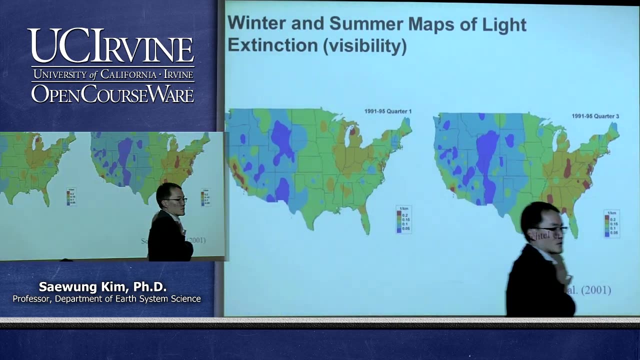 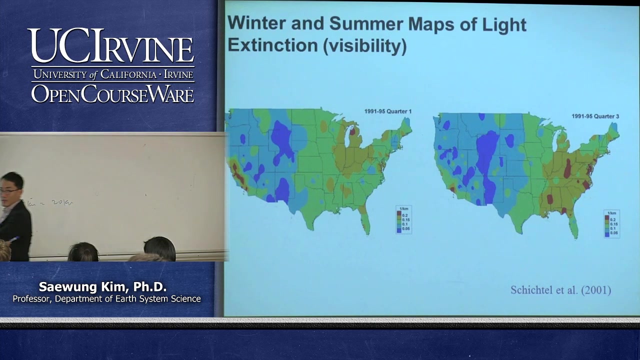 central valley gets better. where is here Los Angeles right? anybody can explain why this thing? this happens: in the summer time, Los Angeles visibility gets worse. in the winter time, central valley visibility gets worse. what's the difference? which means that air pollution, particle scattering, gets higher in central valley. 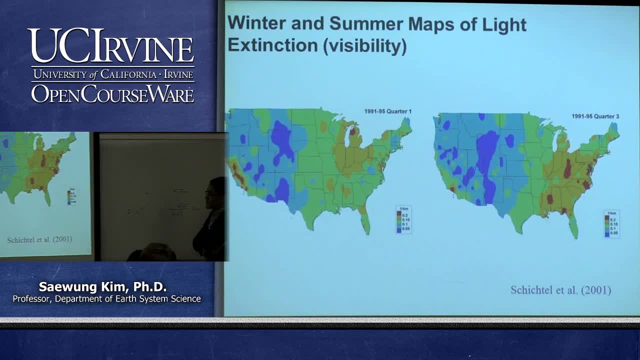 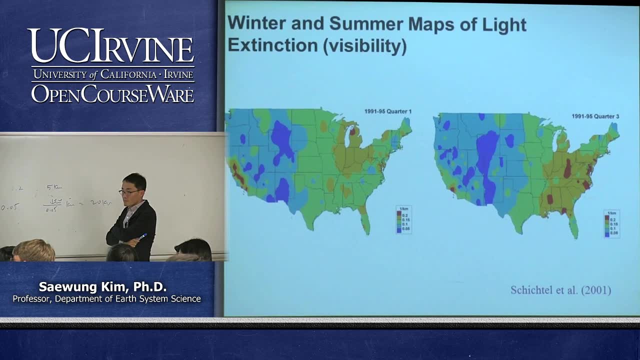 in the winter time and then gets worse. yup, Los Angeles uses a lot more energy in the summer for air conditioning. so you think energy production is actually happening right that place. it's coming from power plants, isn't it? power plant can be located in any place, probably not. 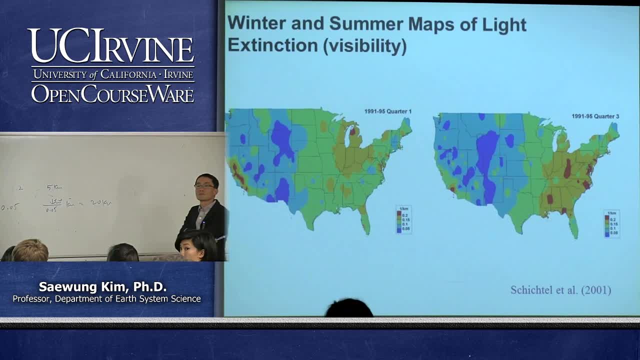 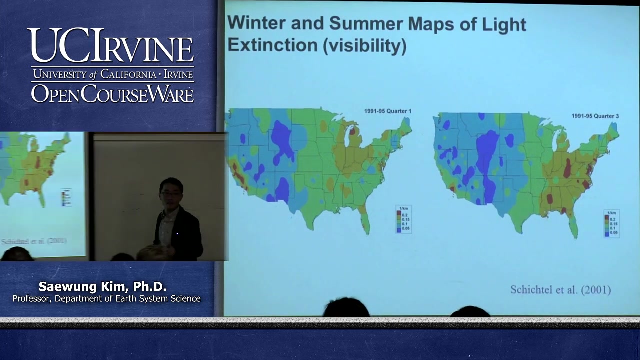 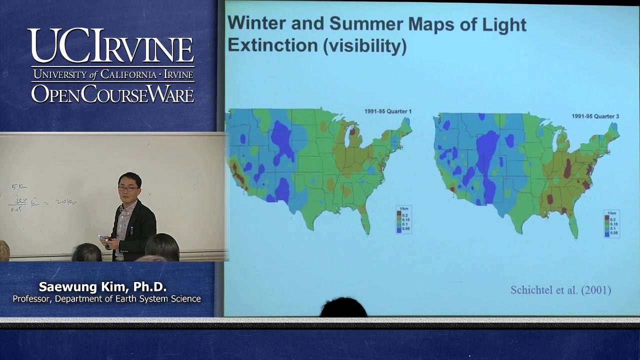 in Los Angeles downtown, I guess, say that again, during the summer time, higher temperature everywhere. I guess, what's that? that's yeah, usually in the winter time out here. so that's central valley. go for it. doesn't the earth radiate, radiation during the summer more? that's true. 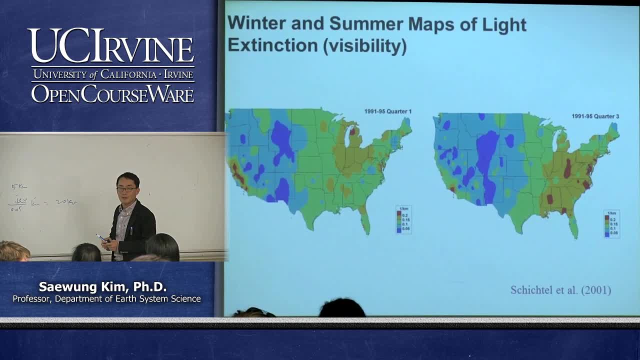 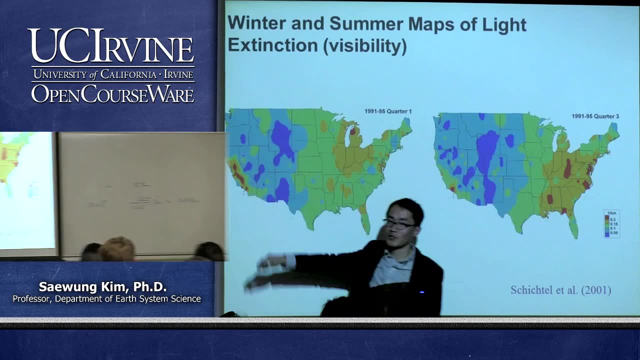 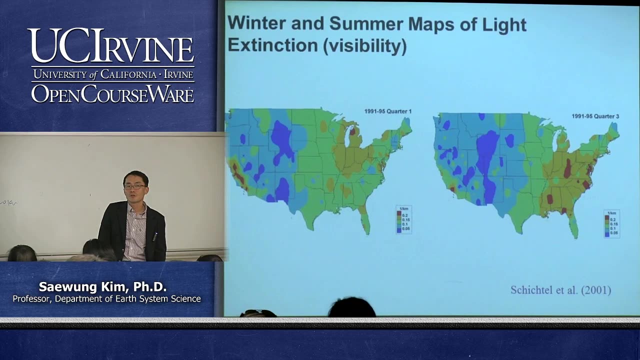 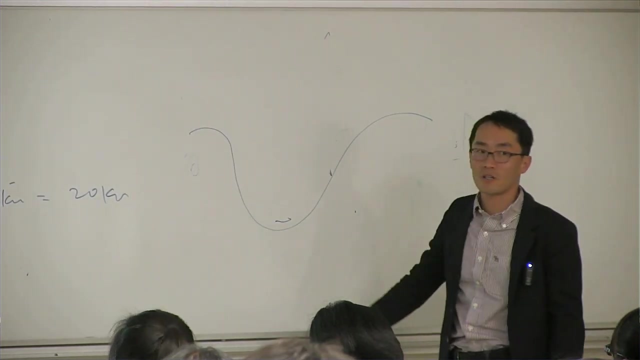 in winter, less radiation happens, so more pollutants are circulating, making it worse. we are getting there. so let's take a look at this winter time scenario. so that's yeah, that's central valley, right. so definition of central valley just valley region. during the winter time, there's a lot of air pollutants accumulated. 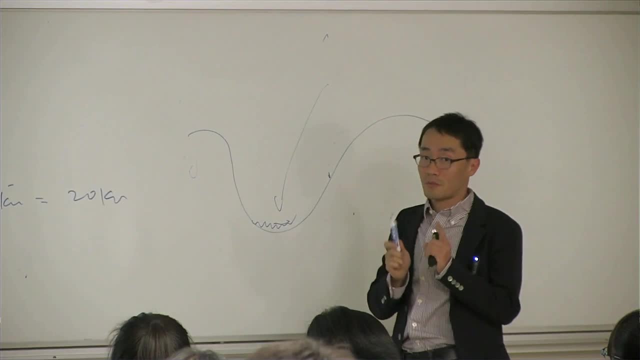 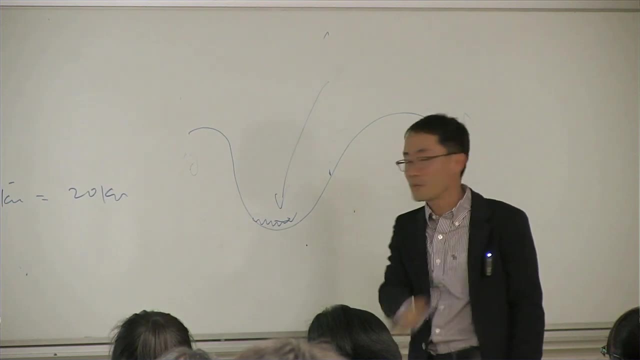 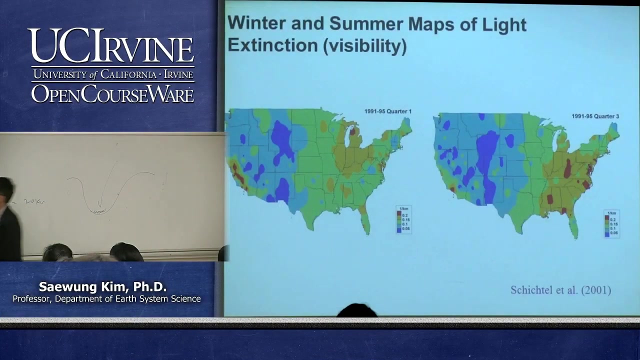 less solar radiation coming in. so one of the former question was about related with this thing. in the winter time you don't want to do outside activity in the early morning because it accumulated air pollutants. that's happening more in the valley region, so that's why central valley visibility. 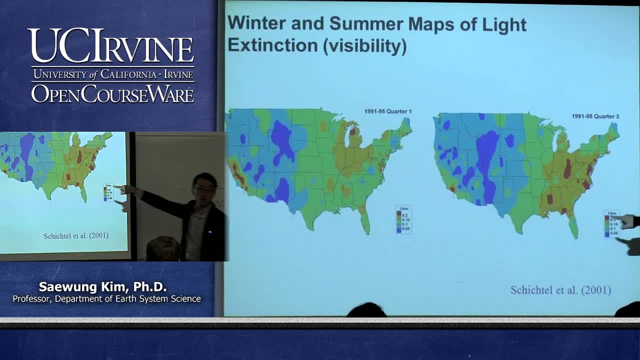 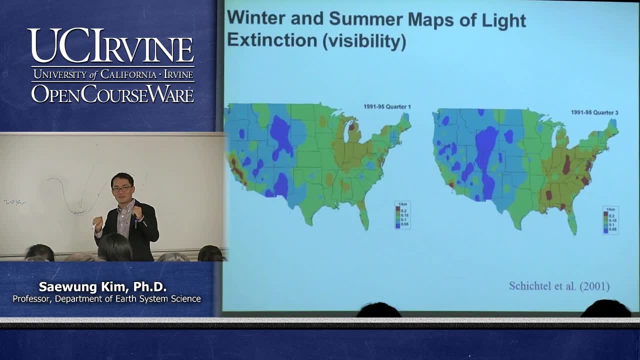 is bad during the winter time, and then why summertime in Los Angeles is bad? come on it's. we talked about smoke. what? the two different kind of smoke, London and what? yeah, Los Angeles smoke which is produced by. so what cause the photochemical smoke, Los Angeles type smoke? 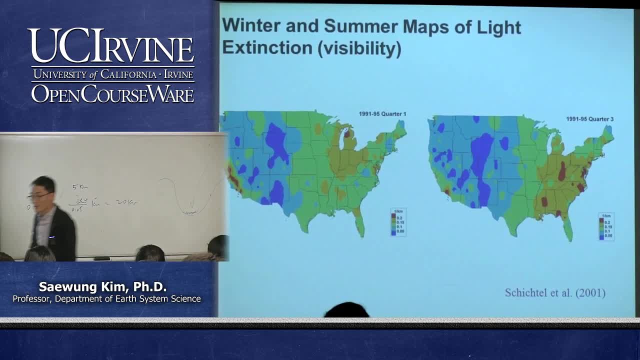 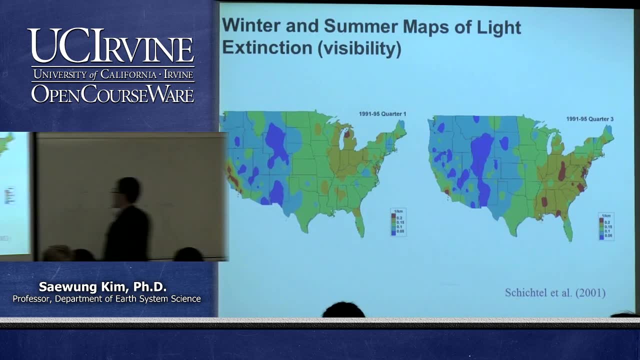 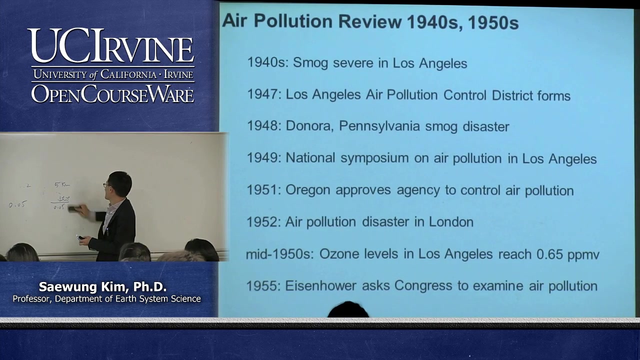 what energy? sun, right. solar radiation, right, this reaction. so that's why in the summertime it's bad, right, okay? okay, let's talk about regulation. even more funny topic. so we talked about pollution so far, then let's take a look at the regulation side a little bit. 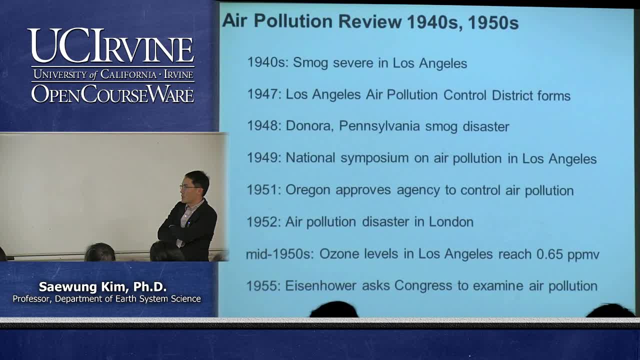 how kind of a government trying to decrease that all air pollution problem. we talked about London smoke and Los Angeles smoke. it is all started. we found that it is gets worse in mid 40 and then so a lot of severe small found the in the 40 timeframe especially. 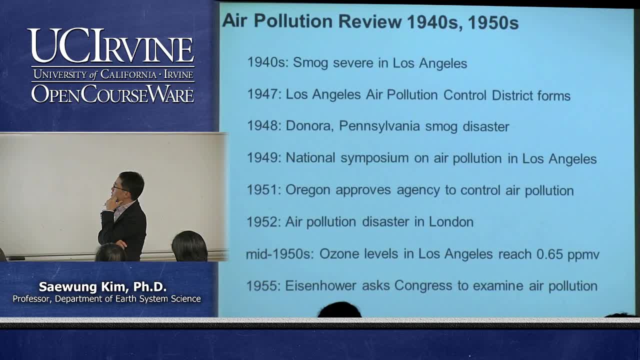 in Los Angeles region. so there's a lot of effort to control air pollution problem in local government, like state and city. so it's first started as the city level and state level regulation and then in mid 50 finally federal government start to propose some regulation after. 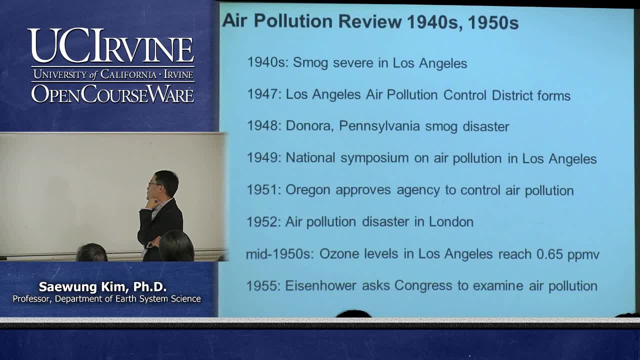 Los Angeles gas. about 650 ppb of the ozone concentration was reported. anybody can guess what's gonna be our concentration right now outside. it should be about 40 ppb, so that 60.65 ppm is 650 ppb, so that's about about 20 times. 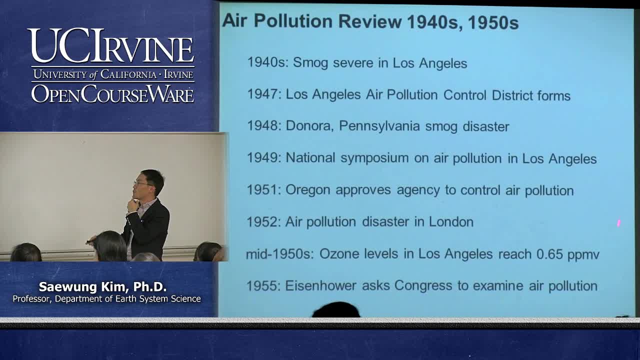 higher than what we have right now. if ozone gets this high you can actually smell it and then you really need to wear the gas mask in this higher concentration. so it's only 60 years ago. you may think that 60 years long time ago. history kind of thing. 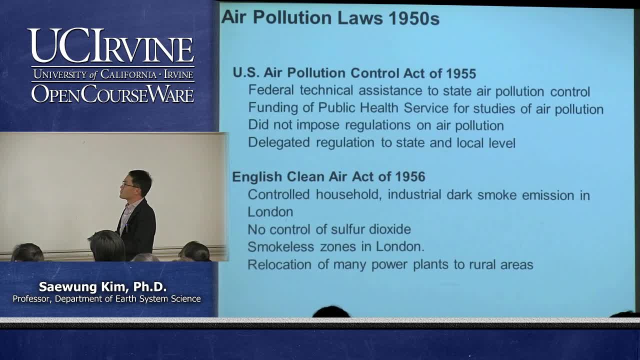 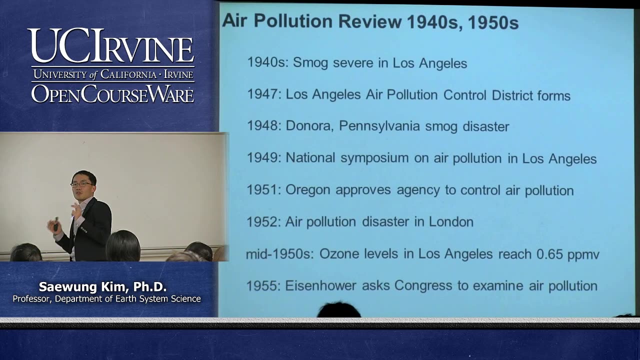 it's kind of your grandparents generation. so so US air pollution act, so that's kind of federal government wide regulation started in 1955. again, it's kind of landmark thing is happening always, kind of big disaster is happening before people start action. that's kind of a. 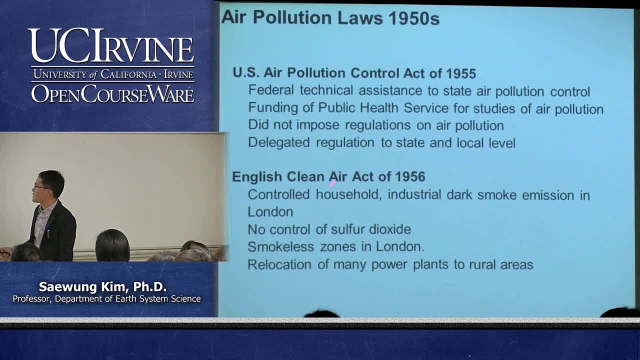 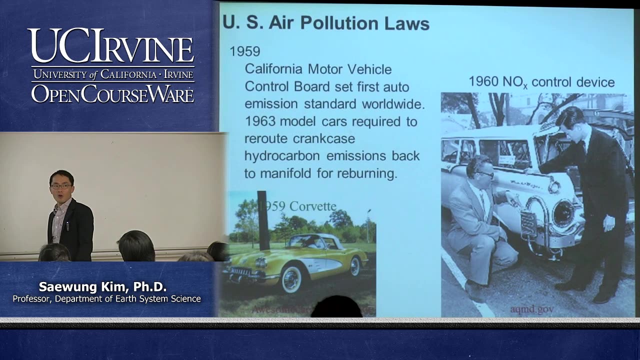 history that you can take a look all the time. and then in UK it's about 1956 that the kind of federal government wide regulation started. but you cannot simply ask people not to drive your car to reduce air pollution because you know our lifestyle already gets into driving. 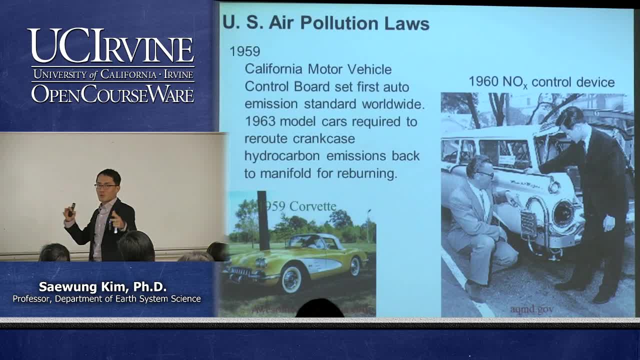 car and people start to live in suburb. so basically social structure is: force you to drive. so at that time, once you reach that, the environment problem gets very, very bad. then you cannot simply go back. so what people usually doing is making some device or technological breakthrough to 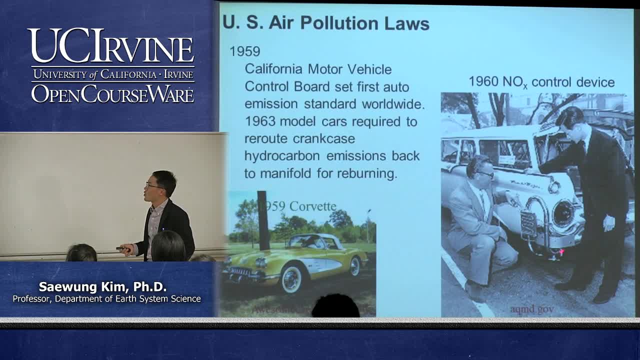 address that environmental problem. so in this case, in terms of emission converter, so back in old days, in 60 actually, people putting this device outside of the car, which makes the car pretty ugly. so basically what this thing is doing is that we talked about incomplete combustion, so carbon. 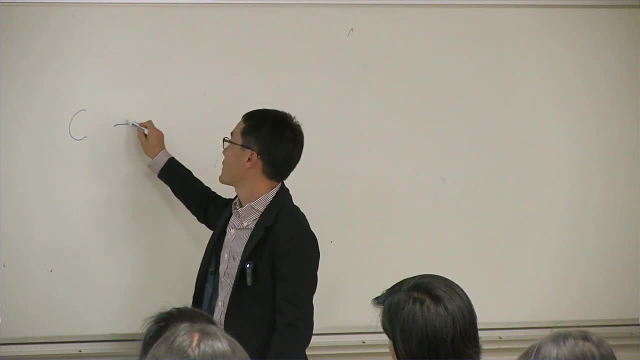 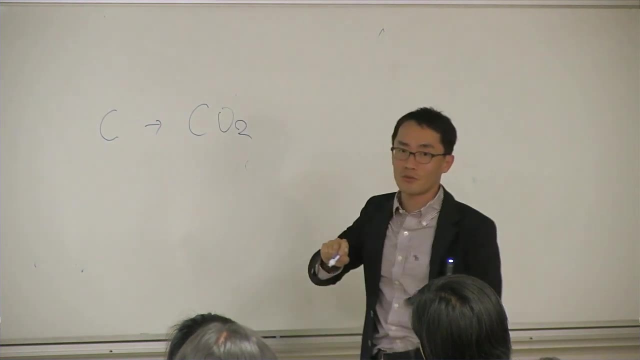 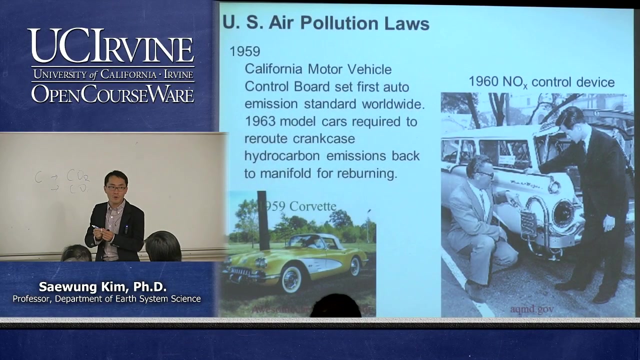 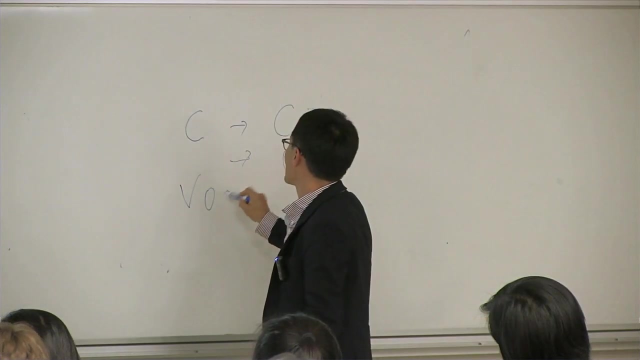 which is organic compound. incomplete combustion is going to make what? incomplete, not complete combustion? complete combustion is going to be making CO2, right, incomplete CO and then all those gasoline is volatile organic compound and then that extra kind of combustion bed making VOC, and then kind of burn this thing into. 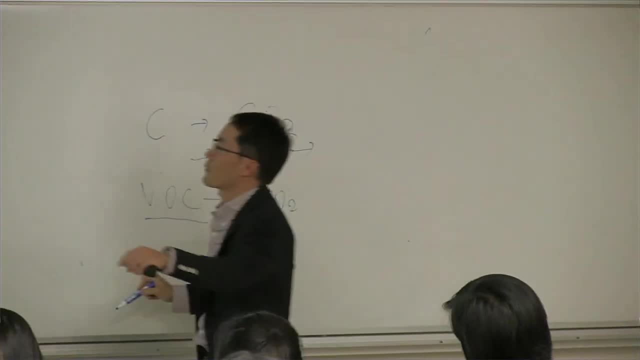 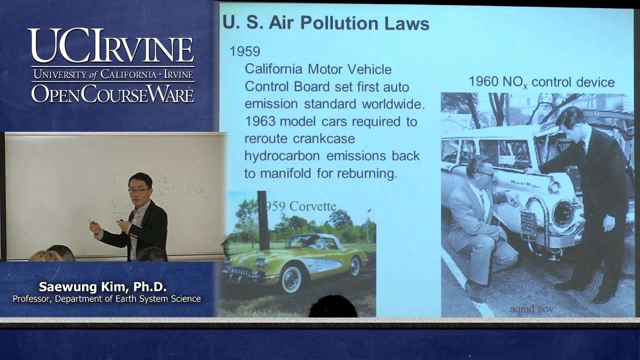 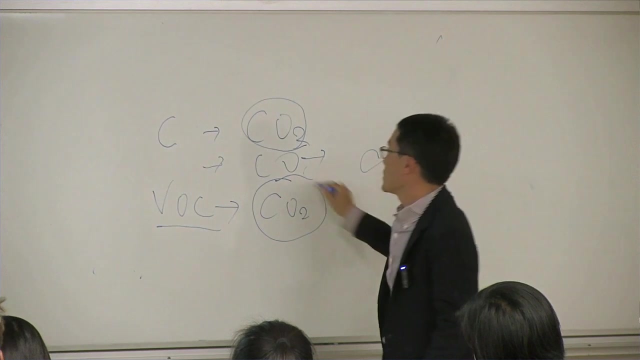 all CO2. so this extra step will make this CO into CO2. okay, that's the idea to putting this extra bed of the combustion. so so making more time to make complete combustion to make CO2 which not cause Los Angeles type smog, but obviously CO2 can. 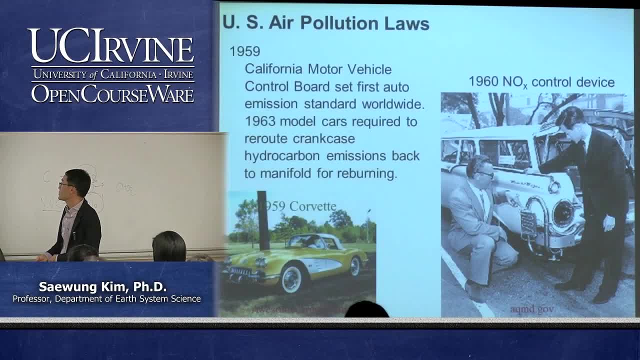 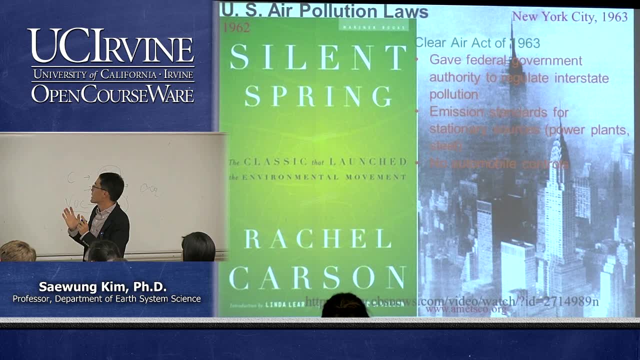 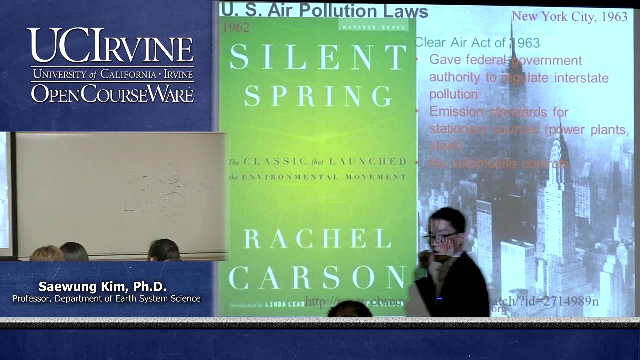 cause other type of the environmental problem that we will discuss later. so one of the kind of a landmark publication about that environmental regulation is this Rachel Carson's book called Silent Spring. how many of you actually heard this book couple? so let's take a look at this video. 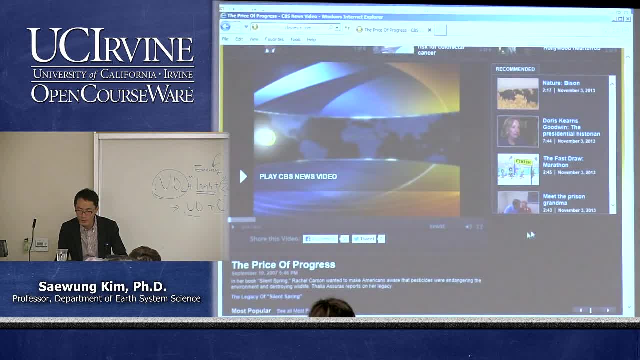 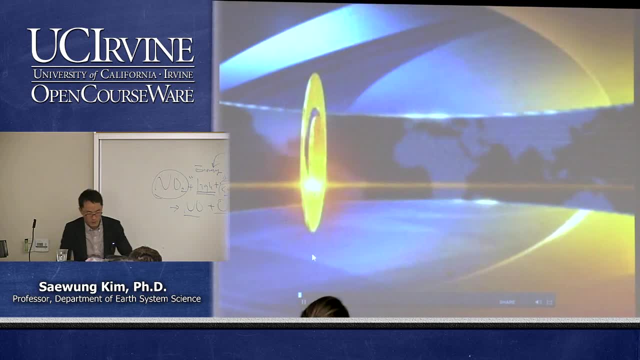 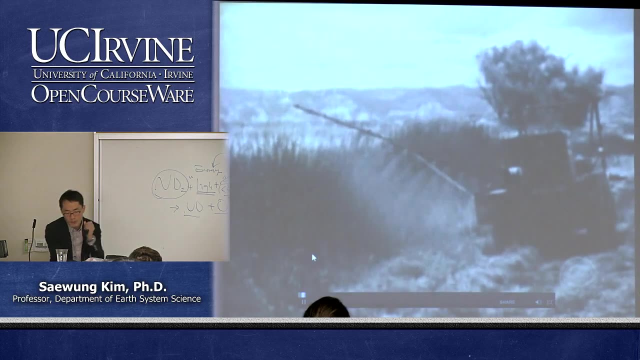 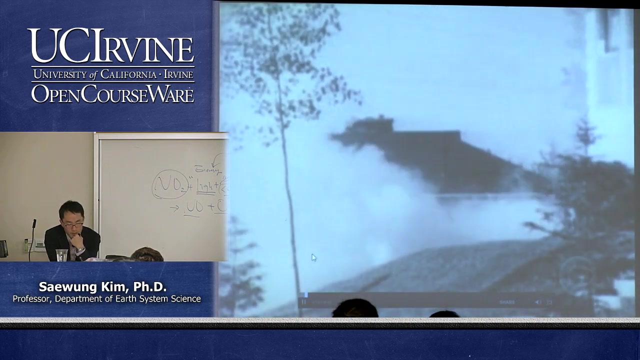 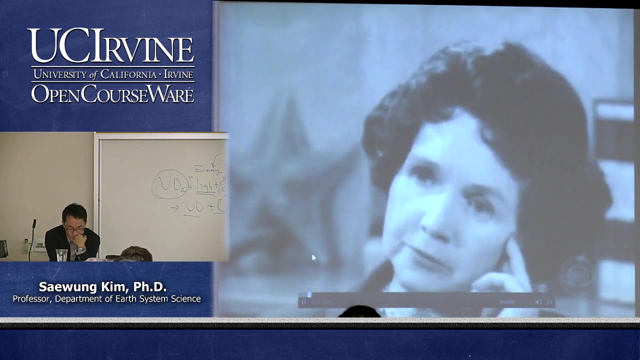 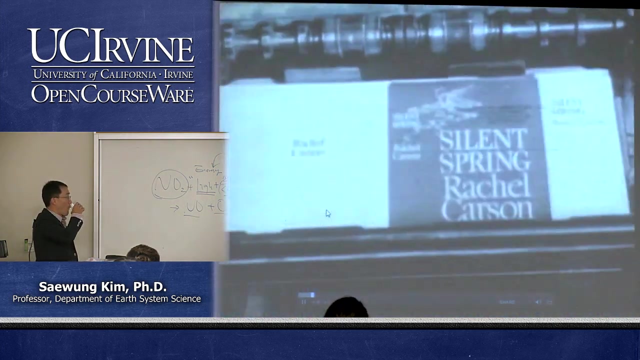 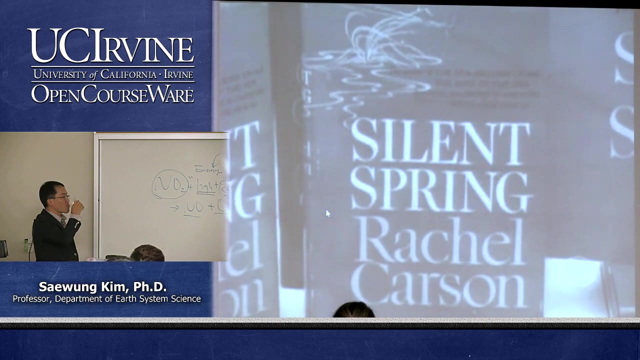 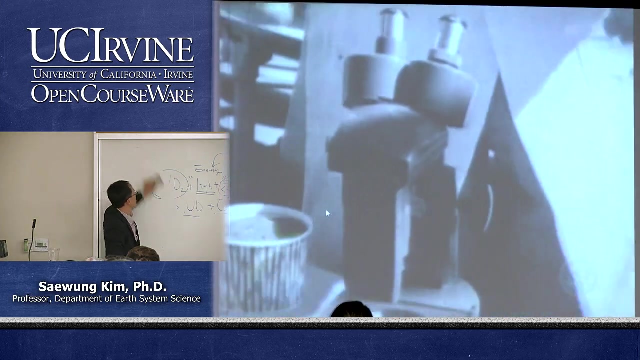 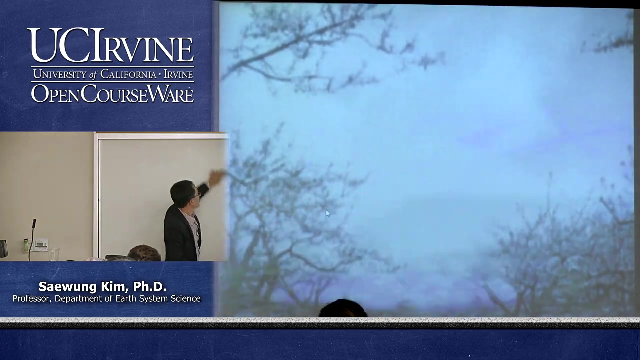 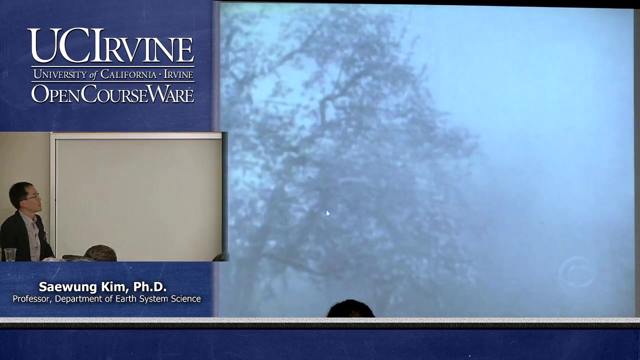 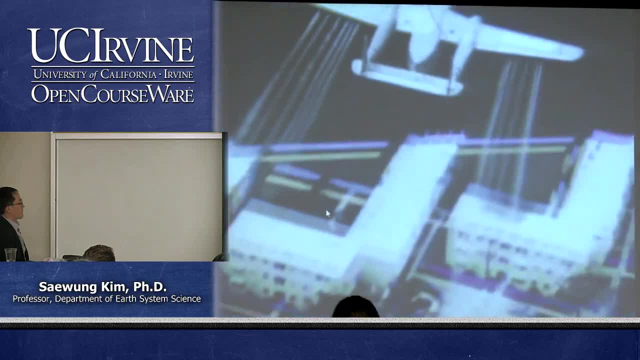 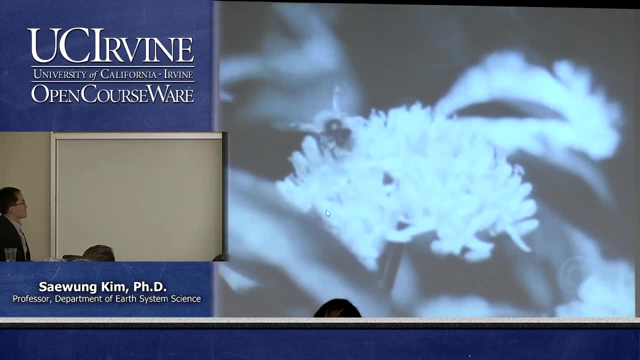 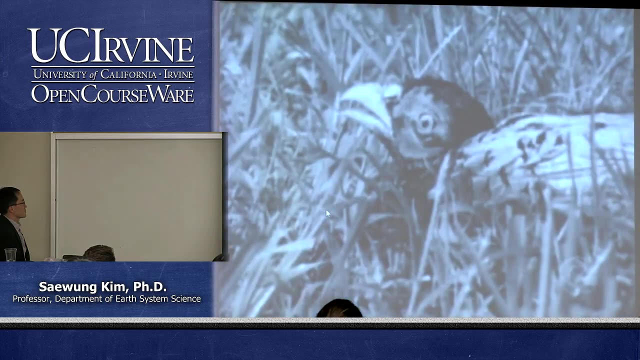 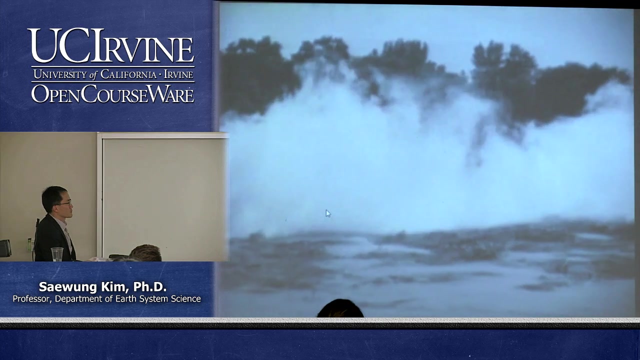 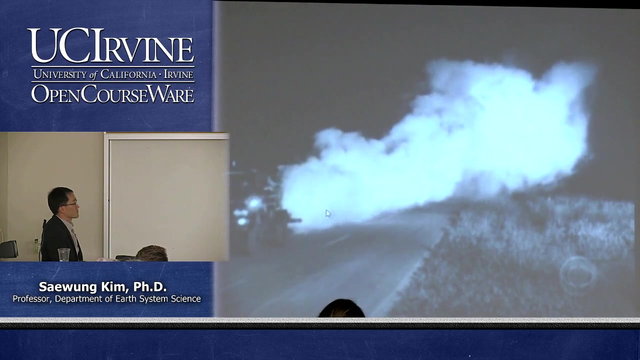 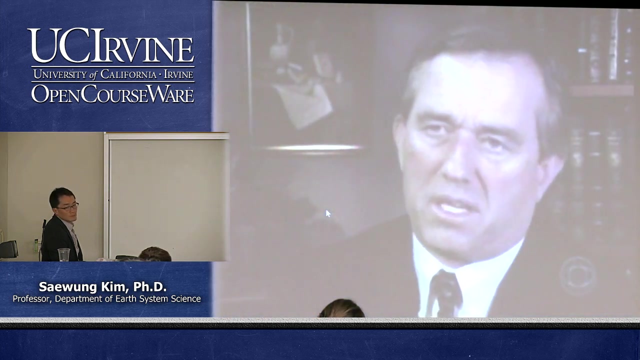 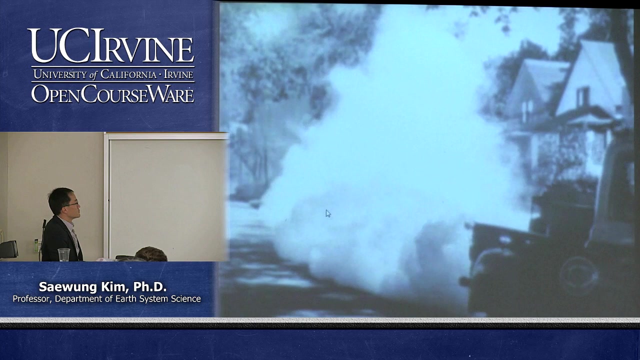 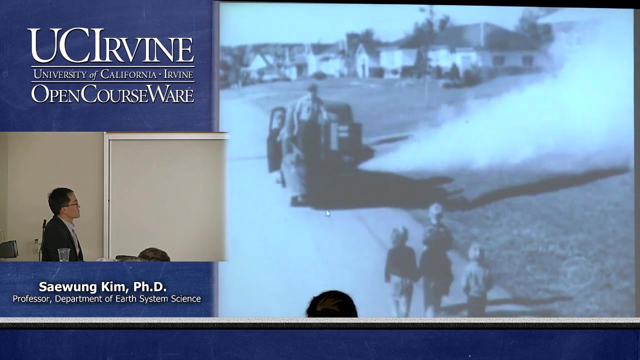 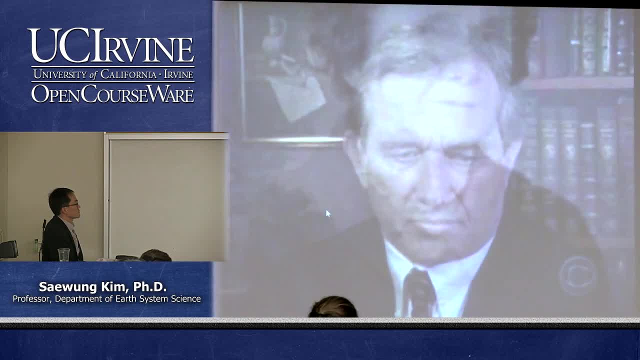 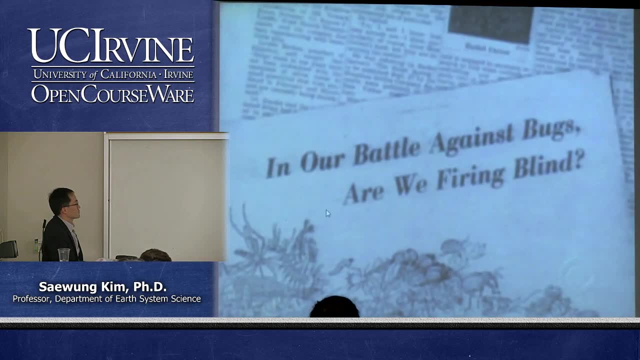 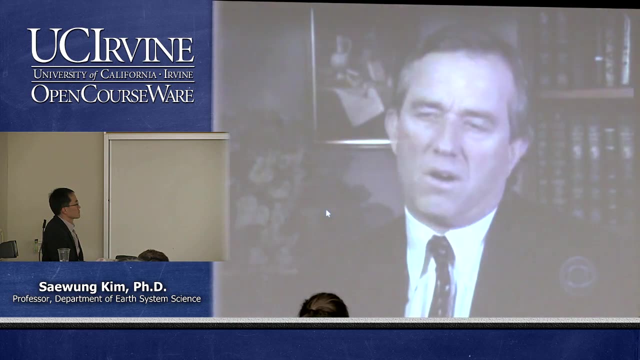 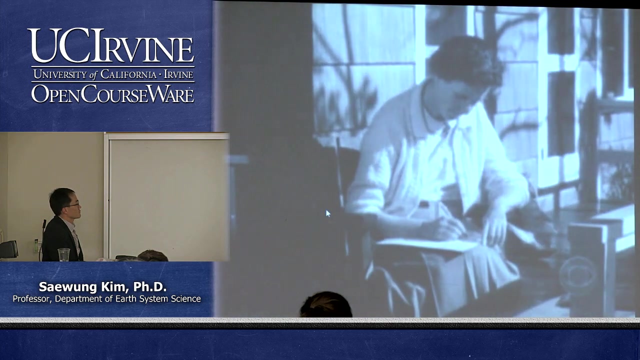 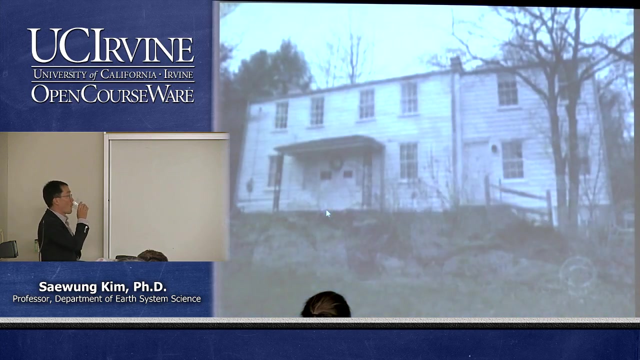 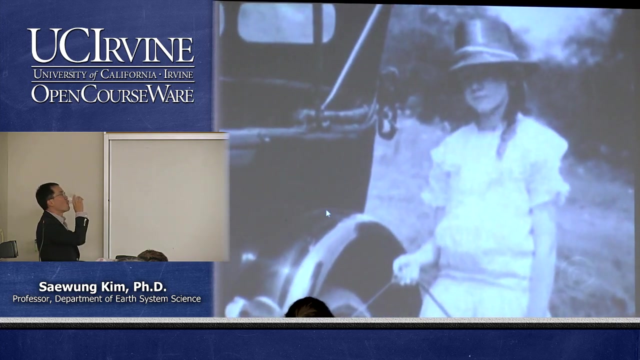 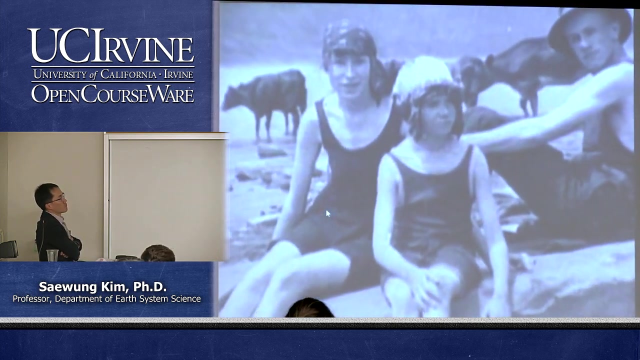 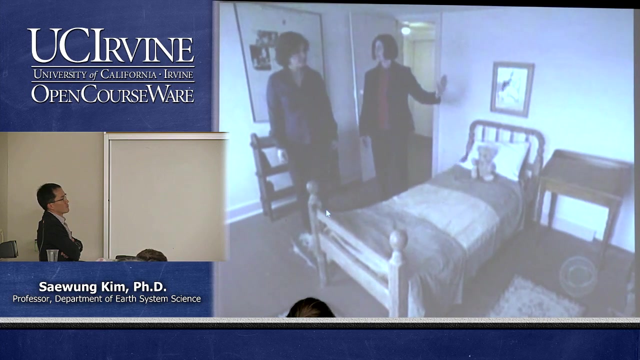 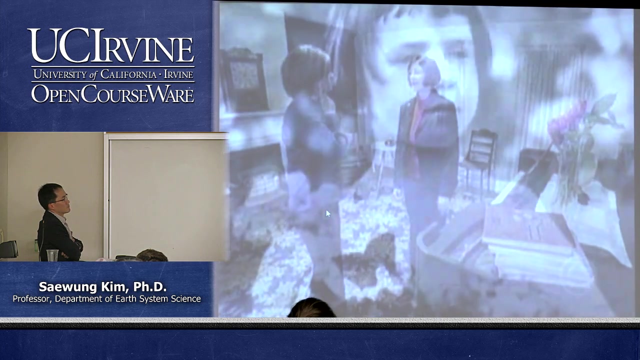 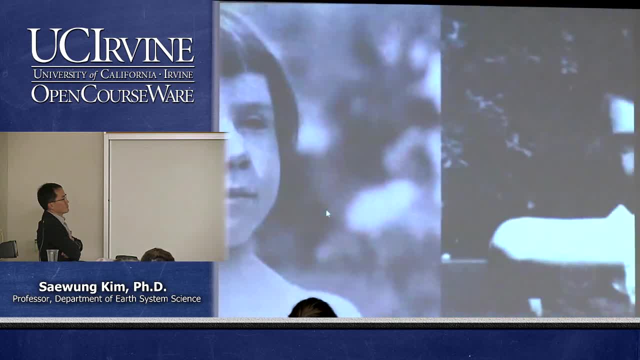 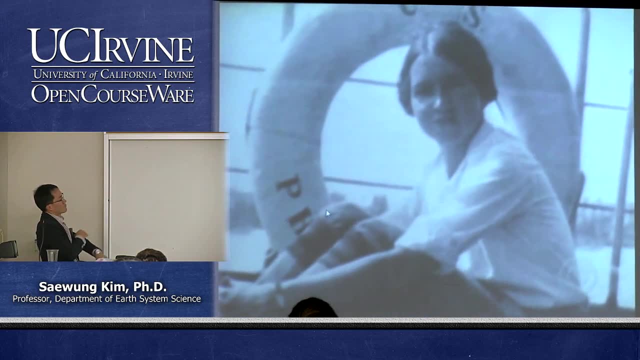 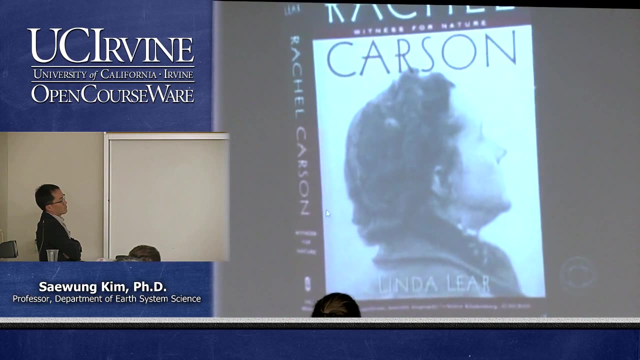 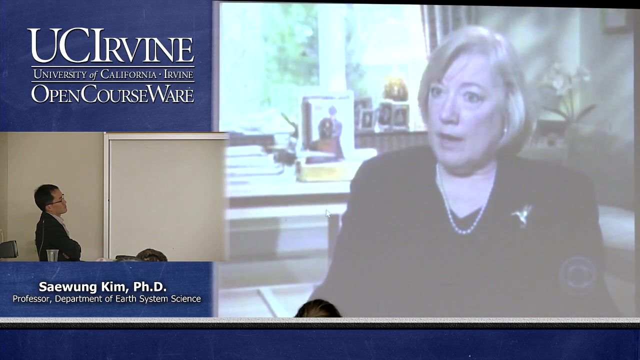 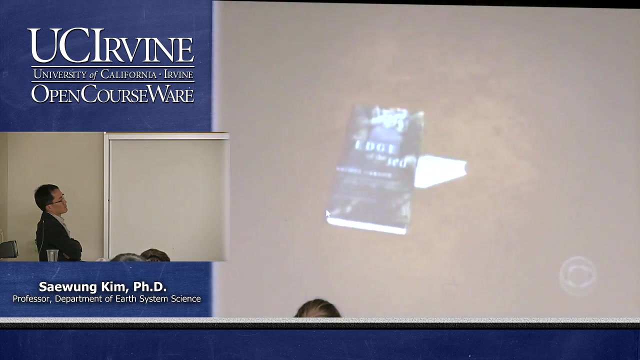 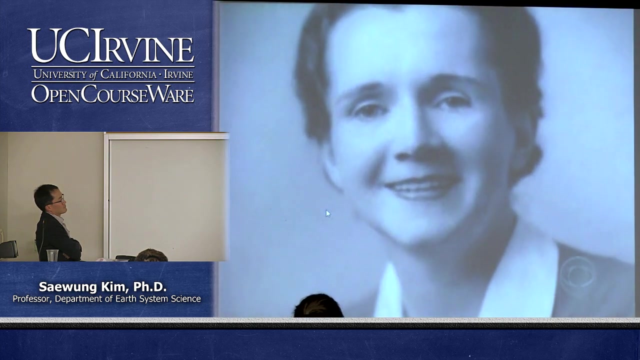 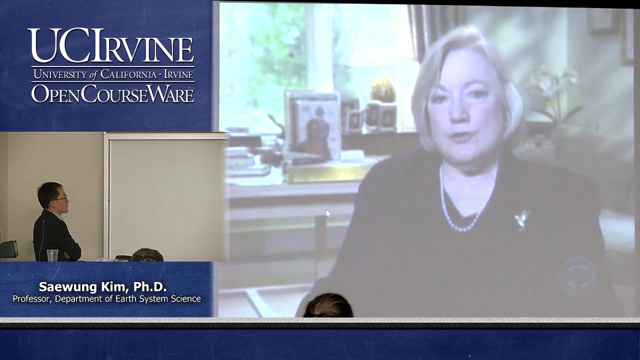 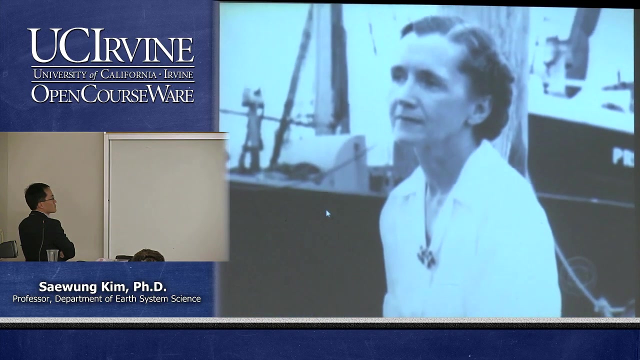 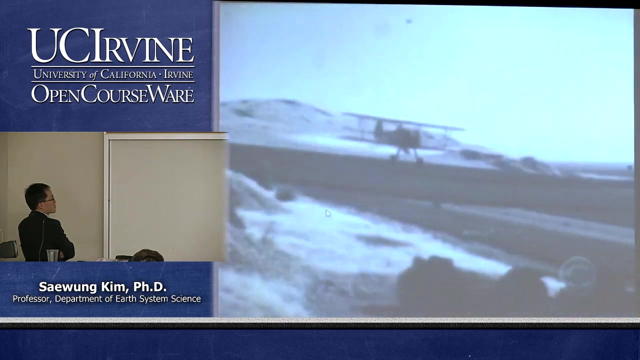 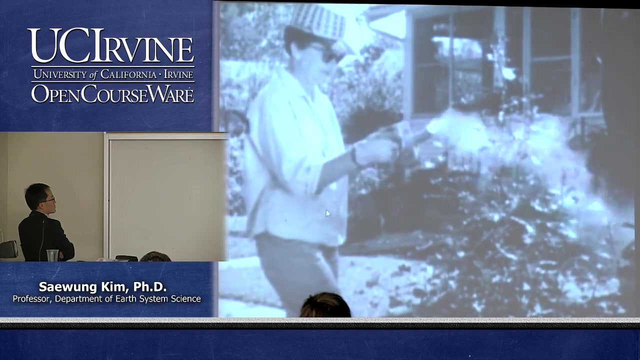 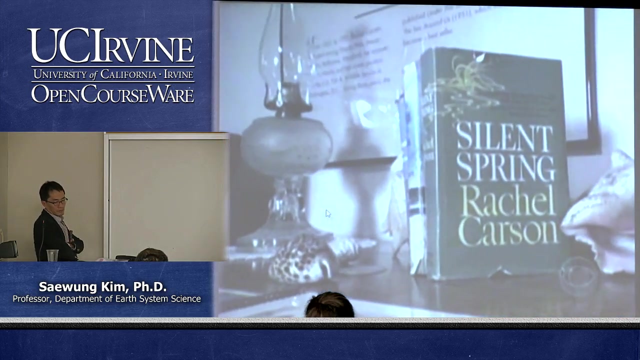 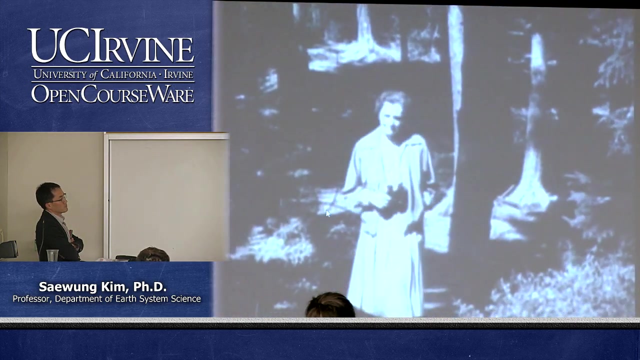 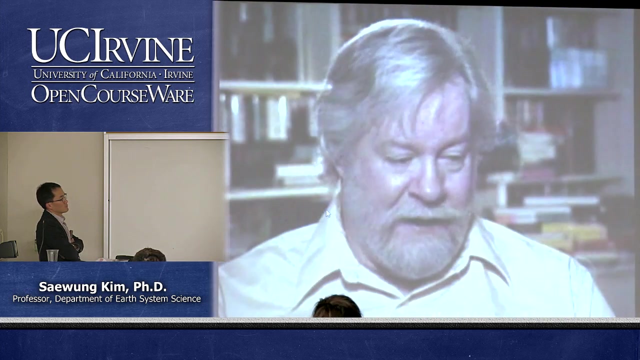 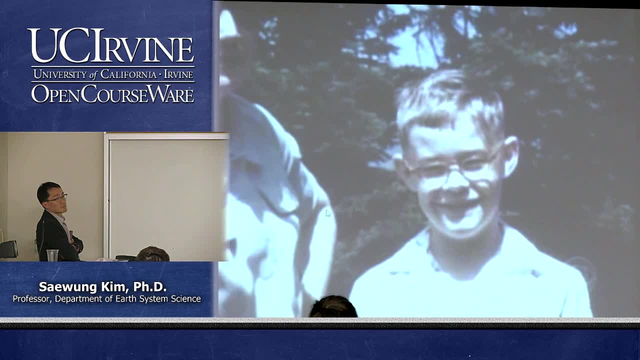 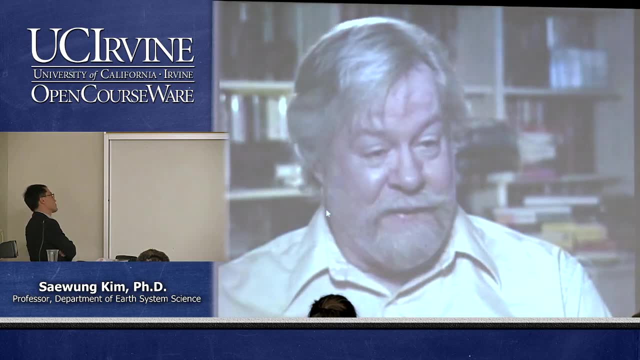 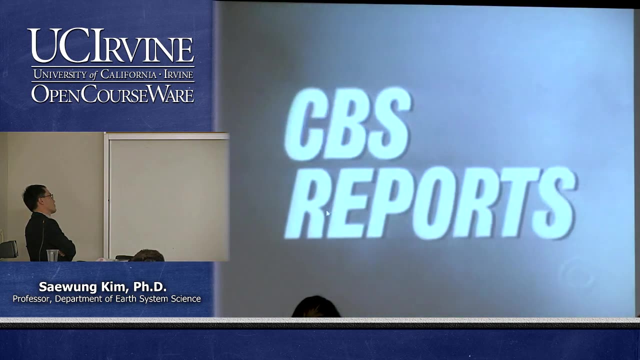 I did. Roger Christie is Carson's great-nephew. Carson adopted him when he was five and she was just shy of 50. Nobody talked to me about it, but I think subconsciously I knew she was dying Through sheer determination. Carson participated in an hour-long CBS News documentary on pesticides. 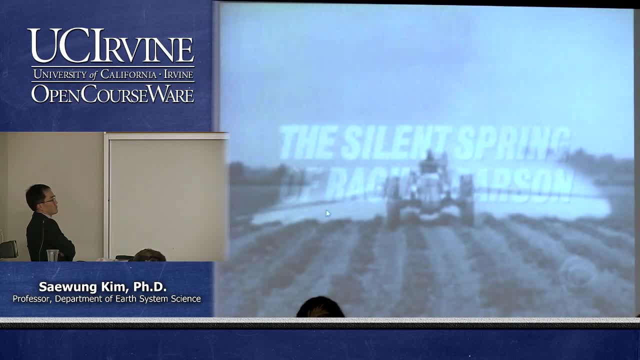 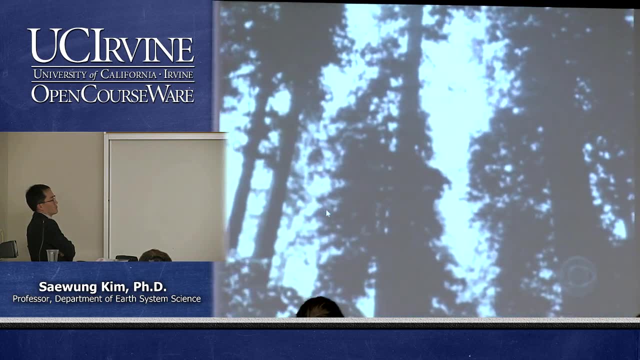 CBS reports The Silent Spring of Rachel Carson, Which aired not long after Silent Spring, became a national bestseller. Can anyone believe it is possible to lay down such a barrage of poisons on the surface of the earth without making it unfit for all life? 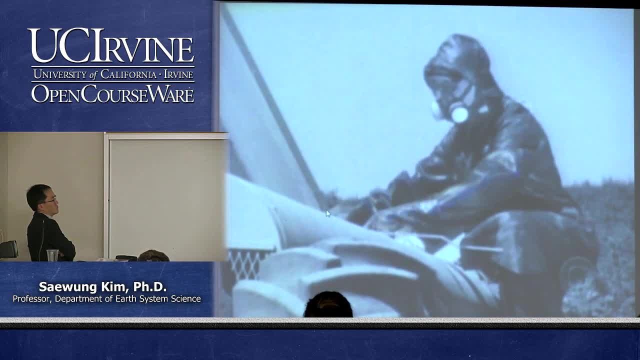 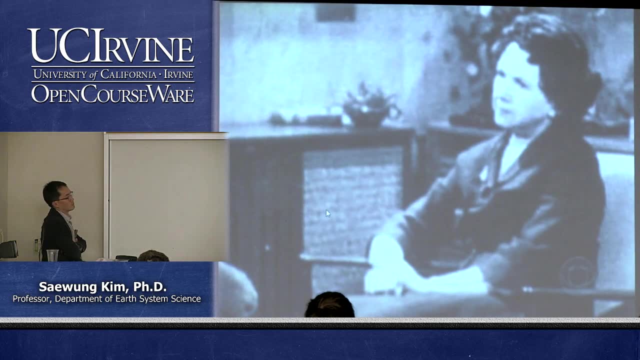 While Carson didn't contend that chemical insecticides must never be used, she faced harsh opposition. Those who were her critics. how did you see them in that documentary? Well, the chief critic was, as they say, he would have made a great 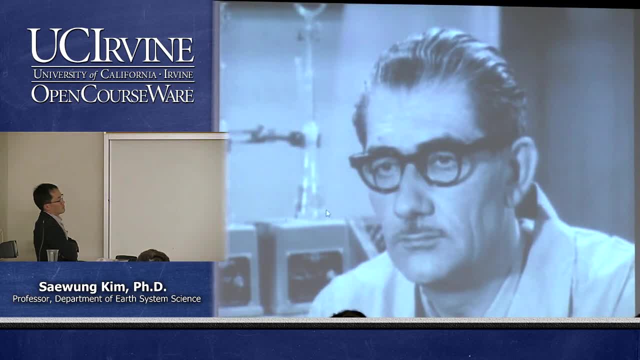 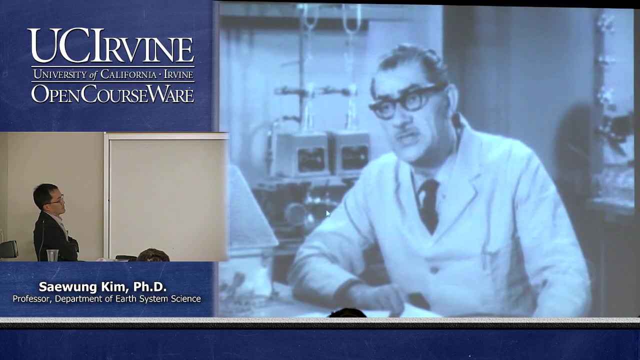 a great villain in a Bela Lugosi movie. Indeed, he would have A spokesman for the chemical industry, Dr Robert White-Stevens. The major claims in Ms Rachel Carson's book Silent Spring are gross distortions of the actual facts. 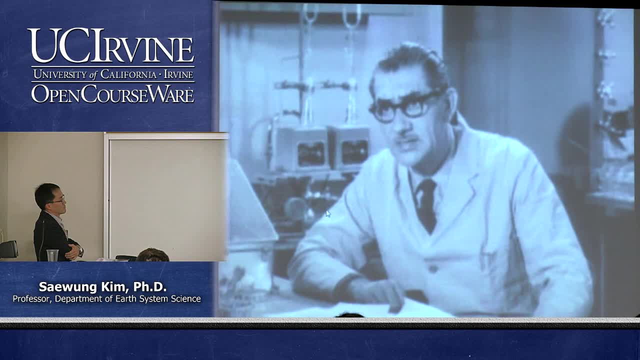 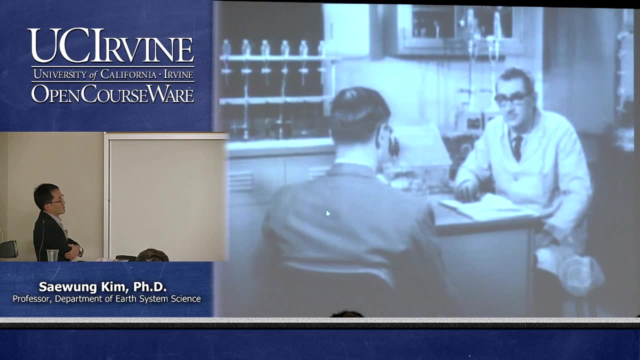 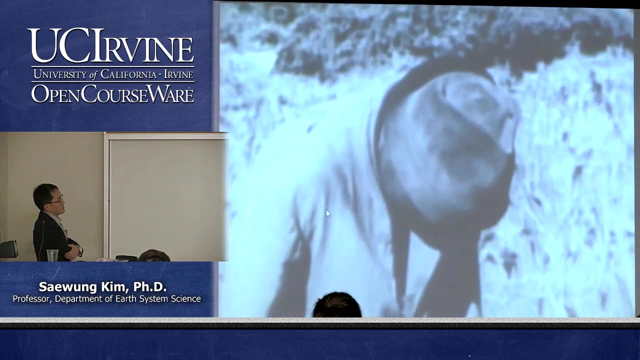 completely unsupported by scientific experimental evidence and general practical experience in the field. He was way over the top. He was: uh, If Ms Carson has her way, hundreds of thousands of people would be starving in the streets tomorrow If men were to faithfully follow the teachings of Ms Carson. 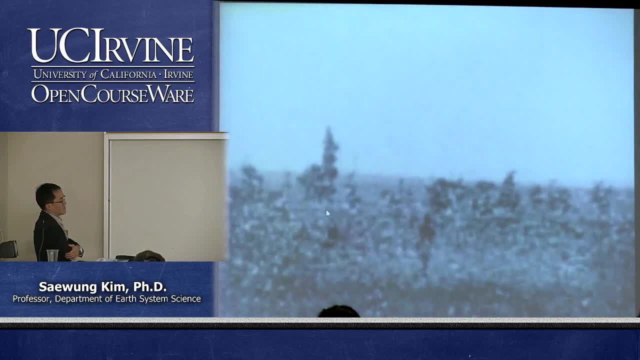 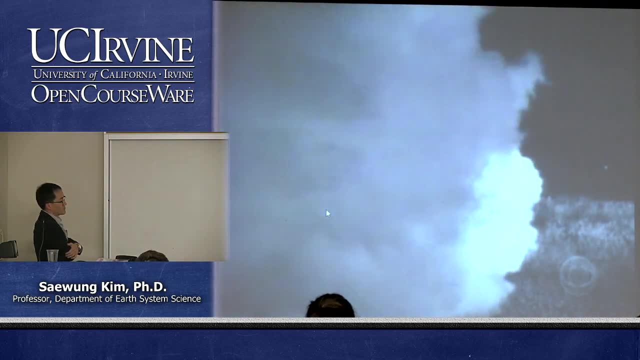 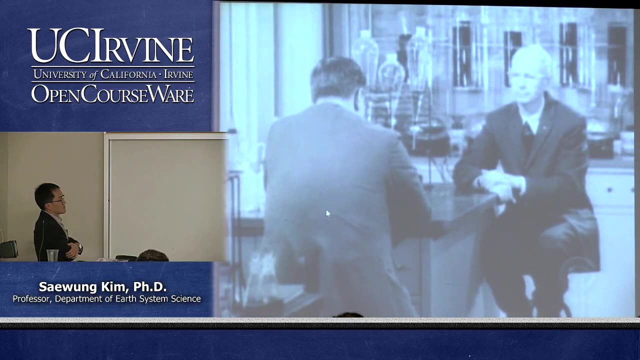 we would return to the Dark Ages and the insects and diseases and vermin would once again inherit the earth. And when CBS turned to government experts, the questions were many but the answers few. Dr Paige Nicholson, water pollution expert, public health service. Do you know how long the pesticides persist in the water once they get into it? Not entirely. Do you know the extent to which our groundwater may be contaminated right now by pesticides? We don't know that either. nor do we know if concentration may be occurring in groundwater. 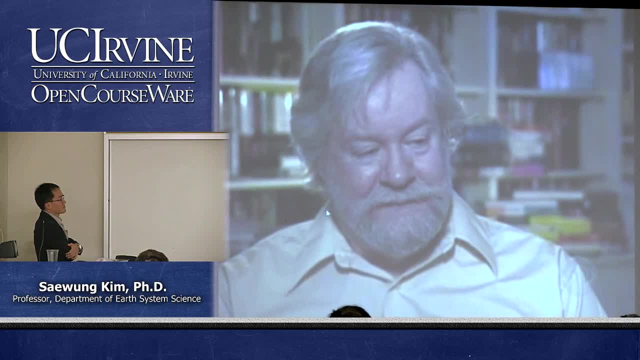 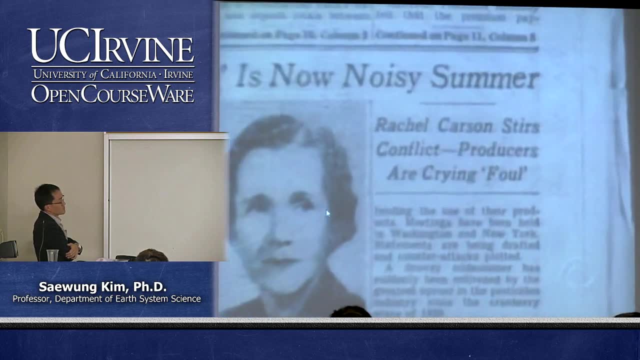 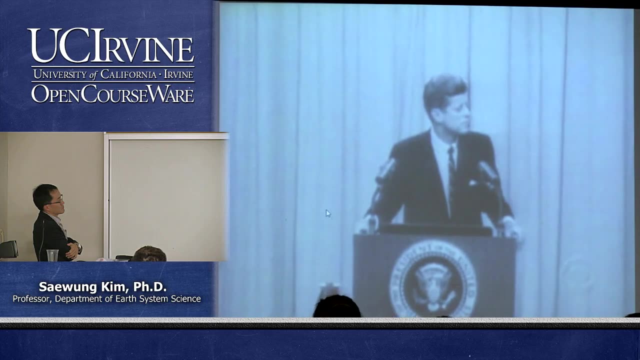 Did you have a sense of the impact she had made with Silent Spring? Oh, yes, Absolutely. John Kennedy mentioned the book in a press conference, so Clearly it was having an impact. There appears to be growing concern among scientists as to the possibility of dangerous long-range side effects. 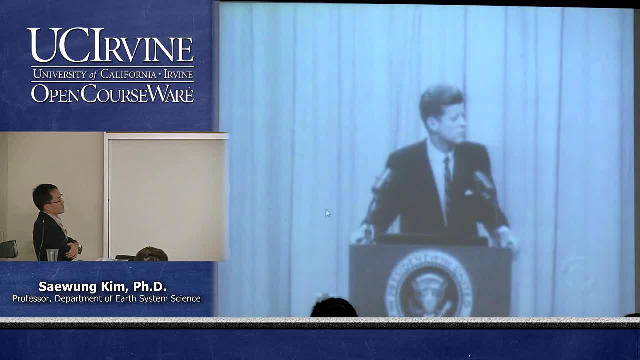 from the widespread use of DDT and other pesticides. Have you considered asking the Department of Agriculture or the public health service to take a closer look at this? Yes, and I know that they already are. I think particularly, of course, Ms Carson's book, but they are. 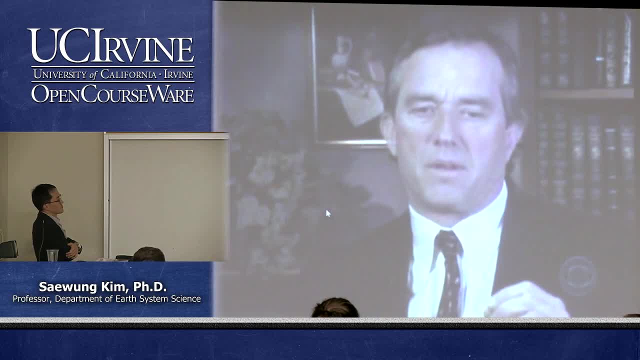 My uncle, Jack John F Kennedy um, read her book and said: I'm appointing an independent commission to investigate whether it's true or not. And that commission met for almost a year and then came out and said that essentially everything in Rachel Carson's book was true. Rachel Carson died in 1964, just 18 months after Silent Spring was published. She would never know that her crusade against pesticides forever changed the way Americans view their environment. DDT was banned in this country in 1972.. Carson's work also led to the creation of the Environmental Protection Agency. 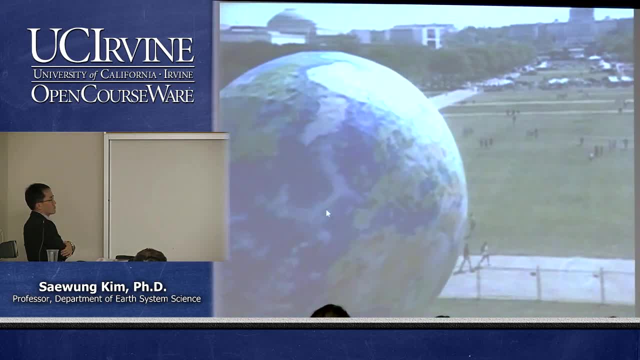 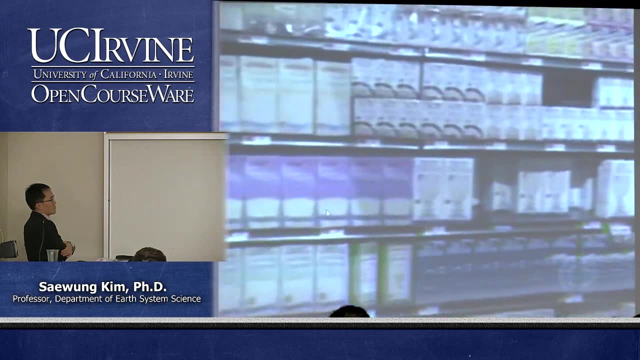 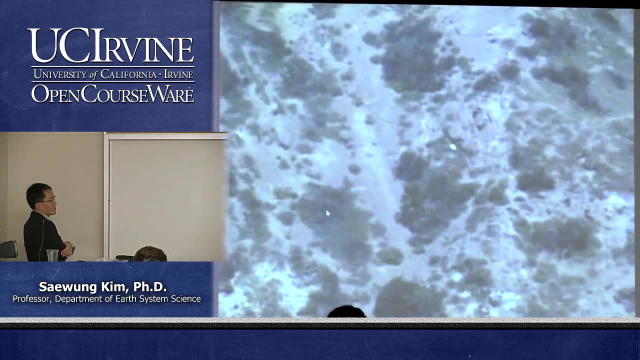 and without her pioneering efforts we might not be marking Earth Day. Silent Spring foreshadowed a debate over global warming, clean energy and organic food, But to best understand Rachel Carson's legacy, there's no better place to look than Catalina Island. 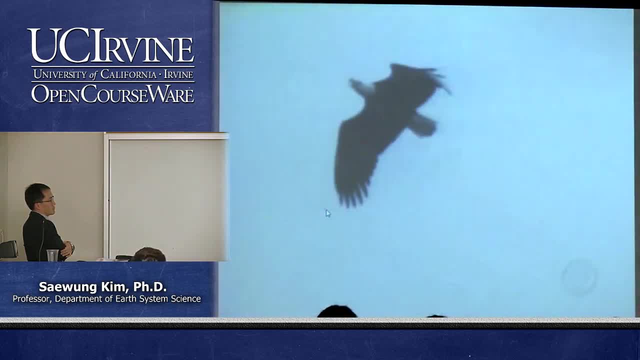 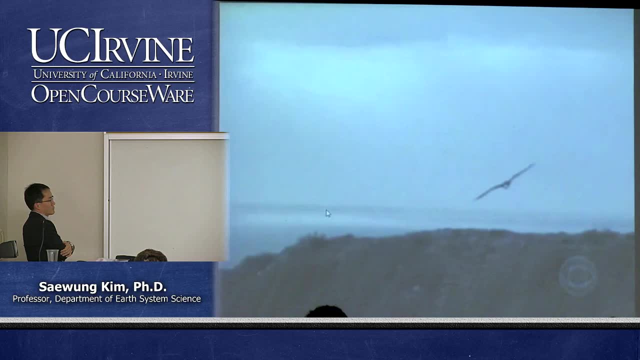 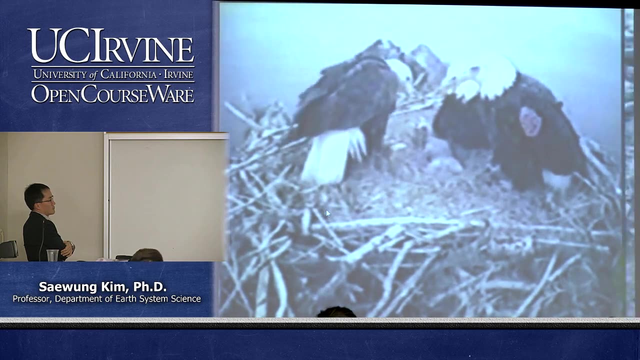 just off the coast of Southern California, home again to the bald eagle. It's really an exciting event for us. The eagles had all but disappeared after DDT was dumped into local waters, leading to eggshells, so thin chicks couldn't survive. 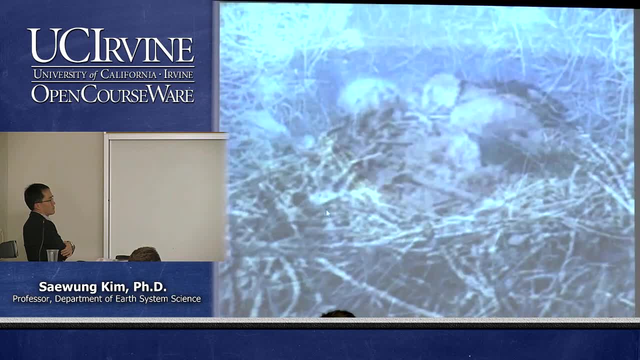 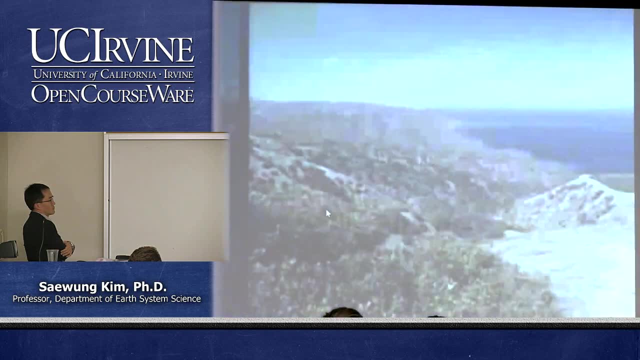 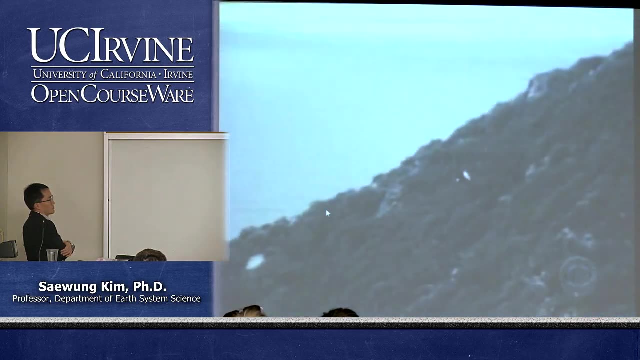 But just this month, for the first time in decades, eggs left in nests in the wild hatched on their own. Those white, fuzzy spots are the new eaglets. Ann Musket, president of the Catalina Island Conservancy, believes the eagles owe it all to Rachel Carson. 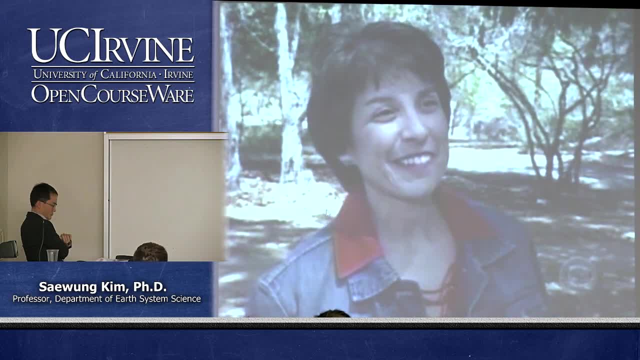 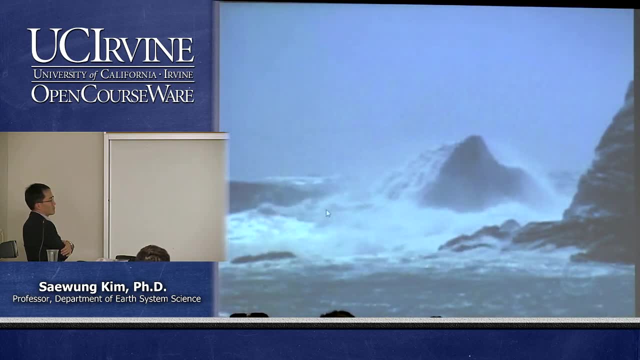 So I think that wherever she is right now, she must be looking down on Catalina and thinking: this is really a wonderful occasion. Rachel Carson's quiet yet insistent voice can still be heard today. I truly believe that we in this generation 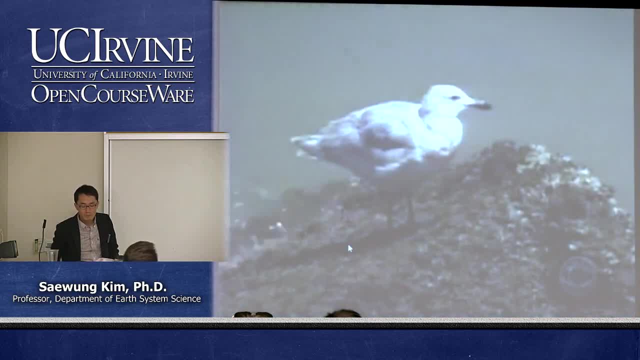 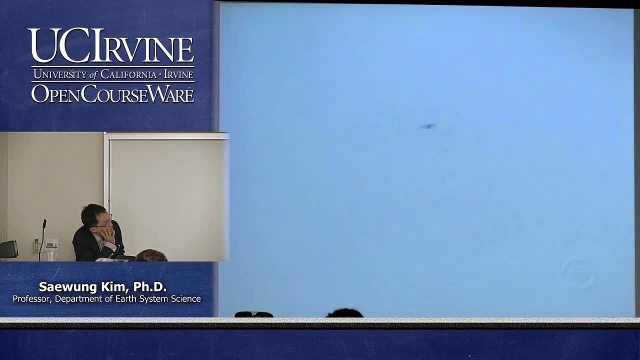 I truly believe that we in this generation, I truly believe that we in this generation, must come to terms with nature, And I think we're challenged, as mankind has never been challenged before, to prove our maturity and our mastery not of nature but of ourselves. 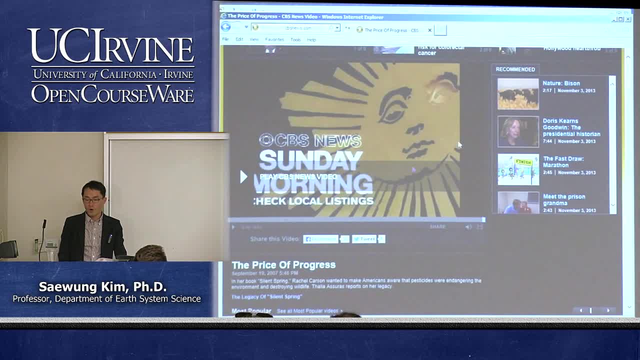 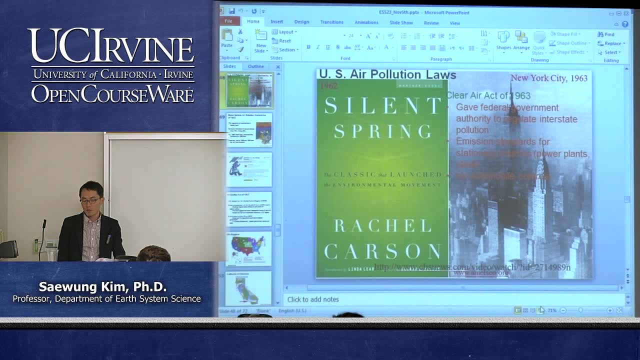 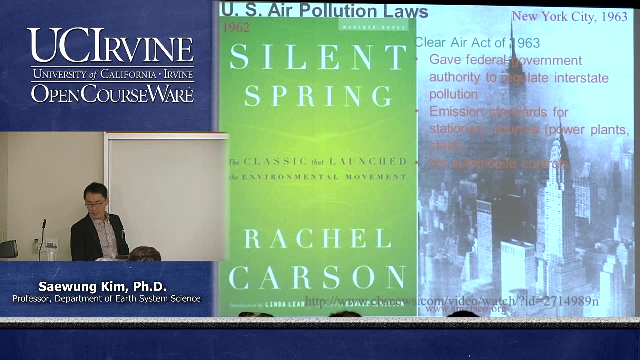 So EPA was initiated not from this Los Angeles smog problem, rather this Rachel Carson's contribution towards environmental awareness, and through the DDT And then EPA regulation got kicked in, So a lot of improvement has happened in terms of other parts of the environment. 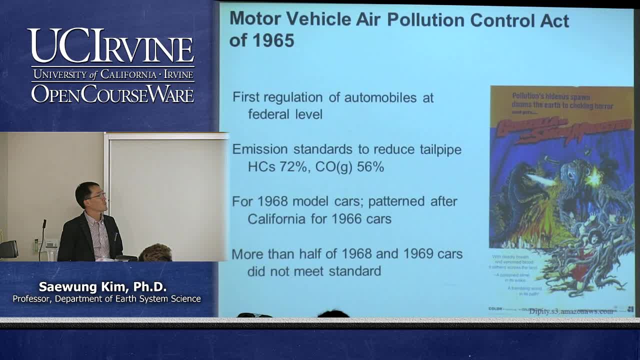 in terms of air pollution too. So even in 1965, before that EPA regulation kicking in, so air pollution in this country was so bad. there was a very- it seemed like a very- mediocre movie called Godzilla vs Smug Monster. 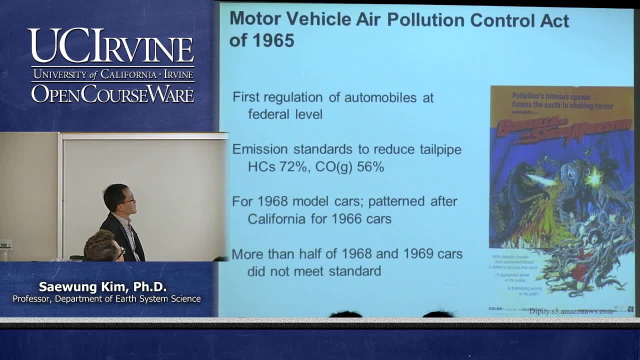 It was actually a movie called Godzilla vs Smug Monster. It was actually a movie called Godzilla vs Smug Monster And it was actually really out there. So I was a little bit. that thing is really out there, Actually, that's true.